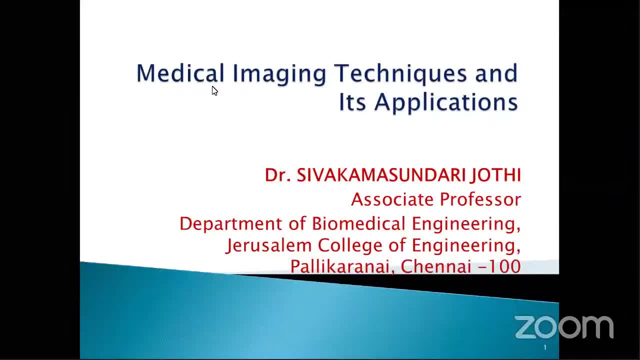 Okay, A very good evening to one and all present. On behalf of Department of Biomedical Engineering, I welcome you to the Institute of Technology, I welcome you to the Institute of Biomedical Engineering Techniques and its Biomedical Applications. So, in this regard, I would 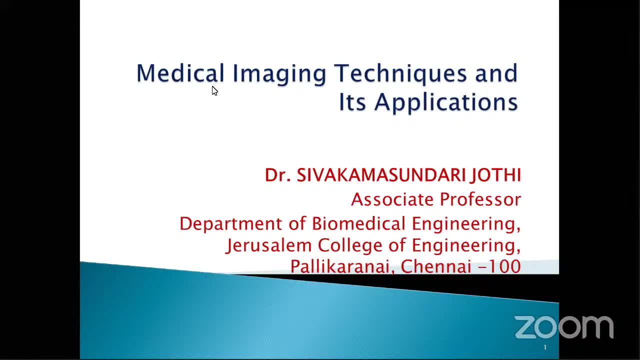 like to request Ms Santoshini Arulvallal to give a brief introduction about today's session. speaker: Dr J Sivakama Sundari: ma'am, Yes, ma'am, Yes, ma'am So speaking. 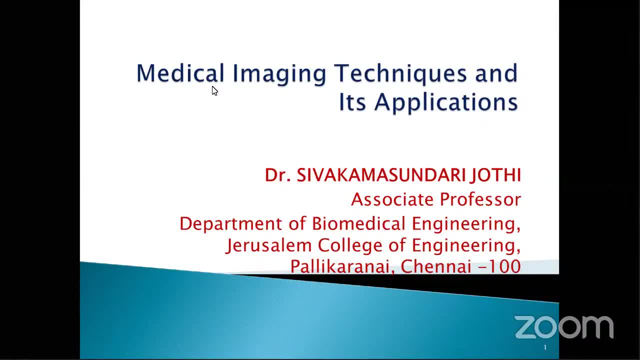 of her education. she had completed her PhD in Biomedical Image Processing and Data Mining in Madras Institute of Technology, Anna University, Chennai, and she holds Bachelor of Engineering in Applied Electronics in Hindustan College of Engineering, Madras University and Dr. 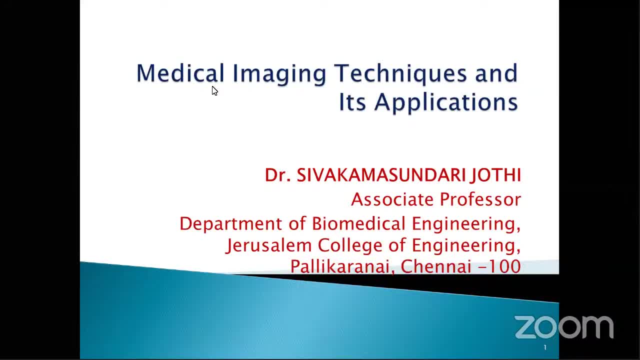 Sivakama Sundari holds her Bachelor of Engineering in Electronics and Communication Engineering in Periyar Maniamai College of Engineering and Technology for Women. Speaking of her teaching, she worked as lecturer in Hindustan College of Engineering, Padur, Chennai, and worked as Assistant Professor in Sri Andal. 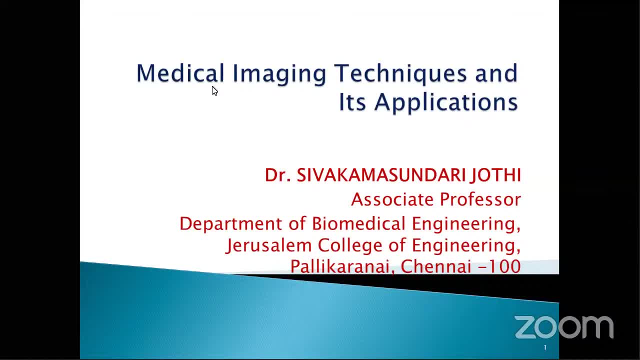 Alagar College of Engineering and in Assen Memorial College of Engineering and Technology, Chengalpur. Now she's currently working as Associate Professor in Jerusalem College of Engineering As a whole. she holds a teaching experience of engineering and technology for women. She is a professor of engineering and technology. 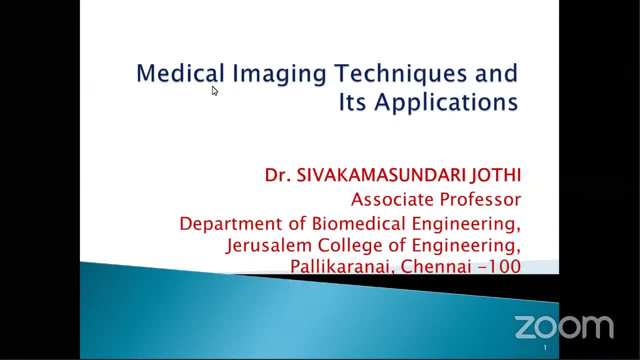 of 12.8 years. Speaking of her research experience, she worked as a project associate in CISCSR, Indian Institute of Technology, Madras, and worked as research associate one in NHHID Anna University, And her current research focuses on development of content-based image. 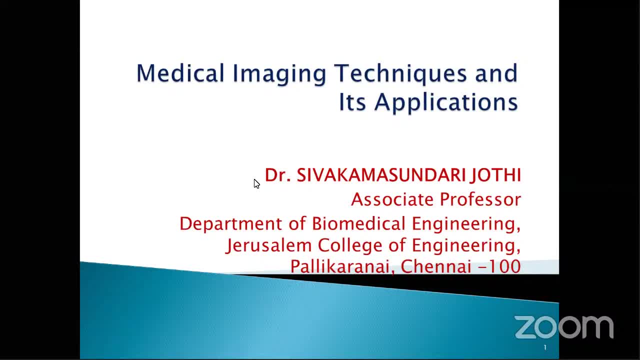 retrieval schemes for screening of diabetic retinopathy and glaucoma, segmentation of images using optimization-based thresholding techniques, analyzing of various textural and structural image features, classification of medical images and Arduino-based signal processing. She has published a number of articles in journals such as Journal of American. 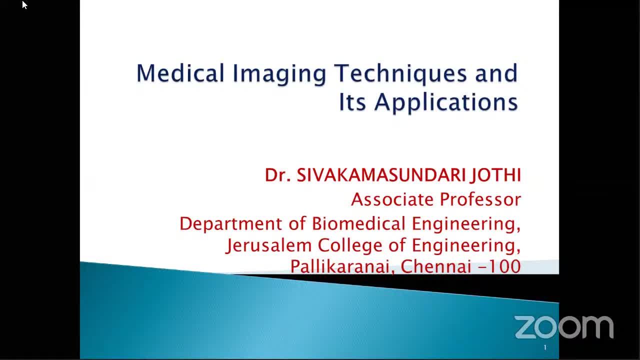 Biomedical Sciences, Instrumentation and Journal of Medical Imaging and Health Informatics and International Journal of Image Mining. And regarding her research experience, she has won the Best Paper Award in International Conference on Communication and Security, Pondicherry College of Engineering, India, and have won the Best Paper Award in National 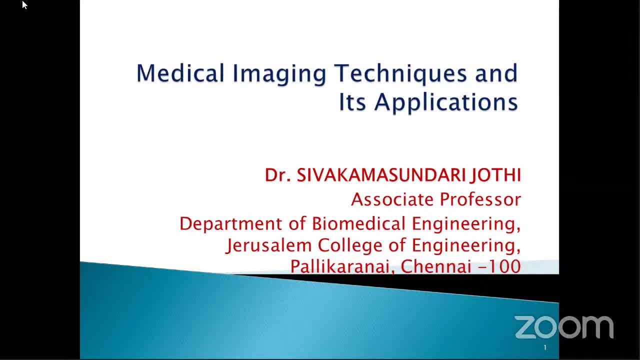 Conference on Computing and Communication in Anna University, Trinalveri Region, India. She has achieved Madras University 8th Rank in 2002 in ME degree exams, So we are very much honored to have you as our today's speaker, ma'am. 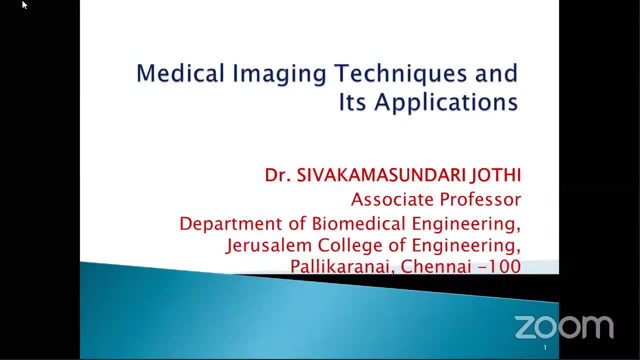 Thank you, ma'am, for our guest lecture, And now I kindly request Dr J Shivakant Sundari, ma'am, to please take over the session. Thank you, ma'am. Thank you for a nice introduction on me, Ma'am. shall we go for next slide, ma'am? 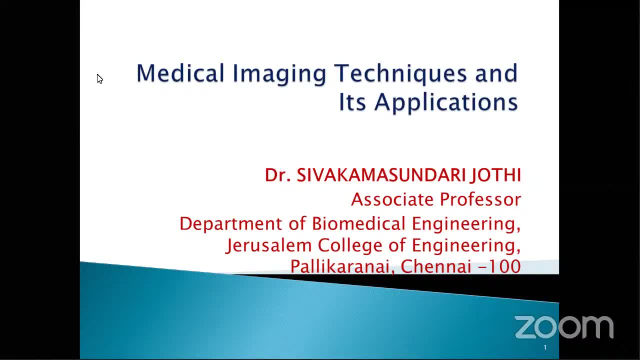 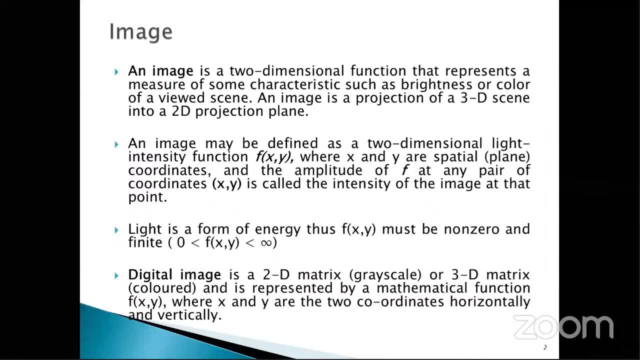 Yes, ma'am. Good evening to our staff members and students. I am Dr J Shivakant Sundari. I am the Director of the International Conference on Communication and Security, Pondicherry College of Engineering. I am the Director of the International Conference on Communication and Security, Pondicherry College. 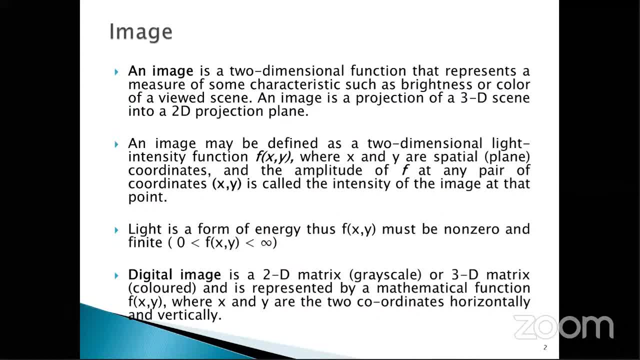 of Engineering. I am going to take medical imaging and its application. Don't panic, Just I am going to try to touch some important topics in medical imaging and image processing. Image, An image, is a two-dimensional function that represents a measure of some characteristic. 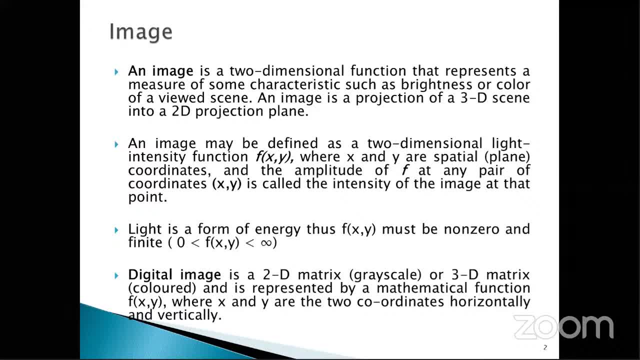 such as brightness or color of a viewed scene, And image is a projection of a two-dimensional image. Okay, So image is a two-dimensional light projection of a 3D scene into a 2D projection plane. So it is a two dimensional light intensity function f of xy, where x and y are spatial. 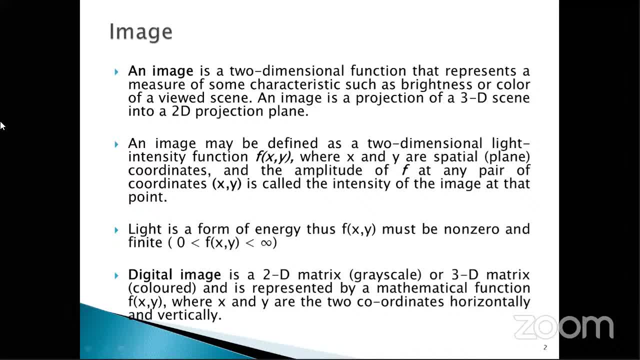 plane coordinates And the amplitude of f at any pair of coordinates. xy is called the intensity of the image. at that point, Light is a form of energy. thus f of xy must be non-zero and finite. Okay, So f of x comma y is greater than 0 and less than infinity. Digital image is a 2D matrix. 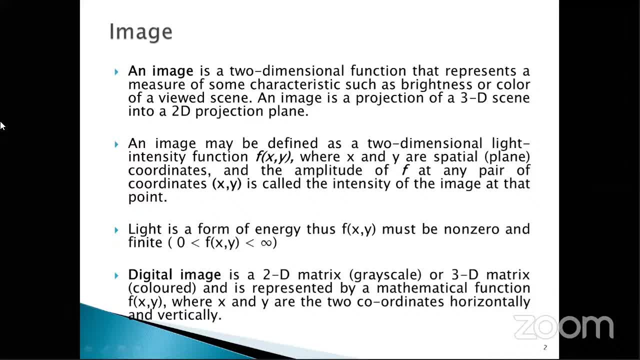 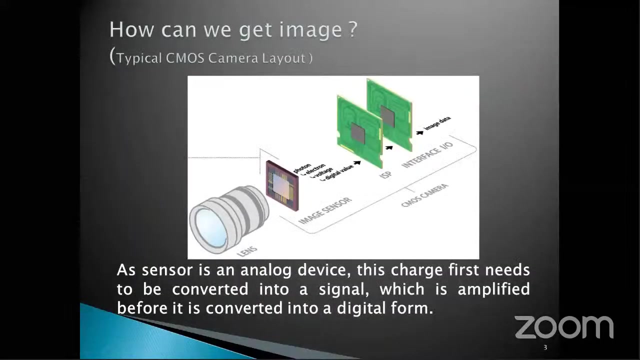 grayscale or 3D matrix color. It is represented by a mathematical function f of x, comma y, where x and y are the coordinates, horizontally and vertically. Next slide now. Next slide now, Excuse me. Next slide now. Okay, How can we get image? For example: 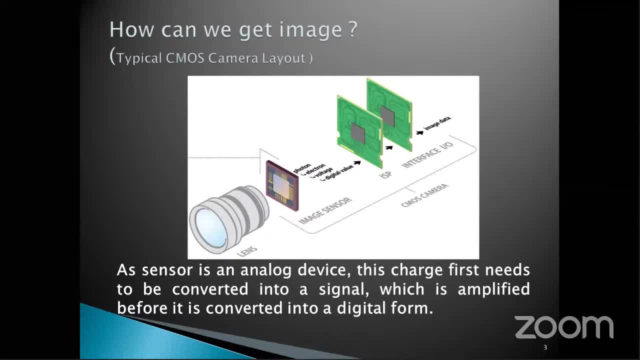 if you have a camera, So this is camera, It is an advanced camera. So here, lens is there. After the lens, image sensor will be there. It is a CMOS sensor. Okay, So after that, image and signal processor: This is a processor. Okay, Image and signal processor and interfacing. 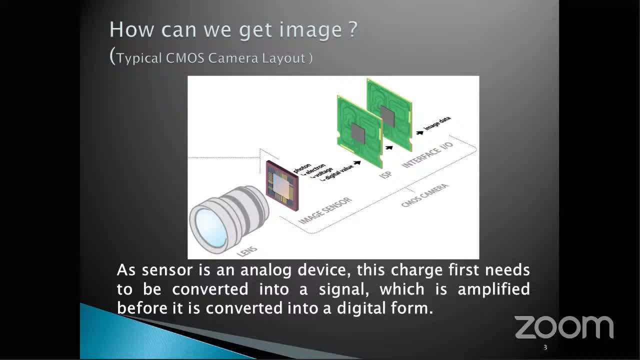 IO. So from this what we have to interface with this camera? Okay, So this is the some block diagram like block diagram, lens, image sensor, image and sensor- sorry, image and signal processor interface IO. Okay, So a sensor. 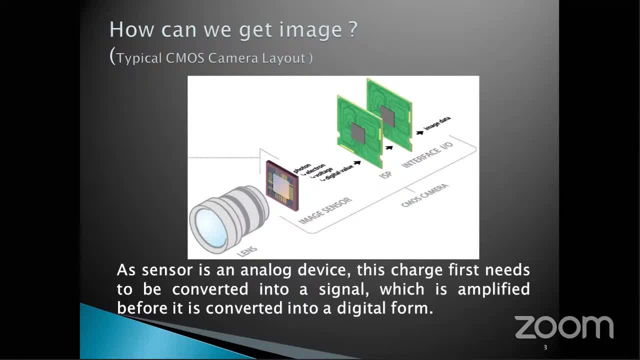 is an analog device. It will sense the image. Okay, When light is focused on that image or any object, Okay, Light is focused on the object. The amplified signal will be converted into digital form. Okay, Next slide. Next slide now. 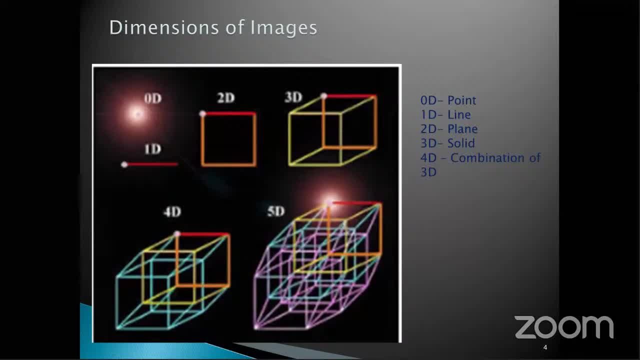 So, dimensions of image, You know 0 dimension, 1 dimension, 2 dimension, 3 dimension, Okay, So many dimensions you know. So what is 0 dimension? It is a point, Okay, It is a point. It can be the. 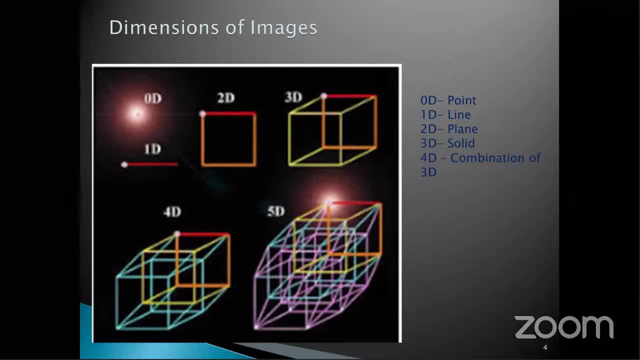 0 dimension. Okay, So line some line from point. we are drawing some line in a paper. It is 1D. It is a line From the point where drawing a line. So it is called 1D. 2D means some shapes. Okay, It is a plane. Okay, It is a shape. 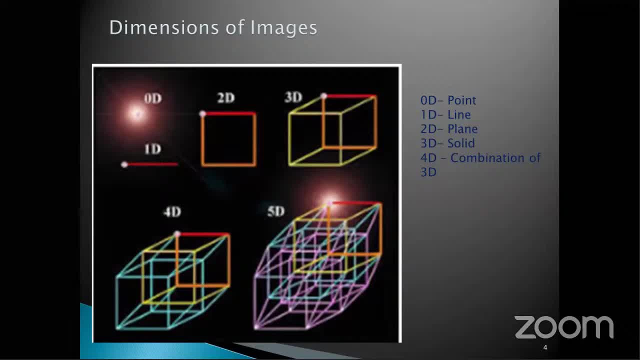 So 2D, This is the square, And 3D means it is a solid. Okay, It is a cube, It is a solid. We can imagine in 3D form: It is a cube. 4D means combination of 3D. Okay, Combination of 3D. 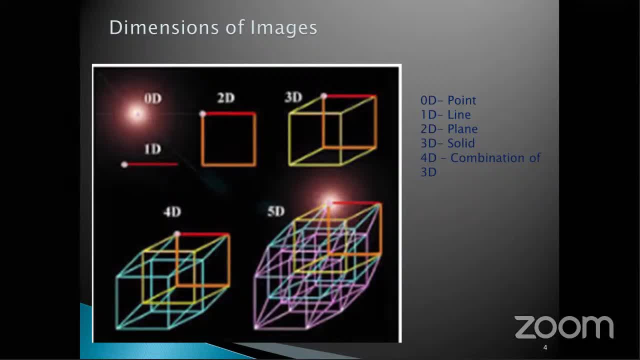 See here: this is 4D. Many shapes are there, Lines point: everything is there. 0D, 1D, 2D, 3D, everything is there. That is 4D. Okay, This is 5D. Next slide: ma'am. 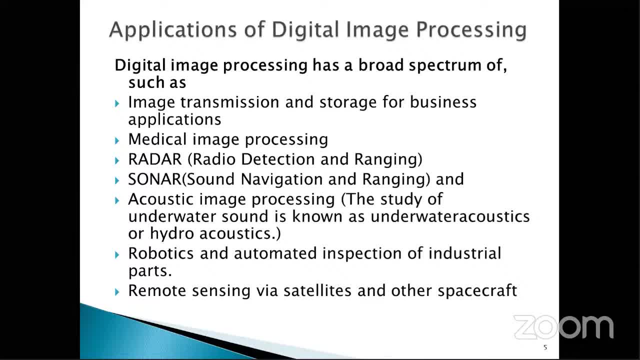 Applications of digital image processing. Okay, So digital image means using some sensor, We are capturing image and it will be converted into digital form. Okay, So what is the application, Why we are going for digital image? What is the application of digital image processing? 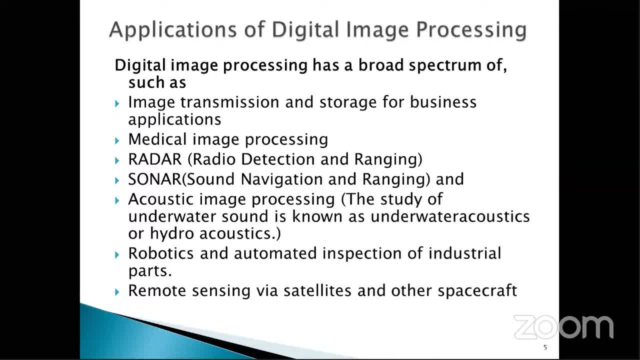 See here. digital image processing has a broad, broad spectrum of classification, such as image transmission and storage for business application. So we are, the application will be broadly classified, Okay, In image transmission and storage for business application. So we are taking many images. If you are having cell phone, 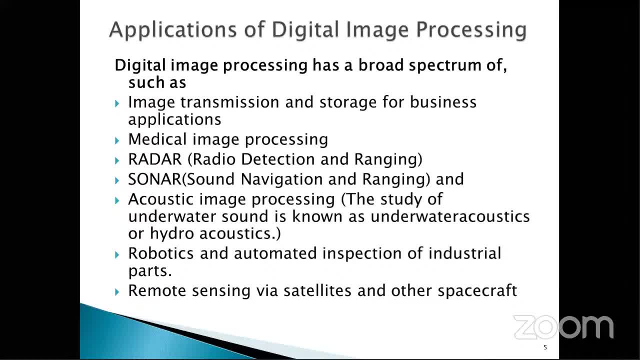 you are taking many images You have to store in your file. Okay, In your folder you are storing. So if you are storing more than 400 or four, 500, it will the the storage. the area will be over. Okay, So we have to transfer the already saved image into some other. 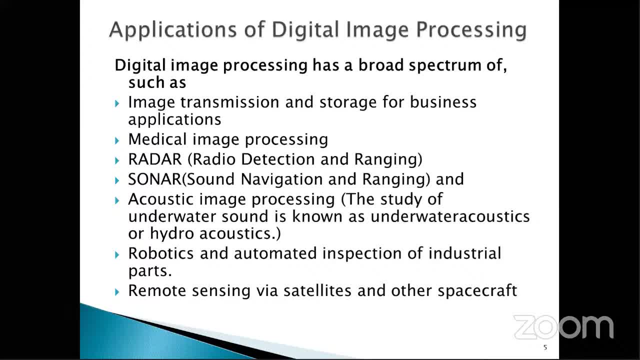 storage devices. Okay, So for further applications: medical image processing: this application, digital images, are used in medical image processing and radar, radio detection and ranging sonars, sound and navigation and ranging. So radars are now in airports. we are having so many radars. 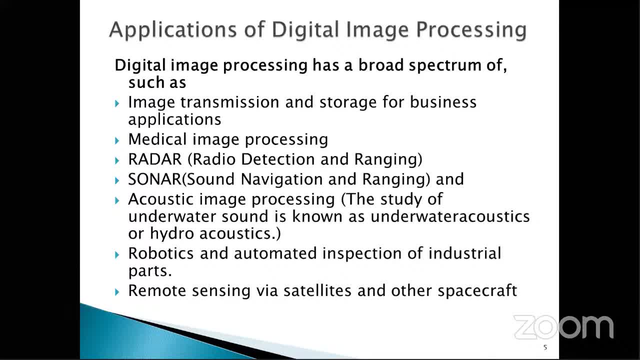 under it, tracking the flights. Sonars: it will be used in ship in sea. Okay, Acoustic image processing: The study of underwater sound is known as underwater acoustics or hydroacoustics. So we are having a ac- acoustic image processing. Okay, Robotics and automated inspection of 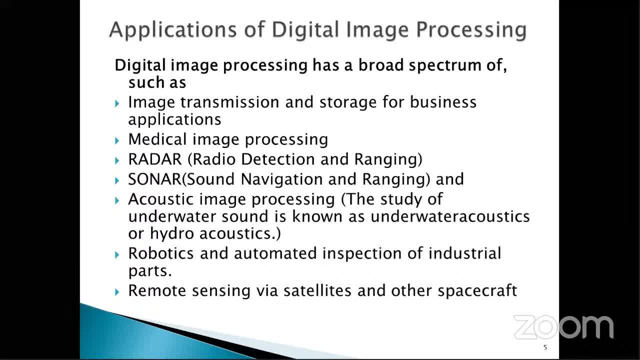 industrial parts. So robots, or if any people are not going to some places in that area, are robots that will be placed. it will attract human or some other extraterrestrial objects and some other objects. okay then, automated inspection of industrial parts: okay, in industry. 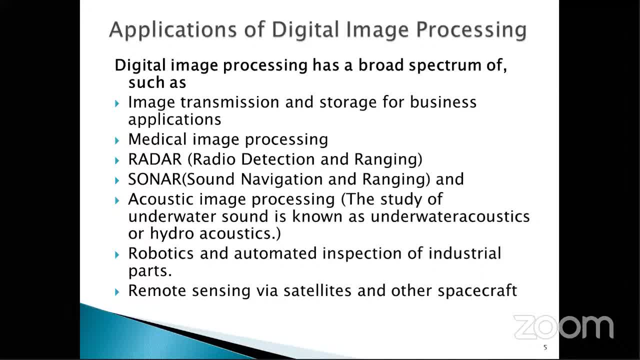 everywhere automation takes place. so in automation um, this camera will be fixed. okay, in our area, also in our house or some um a college. okay, industry cctv camera, road okay, especially in roads. cct camera will be there so it will take picture whenever we want. 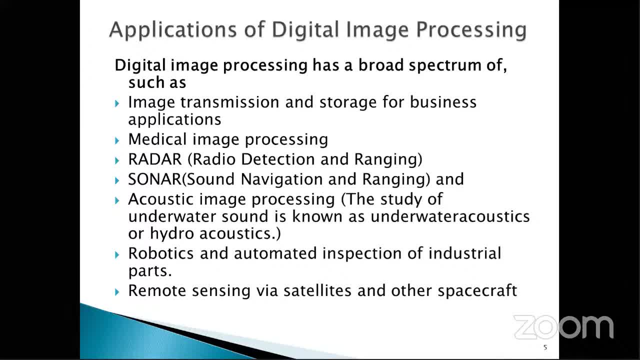 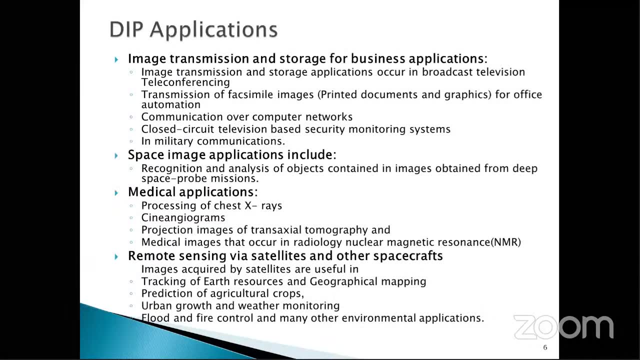 images. we can, um, we can see the images, okay. and remote sensing via satellites and other spacecraft. remote sensing is very, very, very important. uh, image processing application. next slide, ma'am applications- okay. image transmission and storage for business application. in that many applications are there. image transmission and storage applications occur in broadcast television. 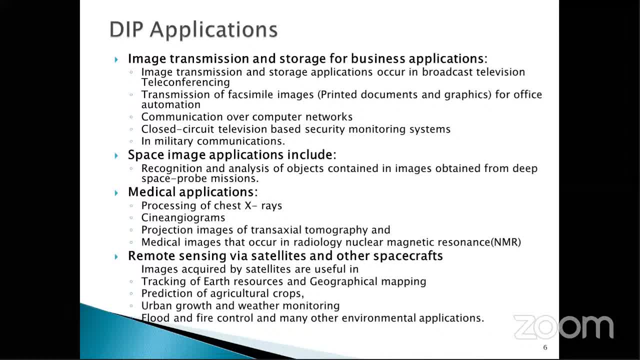 teleconferencing. transmission of facimile images, printed documents and graphics for office automation. communication over computer networks close to subtle television based security monitoring systems in military communication space. in image applications include: recognition and analysis of objects contained contained in images obtained from deep space, probe machines, medical applications, processing of chest x-rays. 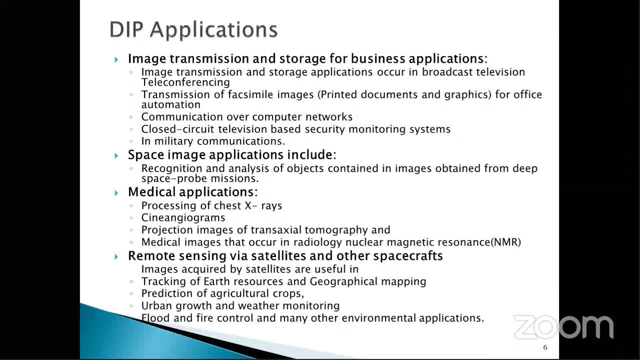 angiograms and the projection images of transaxial tomography, medical images that occur in radiology, nuclear magnetic resonance, nmar. so in this field, also in medical application also, digital processing is used, remote sensing via satellites and other spacecrafts. image acquired by satellites are useful in tracking of earth resources, geographical mapping, prediction of agricultural 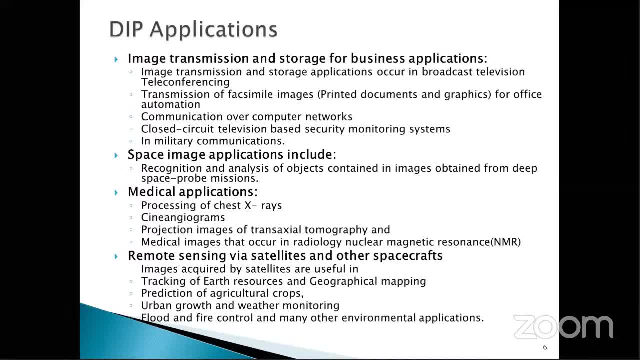 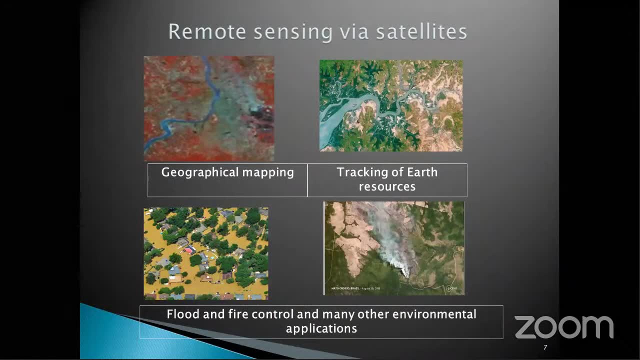 crops, urban growth and weather monitoring, flood and fire control and many other environmental applications. next slide see here some images are given: remote sensing via satellites. here geographical mapping. so in this mapping river and mountain areas will be identified. okay, any extra uh objects are there and uh tracking of the earth resources? okay, 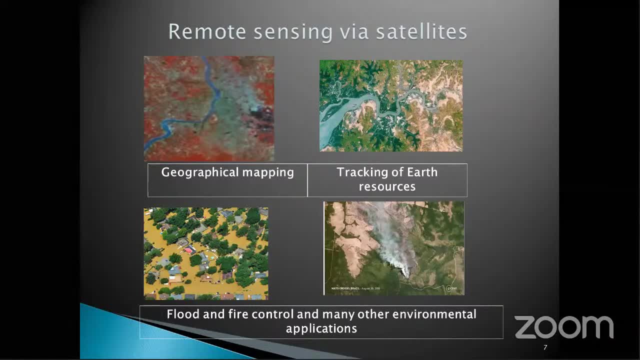 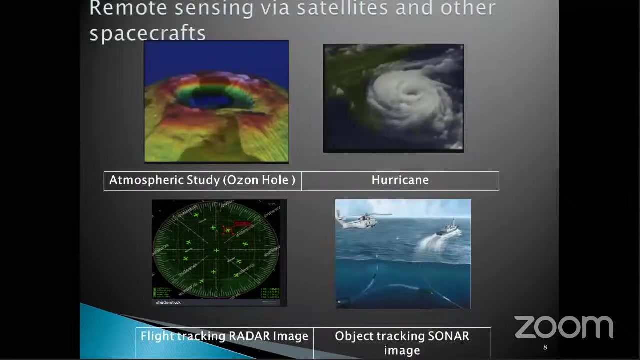 where uh flood is occurring, or fire fire control. okay, see here this is forest fire and here flood. okay, surrounded in a village. so this can be seen through this image processing. okay, there also image processing is used. next slide here: remote sensing via satellites and other spacecraft. see here, this is. 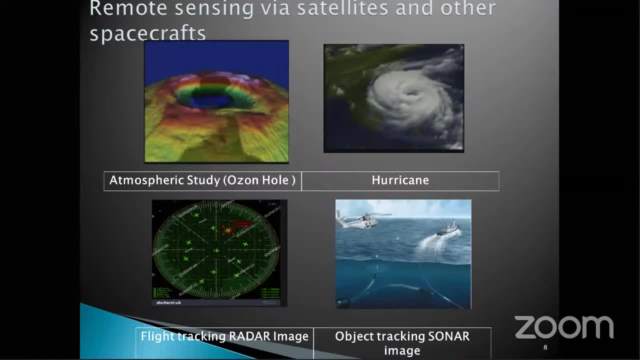 atmospheric study ozone hole is viewed okay, so we can measure the ozone hole, we can monitor how the ozone hole is expanding and depleting like that. then hurricane, the way of hurricane, we can see, and here this is uh, radar, okay, finding our tracking the airplanes- okay, from the airport. and here it's a ocean under ocean, uh, some. 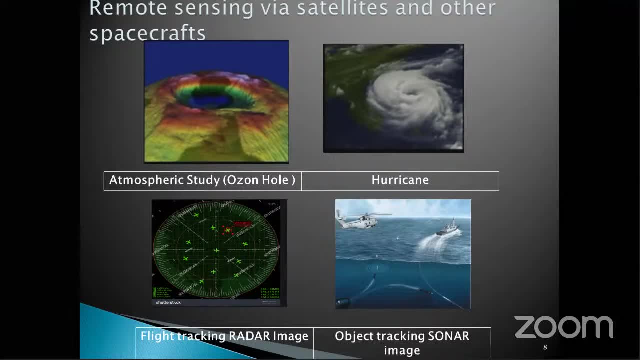 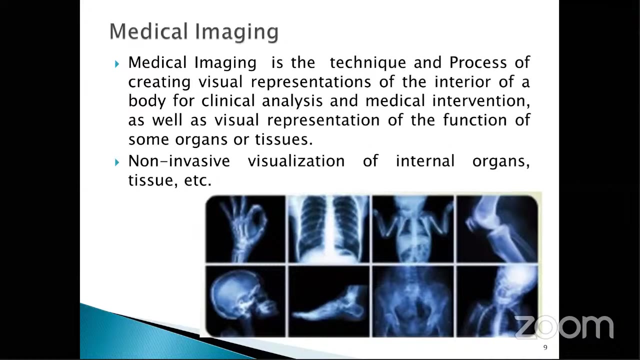 submarines, seabirds, icebergs and some other objects present inside the sea will be monitored. next slide: medical imaging. so image processing. we know we are using image processing in medical imaging also here. these are all x-ray images. okay, x-ray images. medical imaging is the technique and the process. 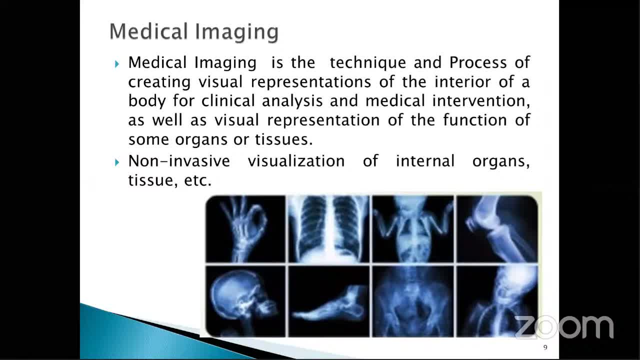 of creating visual representations of the interior of the environment and the environment and the interior of a body for a clinical analysis and a medical intervention, as well as visual representation of the function of some organs or tissues. you know why we are taking x-rays: if any broken legs or something chest x-rays, it will show flum or any deformation in 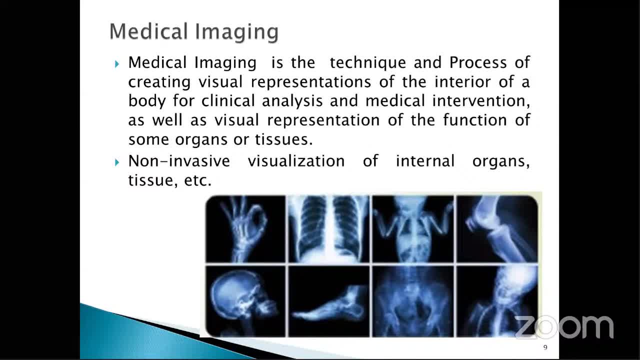 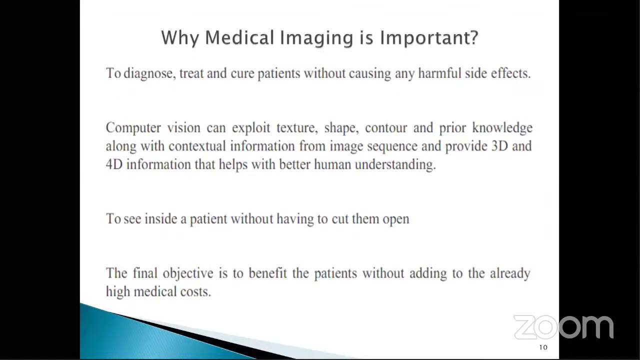 abnormalities in lungs we can find. okay, so it is a non-invasive imaging means it is a non-invasive visualization of internal organs and tissues. okay, without any cutting or opening of the tissues we can easily visualize the internal organs of the tissue. next slide now why the medical imaging is important: to diagnose, treat and cure patients without causing any harmful. 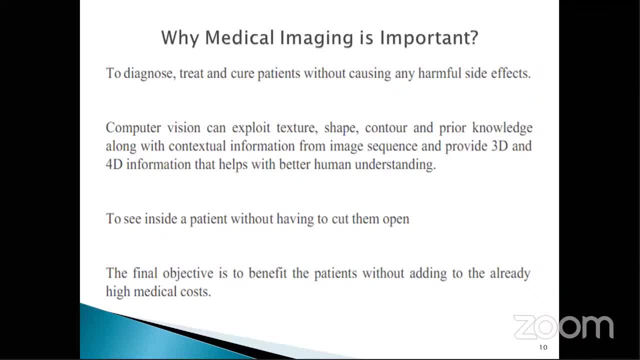 side effects. okay, without causing any harmful side effects. computer vision can explore the causing any harmful side effects. computer vision can explore the other side effects. computer vision can explore the other side effects. all kinds of are time-serving to determine. can Sanae perform from the physical lens. so the challenges arising from the physical image can be- Dumsek 기능, someday made un clearly to see exactly the sides of a child's body, coffee and Ted McClellan to see the Himalayan Sue Vextreme information from some parleran as well, and provide a better human understanding. so while we are seeing the image we can store and we can use. Canan, eosa andou angele are also to see inside a patient without having to cut them open. the final objective is to benefit the patients without adding to the already high medical costs. describing the subject, as mentioned earlier, cannot be found處rred. 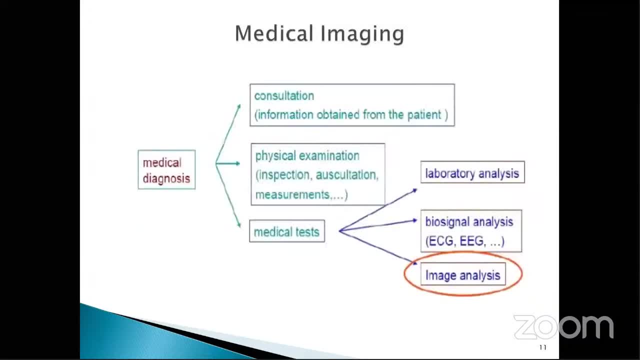 Next slide In medical imaging. see here medical diagnosis. medical imaging is used for medical diagnosis, consultation, information obtained from the patient. So we are taking some images and going to doctors, they will consultants, they will see the x-rays or some other ultrasound images, CT images. 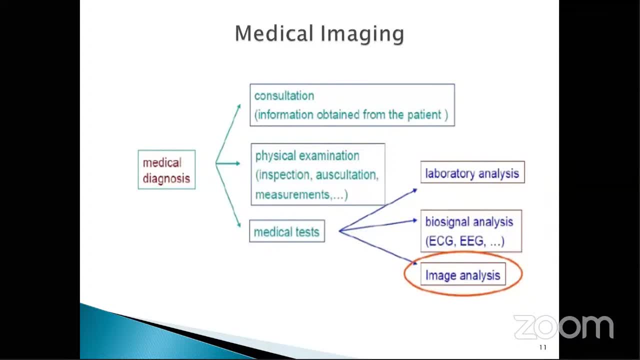 They will find what are the abnormalities present in that image And physical examination, inspection and auscultation and measurements. Then suppose in a image some lumps are there. okay, benign or malignant, some lumps will be there. They will find the size of the lumps. okay, doctors. 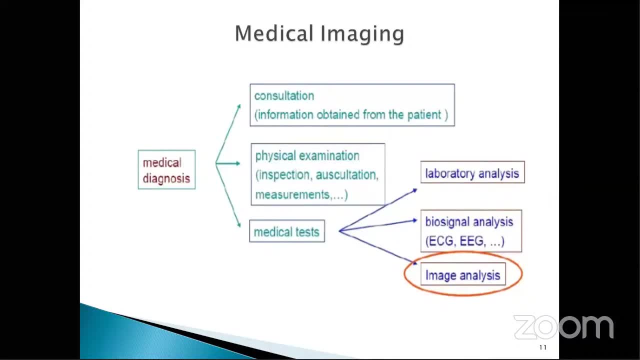 And they will prescribe medical tests. further tests: Okay, biopsy, if biopsy is needed, they will describe that. Okay, the laboratory analysis: they will instruct us to go for laboratory analysis: biosignal analysis, ECG, EEG and image analysis. Okay, doctors will describe for us to take image analysis also. Next slide: 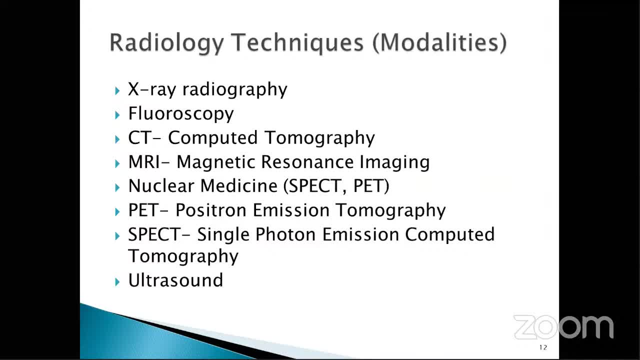 So what are the modalities? Okay, modalities, imaging, modalities available in medical imaging means x-ray, radiography, fluoroscopy, angiogram and all called as fluoroscopy. They will inject some dye to our body and they will take x-ray. okay, or CT scan. 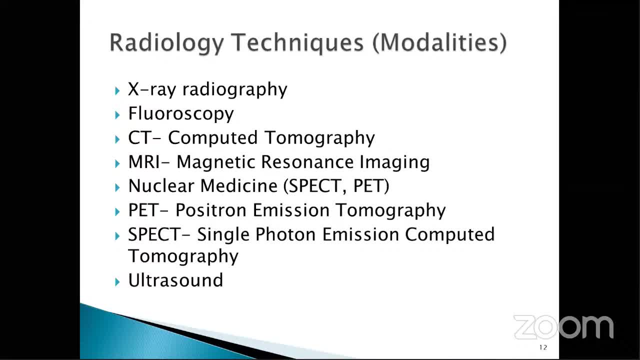 And it will be. the abnormalities will be easily seen through fluoroscopy. Okay so, x-ray radiography, fluoroscopy, CT, computed tomography, MRI, magnetic resonance imaging, nuclear medicine, SPECT and PET. PET means positron emission tomography, SPECT means single photon emission computed tomography, and ultrasounds. Okay, next slide, please. 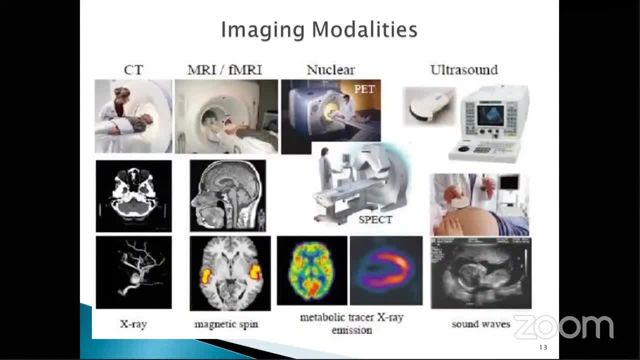 See here, this is the imaging modality for CT And this is MRI. The output of the CT is like this: Okay, it's a brain. Okay, Then here it's a MRI, It's a whole head inside the head, how the brain and the thalamus, hypothalamus, all will be seen here And it's combination, combination of MRI and SPECT. okay, or PET. 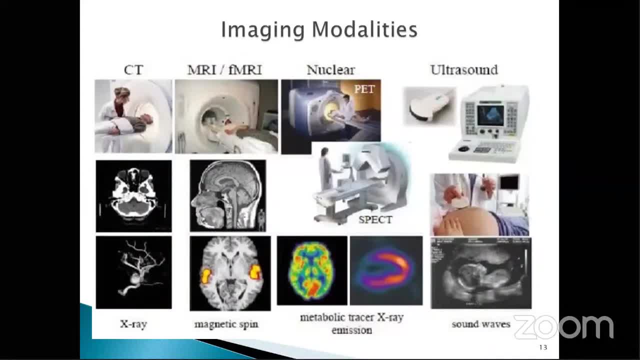 And this is PET positron emission tomography. This is SPECT. See, here, coloring will be there. Okay, so if there's a regions or red means it is having some abnormalities And blood is more present in that area and heat also more here, And this is SPECT. 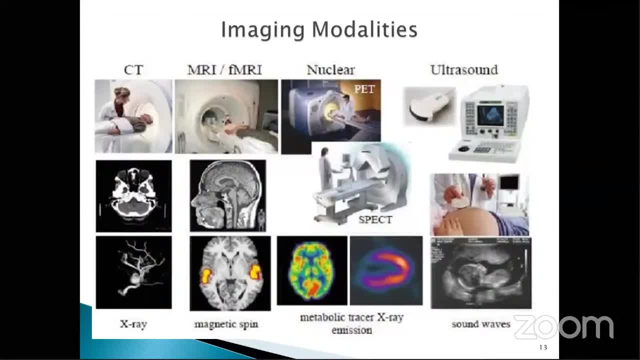 This is a sensor. Okay, here it's a sensor. Probe is there? And the output of the ultrasound image. Okay, next, This is the ultrasound image. Okay, next, Why we need image processing. Why we need image processing. 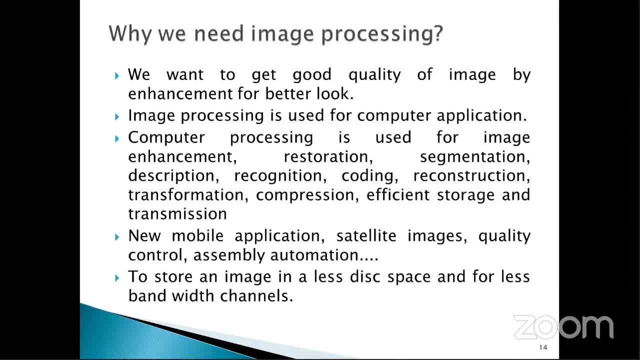 The output of the ultrasound image. Why we need image processing: want to get good quality of image by enhancing uh, but for better look. okay, you are taking many images in cell phone, for example. we are taking many images through cell phone. if it is daytime with the good sunlight, we can get clear image. if it is very dark, we cannot get good images. 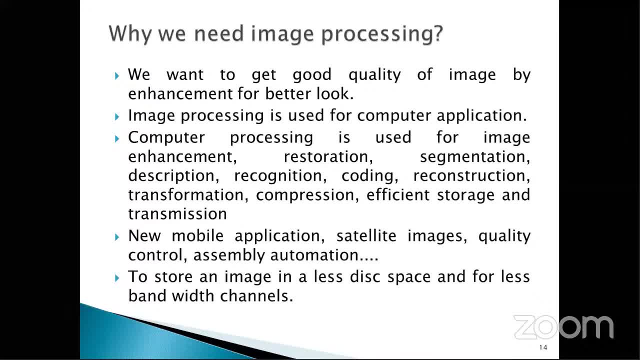 okay, so that in that place. okay, we need some enhancement techniques. okay, so we want to get good quality of image through enhancement. image processing is used for computer applications. okay, if you take some image and you stored in a storage device, we can easily come connect to the computer. 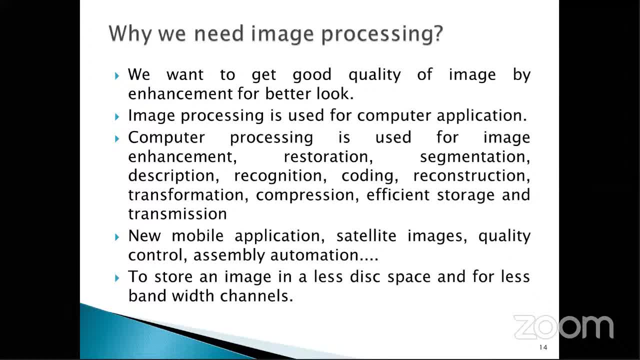 and whatever uh process we want, we can do that. okay. so enhancement, image restoration: okay, we can fuse the image, we can register the image. okay, so through computer we can do many process. okay, so computer processing is used for image enhancement, restoration, segmentation, description, recognition, coding, reconstruction, transformation, compression, efficient storage and transmission. 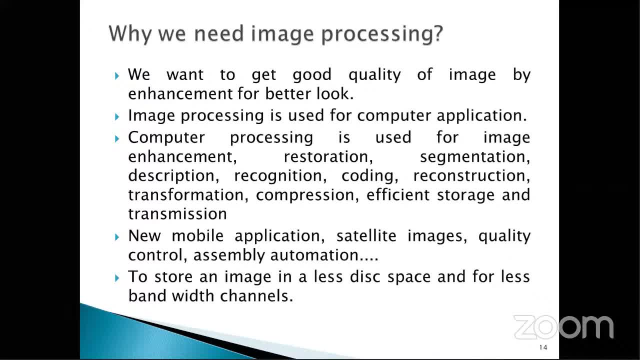 okay, so many things we can do with this computer processing. okay, so after time we can send more images to anybody. okay, through whatsapp, we are sending more images through emails. we are sending, uh, e-mails, in other words, to anybody else we can. you can go to our web page, sorry, or google, in very small numbers of the email we can. 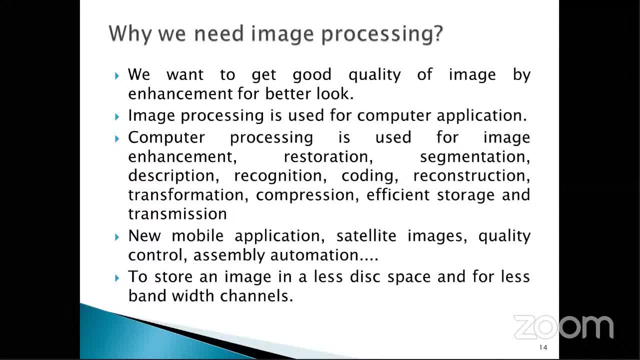 go through all these links that you can download or upload. and, uh, you need just to download all the souiono desks for description of the lab videos and also the web page to download, and so you can download most of theAt flexbeat. uh, all the layers. competitors, so glad that you guys watch this video. important also for capabilities. we have gotå constantly video conferences. okay for that, video conferencing. we need image compression also. okay so, image compression. it will reduce our data- okay, total data- and it will helpful for easy transmission. okay so, new mobile application, satellite images, quality controlled assembly automation. so in this area also, we are using image processing to store an image in a less disk space and for less bandwidth for non-computer services. 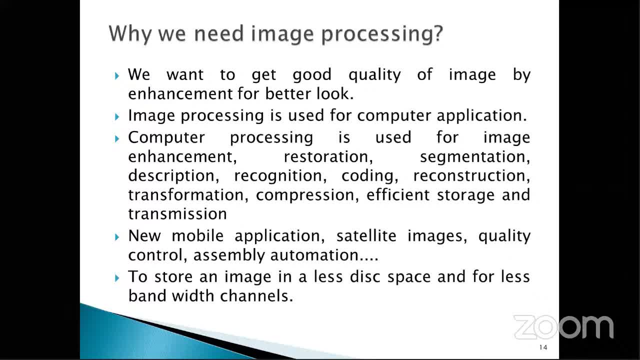 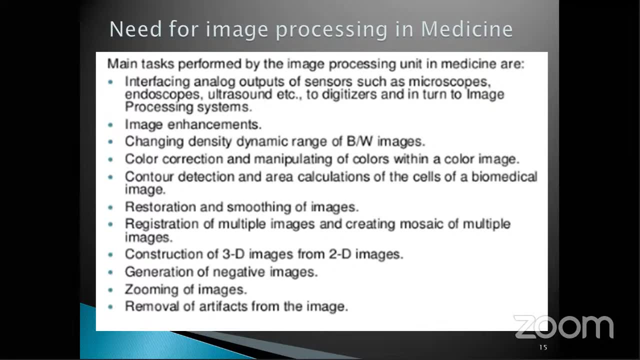 channel, okay. the compression is used for to store the image in less disc space and for less bandwidth channels for transmission purpose. okay. so all these areas we are using image processing main task for performed by the image processing unit in medicine are interfacing analog outputs of sensor such as microscopes, endoscopes, ultrasound, etc. to digitizers and in turn to 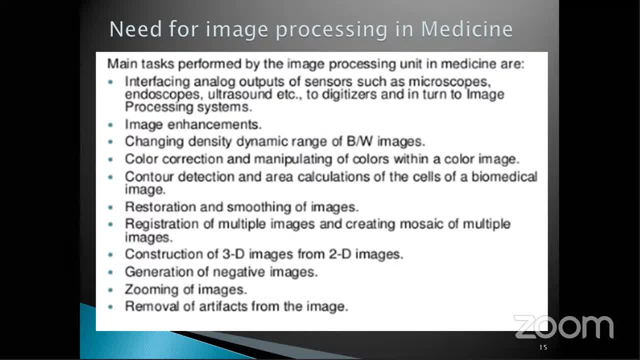 image processing system. okay. so if it is in analog, we cannot process it. okay, if you want to process, if you want to store the image, if you want to analyze again and again, okay, we need some image. that is digital image processing. so it is very, very important in interfacing analog outputs. 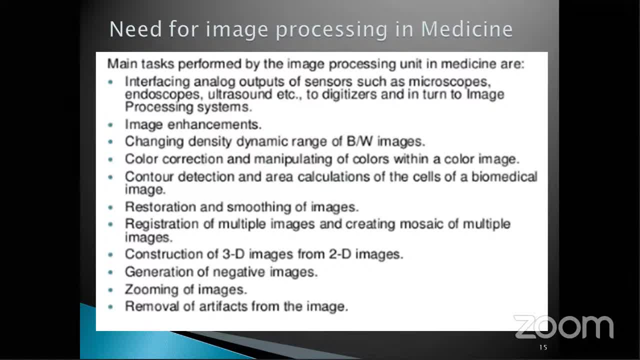 okay, all the sensor are analog cell sensors, for example, ultrasounders. also we are using probes- ultrasound probes in the tip of the image processing unit. we are using probes in the tip of the image processing unit of the probe sensors will be there. so it will take the. it will send some sound waves to the. 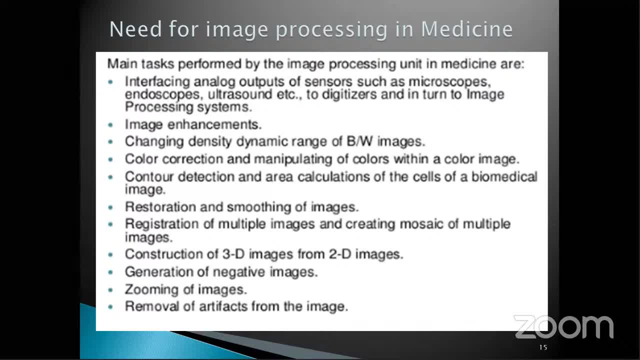 organ and it will reflected back, the reflected back that waves are collected and it will show some image- okay, in the ultrasound images. these sensors okay, such as microscopes, endoscopes, ultrasound sensors- will be connected to computers and it will. we can carry any other image processing. 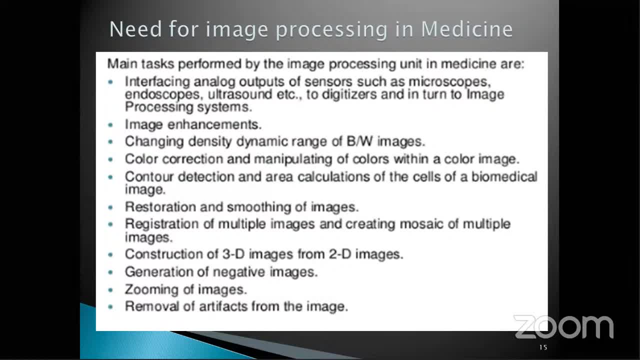 techniques. so image enhancement. so if it is having more noise artifacts we can reduce those things through enhancements. okay, changing density, dynamic range of bandwidth images. okay, sorry, black and white images. so suppose if you want to color the image or shade the image, we can do that color correction. 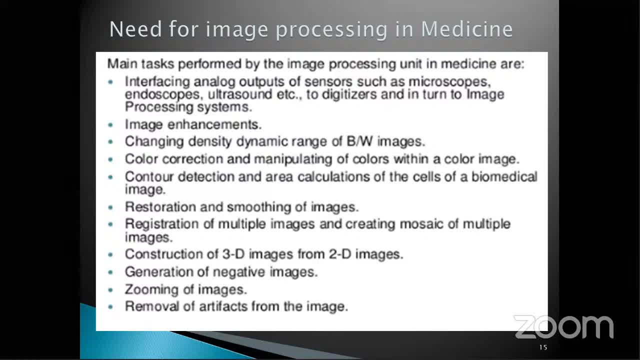 and manipulating of colors. with a color image. okay, suppose we have some color image. we want to change the color, we want to reduce the contrast, the hue, anything we can do, we can manipulate colors. okay. contour detection and the area calculations of the cells of the biomedical image. 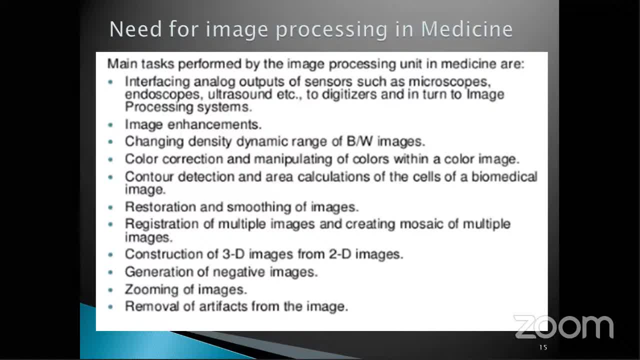 we are. if you are taking a ct scan image of some tumor- okay, tumor cell- in the body, we can calculate the size of the image, the size of the tumor: length, width, depth, everything, volume, everything. we can calculate to this. manipulators and the restoration and smoothing of an image. okay, we can smooth the image. the restoration means we can filter out many. 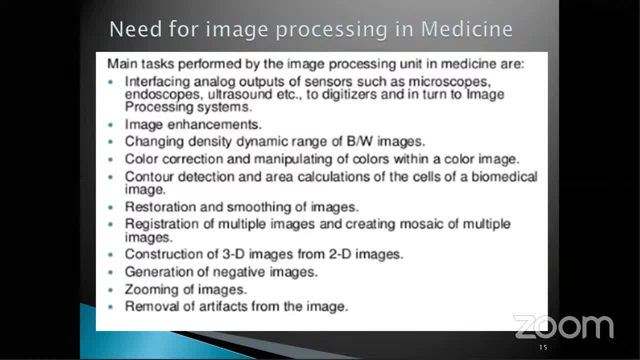 unwanted things. we can smooth the image and the registration of multiple images and creating mosaic of multiple images. okay, in mri images, we are taking more images in the different directions, 360 degree directions. we can take more images. we can mosaic the video. we dangloing昡. 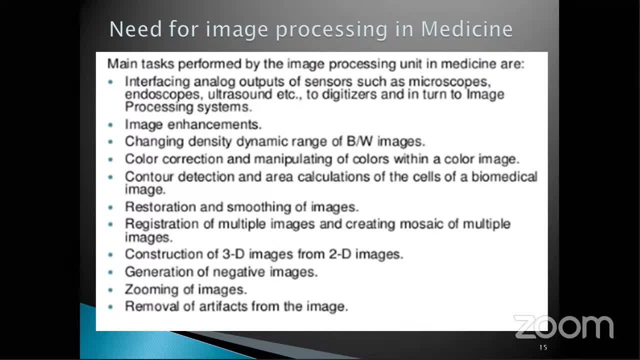 we can take more images. we can mosaic the different image images and we can filter distance two degrees 있는 방식. mosaic means in a platform, in your background. we can collage like collage. we can paste many images. okay, so in different directions we are taking many images. we can put all the images in a background. 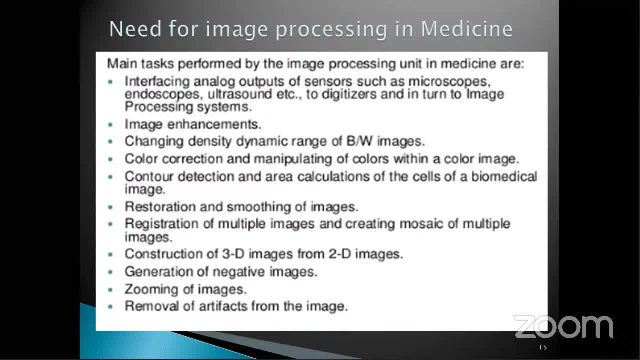 we can compare one image with another image, okay, we can easily understand the abnormalities of the image- person or patients- okay. so registration fusion means combining some two modalities. x-ray and ct will become combined and the ct x-ray we can take, so ordinary x-ray cannot show. 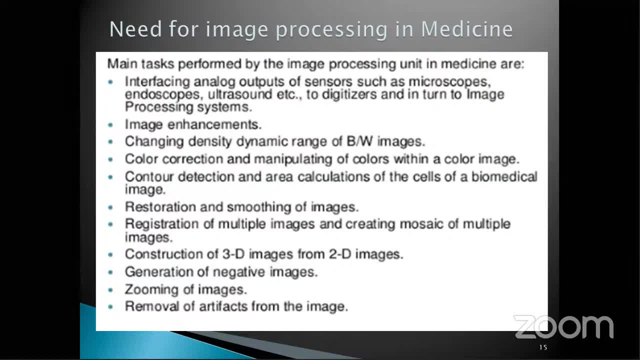 many abnormalities and ct also sure doesn't show many abnormalities. if you combine some some chest ct or whole body ct, we can combine it. it will give good abnormality details and the construction of 3d images from 2d images. okay, this is a technique combining more 2d images, like mri mri. 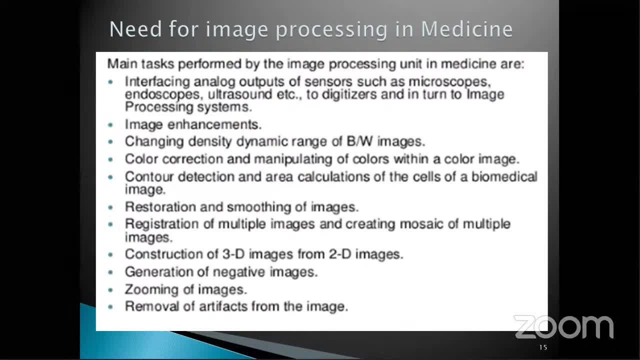 is taking 2d images in 360 degree directions. all the directions and all will be combined. it will give 3d image. okay, we can see the whole structure of the tumor. okay, but it is not taking whole structure, it is slicing. it will take slices. many different slices will be taken. 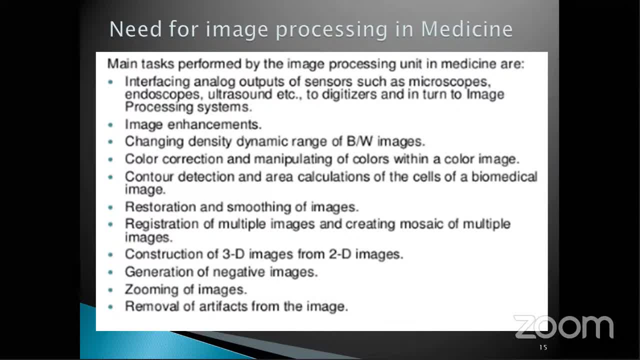 and all will be combined, we can see the 3d image. so that is the construction of 3d images. generation of negative images. if you want to take negative images, that also we can take for storing purpose. afterwards we can create uh, actual 2d image and from that we can take 3d. 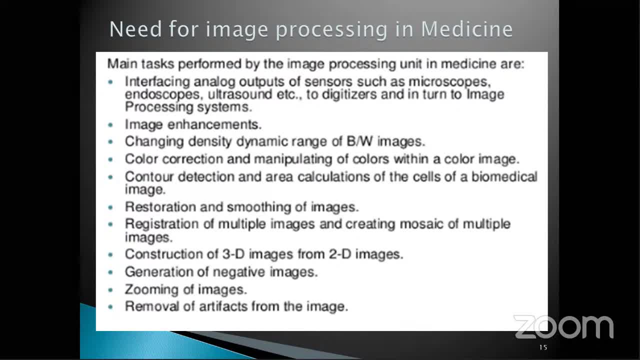 images. so for compression purpose we can store negative images. zooming of images: okay, so ordinarily we are taking some image. we cannot zoom it. okay, if you want to. particularly we have to see some uh object we cannot in surveillance and all in surveillance, object tracking and all many. 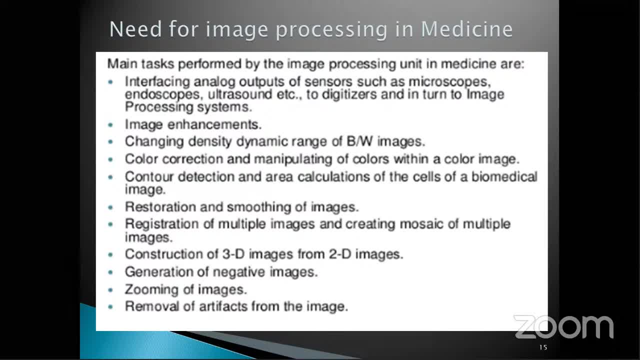 object will be placed in your scene. so we we have to zoom and we have to find some important object. okay, for suppose, india crowd, some terrorist is there. okay, we can find terrorist with zooming. okay, removal of artifacts from the image. so in ultrasound more artifacts will be coming because it's a sound wave now. so 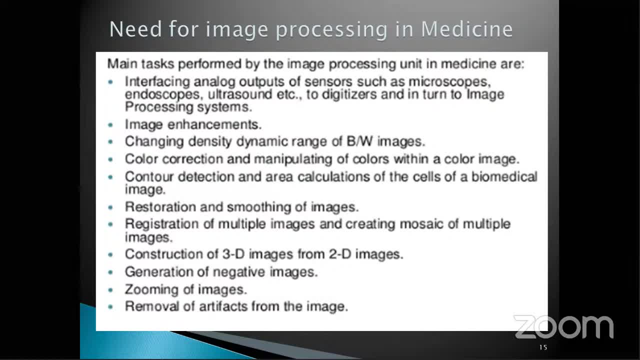 baby also, suppose a pregnant woman is scanned through. ultrasound means baby also producing some sound and the mother also producing some sound. okay, so all will be combined with the actual ultrasound signal and it will be given as an artifacts. so if you remove all the artifacts we can clearly view the baby and if any abnormality is there, that 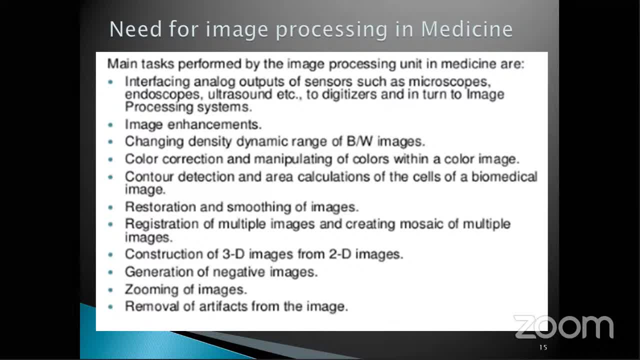 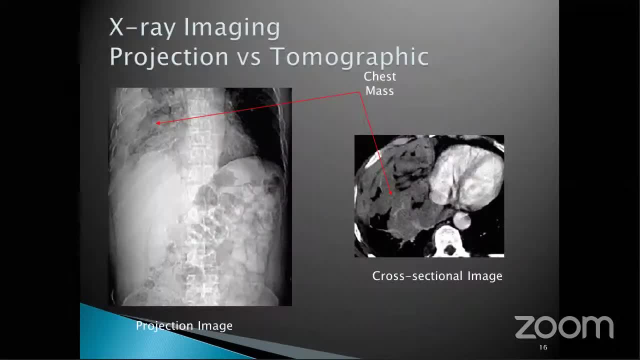 also we can see. okay, so, like the kidney stones, gallbladder stones, anything we can see. this, uh, ultrasonic images, ultrasound images. next right, see here it's a tomogram graphic image. but in the x-ray we can see this this much. we cannot see this much clarity. see here: one slice is given. so 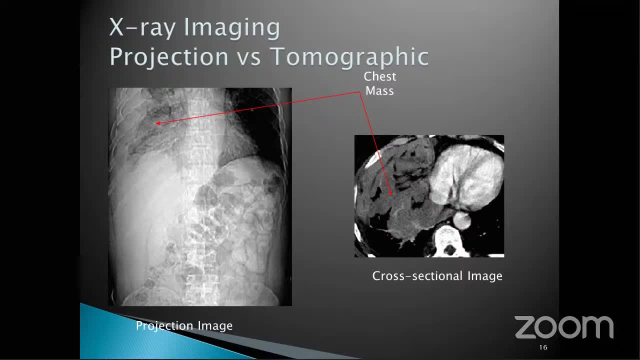 this slice is taken from this area. okay, from this extra x-ray we cannot see this, what is present inside this, but through ct we can take the slice. okay that in from the slide see here. so many objects will be seen inside this. if i suppose here some lump is there, we can see the tumor or lump, okay. 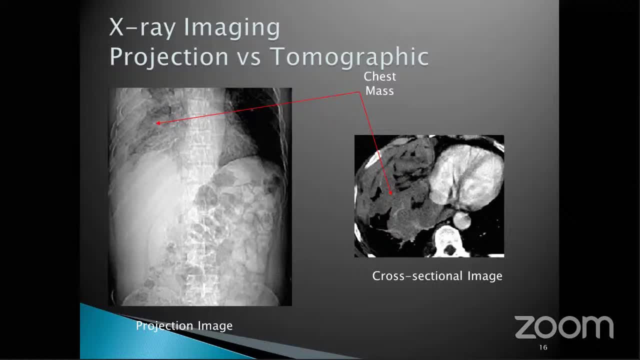 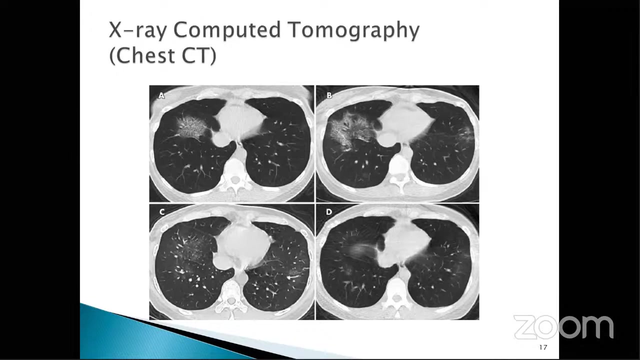 is the cross-sectional image. so what is the use of mri and ct means we can see the cross-sectional image because it is taking 360 degree directions, all the direction. it is taking some images, okay, next slide. so this is the ct lung chest, ct. this is lungs. see the uh. this is one uh projection of ct. 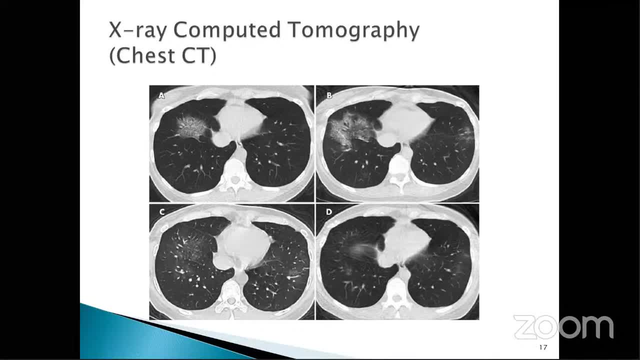 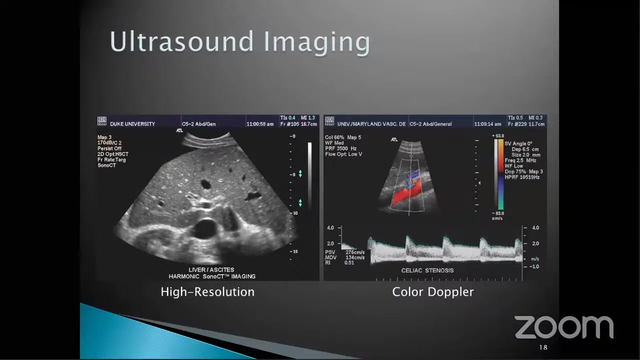 here it is some problem, some pneumonia. this patient is having some pneumonia here. some flum will be formed. the congestions: this this shows the congestions. so this is the x-ray computer tomography. here x-ray and uh ct will be combined. okay, next line, this is the ultrasound imaging. okay, ultrasound image. we are sending some uh rays inside our organ. 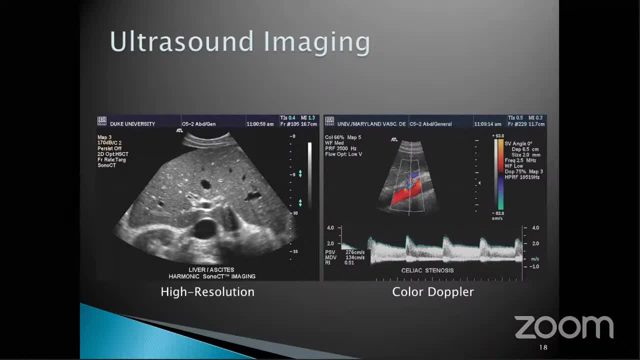 the reflected waves will be collected from that. uh, the organ will be shown. it's a color doubler. we can use colors also color doubler. so through image processing only we are doing all this color mixing and all okay inside our body, uh, that colors will not be appear outside in this image. see here only. 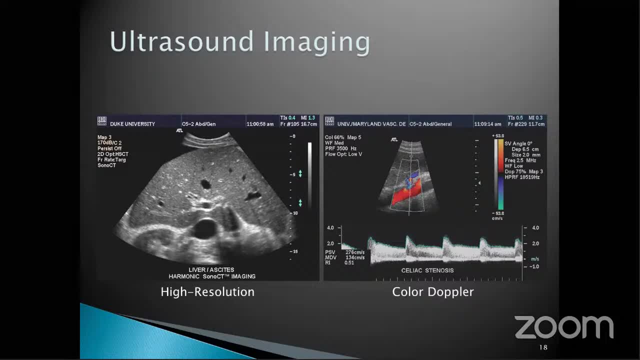 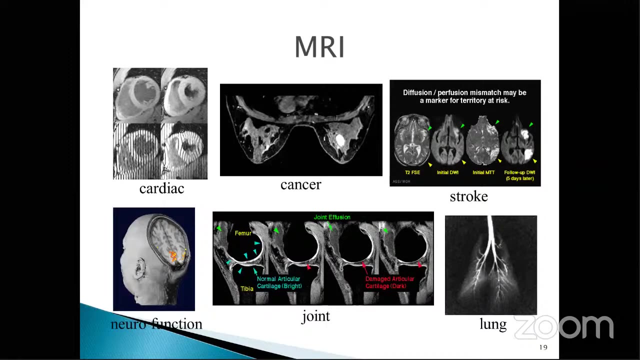 grayscale images: black, white. some gray levels are there, but here some. this is pseudo colors. we can use pseudo colors to see the images next slide, please. this is mri image. okay, see cardiac image through mri. so many types of images. okay, many organs are taken as a image- cardiac. this is mri through mri modality. cardiac image, cancer image: see here. 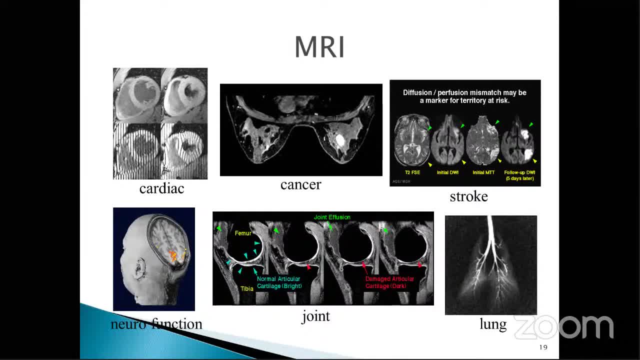 cancer image and stroke. so, stroke for stroke, they are taking skull image. okay, here brain image will be taken. this shows different slices. okay, different directions, different slices. they are taken and see, here this is one cross section of our skull and here different veins. okay, so here we have lines, bones, femur bone- okay, femur bone joints. see this. 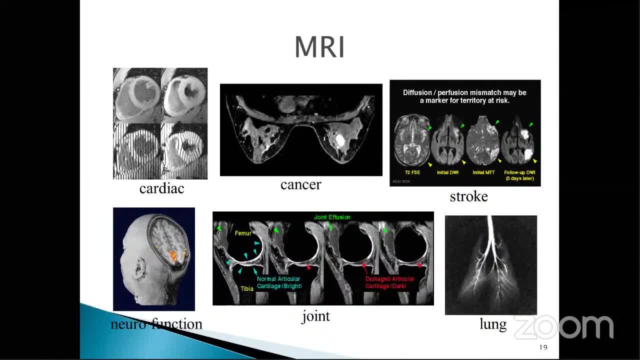 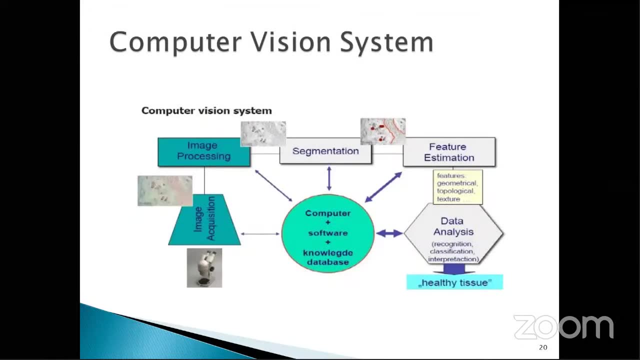 pressure, normal or abnormal, or having any injury. we can find easily through mri and this is lung inside lung. we can take the lung also lung mri. comparing to ct, mri is best for our uh health. okay, ct is having its combination of x-rays. okay, x-ray in different direction, that is ct, so it will give. 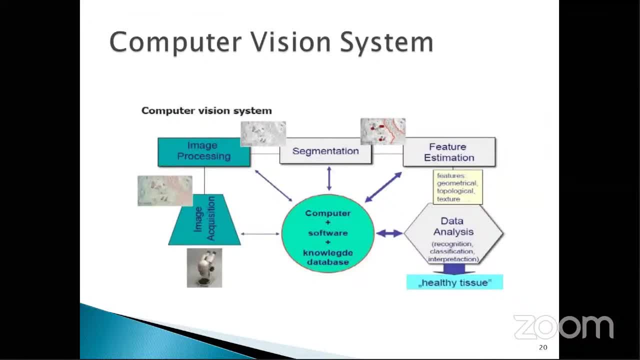 some radioactive emission, it will be harmful to our body. but mri is magnetic resonance image. so magnetic field is applied on our body and it will be converted into image, so it will not affect our organs. so computer vision system, what is meant by computer vision system? so for computer: 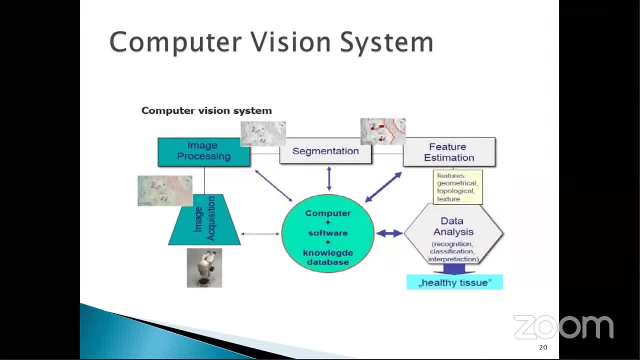 processing, computer image processing, we need to have these blocks, okay. so what are all these blocks? this is sensor- okay, for example. it is a camera- okay, so here we are acquiring images from camera. okay, so this acquired image will be processed. so in image processing in depth, we have many. 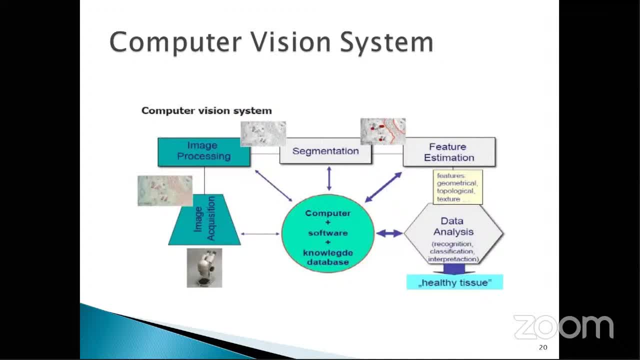 processing, segmentation. see here. segmentation we are capturing some abnormal parts, abnormal area from the image, particular image. so this is segmentation, okay, and features estimation. so segmentation means we are taking, we are extracting some tumor. okay, so from the tumor we are taking many features. what is the size of the tumor, tumor, what is the volume? 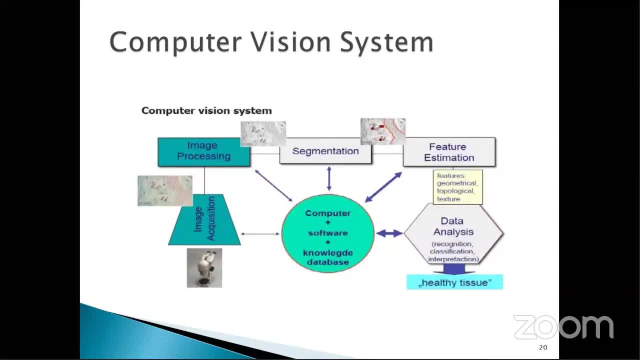 of the tumor where it is placed, from chest it is, how much depth it is there. okay, so like that features we can estimate. from this feature we can use data analysis. it is used for recognition, classification whether the lump is in early stage or advanced stage. like that analysis we can do. 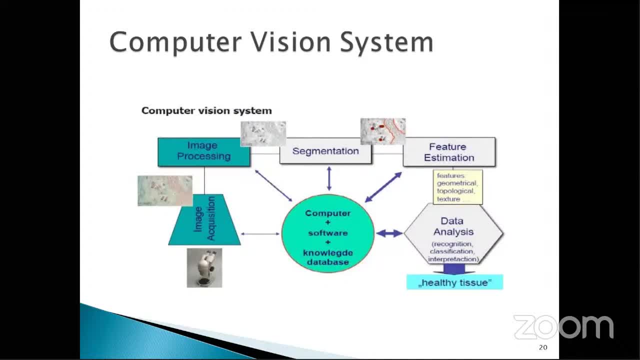 okay, or it is the healthy tissue, so that separations, that the separation, we can do. classification: okay, it is a normal or abnormal, we can do so in the computer image processing. we have computer software and knowledge database, okay. so i am using different algorithms to process my image, okay. some other person use different algorithms? okay, advanced. 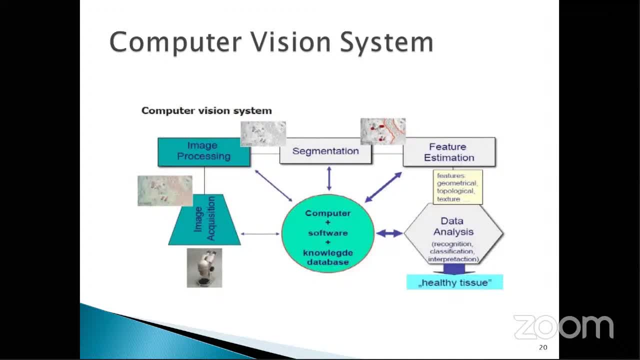 algorithms they can use to process their image. i want to use some filtration, i can use some fusion. i want to fuse two or three images means which i can use. so this is the computer image processing. okay, digital image processing, if for that we have these blocks. okay, image acquisition: we need to have 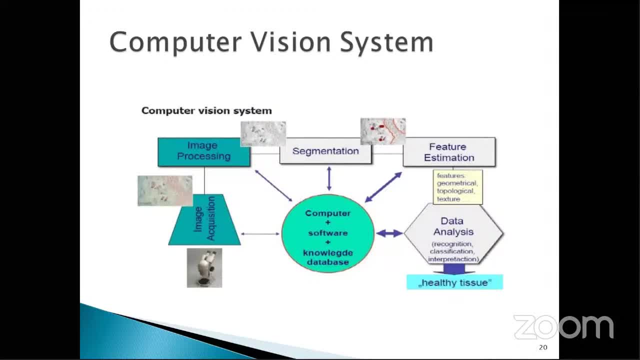 image acquisition. for that we have. we need some good equipments, imaging modalities- it can be x-ray, ct, ordinary digital camera and then any other thing. okay then image processing, segmentation, feature extraction and data analysis. this is the computer vision system. the total system is called computer vision system. next, 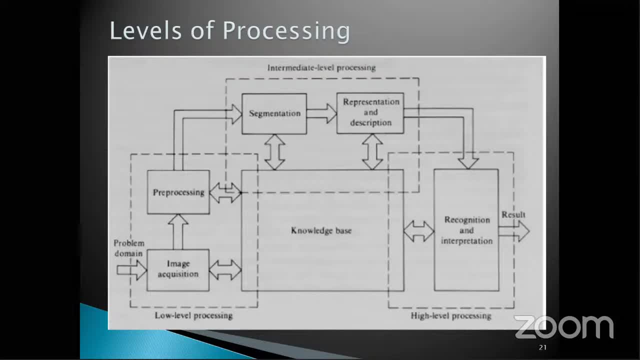 so levels of processing. okay, levels of processing. so we are in computer vision system, the whole as a whole. it is called as computer vision system. so in that system we are classifying as low level, intermediate level, high level. okay, so the high level, all these are using this knowledge base. 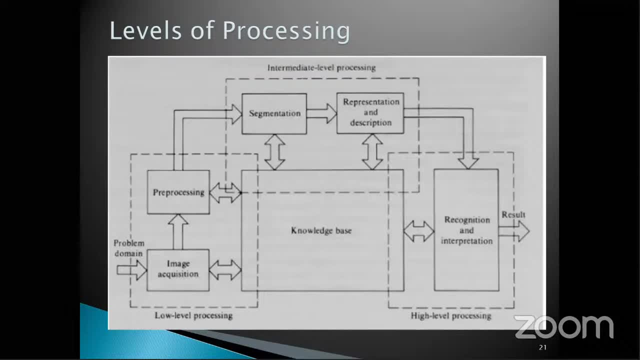 okay. all these are used by knowledge base. so here low level means image acquisition. it may be anything, can be any image acquisition. it can be any image acquisition. it can be any image acquisition camera or x-ray ct. any image processing, any image acquisition. okay, and here pre-processing. 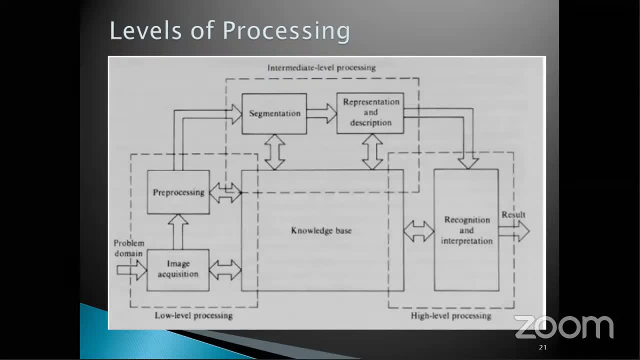 okay, this is also using this knowledge base. knowledge base means our uh utility, okay, our utility on this image. whatever algorithm, whatever pre-processing, whatever enhancement i need to use, we can use. okay, so many image processing techniques are there? image enhancement techniques are there. in that, what i want to use, we have to select and we have to use them pre-processing and see after. 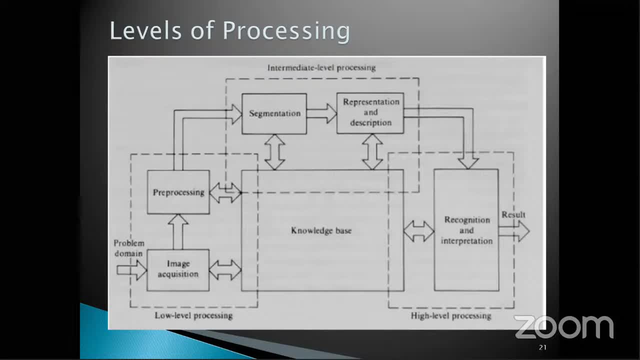 pre-processing, intermediate level processing. so if any some image need not use this intermediate level after pre-processing i can use the image as it is no need for segmentation and description and all representation, the description and all i don't need. okay, so from pre-processing i can use the image. otherwise i need more image processing. 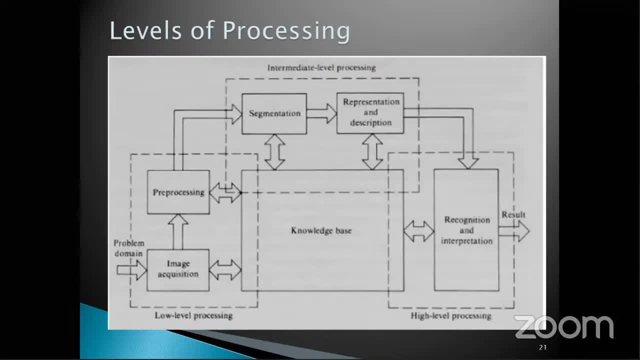 i need more color image or i need more clear image. i need to go for the segmentation techniques. okay, segmentation representation- how i can represent the image, so clear or neat image we can represent. for that also i know i need knowledge base. i need to use some segmentation. 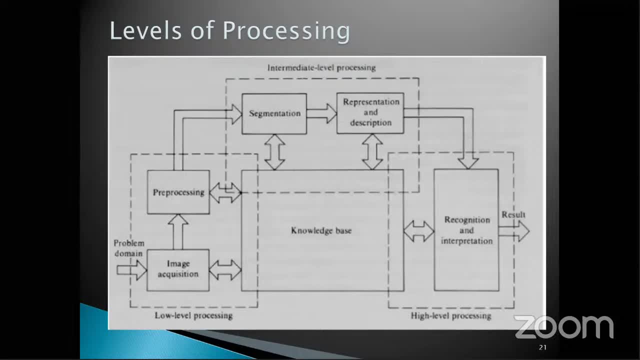 methods. it's a low level measure method or a high level programming, anything i can use okay. so this, this also needs some knowledge base. so then recognition: okay. recognition means, if i want to fuse two or three images, i can fuse. i can take any image. features: number of n: number of features are there. 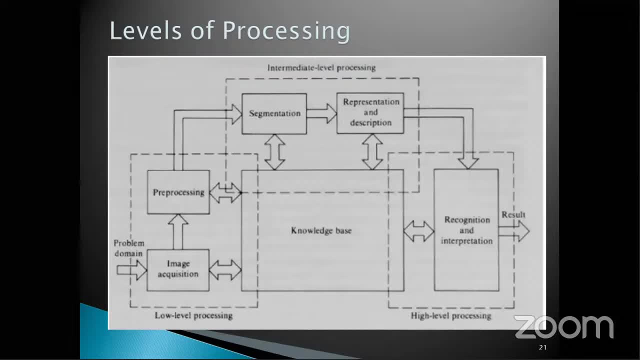 so what are the features i want? i can use that alone, okay, using this image. uh, features- you can use a number of features. i can classify the image. okay, at last i can classify the image. okay, it's a normal image or abnormal. if the lung ct is taken means we can find it is corona, is there or not. 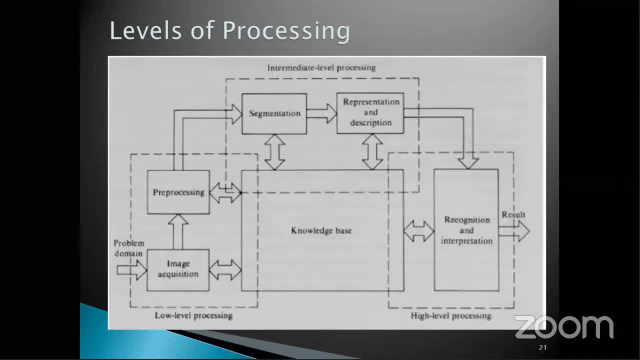 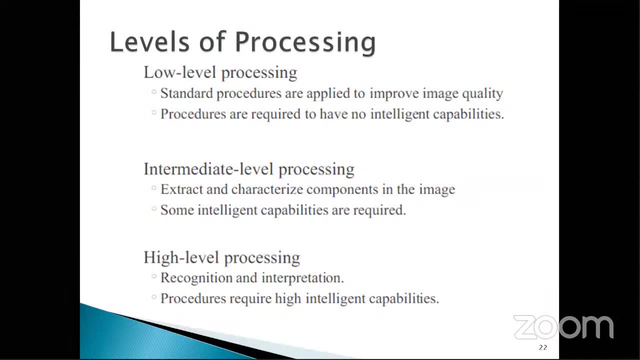 okay, using this, image clarity and enhancement and all next. so this is the levels of processing. higher level processing: standard procedures are applied to improve image quality. procedures are required to know intelligent capabilities. so here no need of intelligent capabilities. intermediate level processing extra and characterize components in the image, and some intelligent capabilities are. 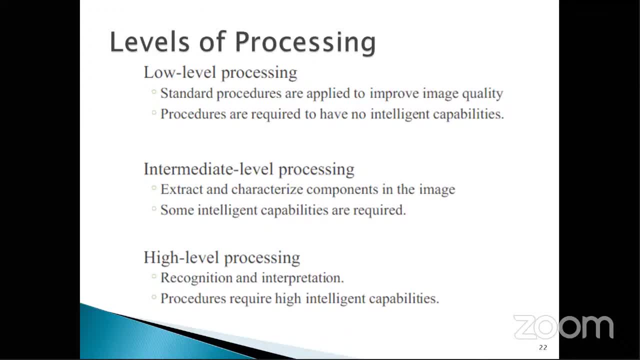 required. so if you want to build a new program, new software, you can use that to get more, more compatible results. okay, high level processing, recognition and interpretation: okay, so i am interpreting, i am showing this result to the patient. i am showing this result to the patient, i am showing the result to some other usage. so, recognition and interpretation. 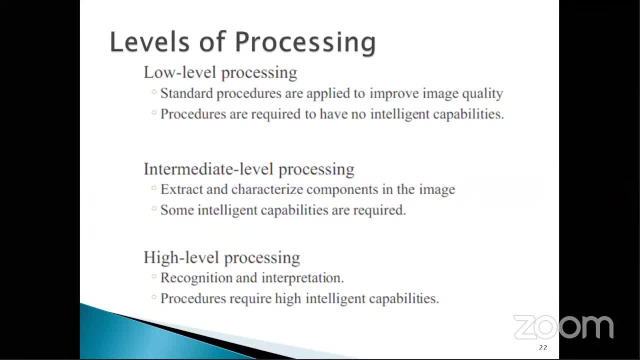 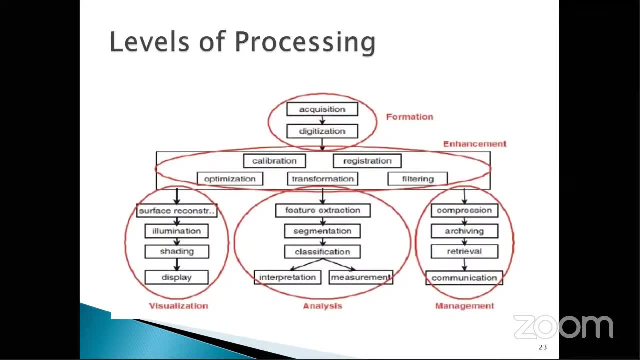 and procedures, okay, require high intelligent capabilities. next slide: so see, this is also class giving the levels of processing. so first here we are starting from here: formation, image formation in this formation, acquisition and digitization. we are taking image, that image is 2d and we are creating this image to 3d using some digitization techniques. 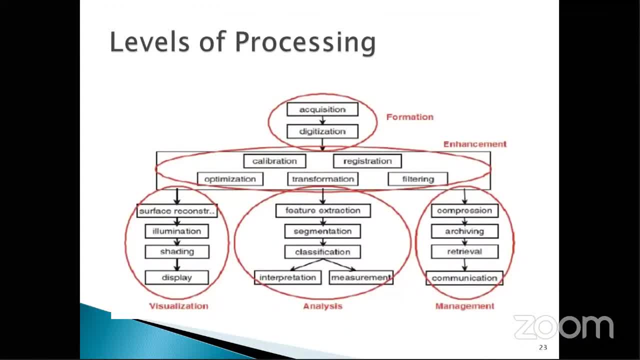 okay, formation, so acquisition and digitization is the formation and enhancement technique. the image: if the images are containing some unwanted noise artifacts, we can clear those things through enhancement. so enhancement technique means calibration, registration, optimization, transformation, filtering. so these are all some enhancement techniques. okay, en이면, enhancing methods, usually in a particular image visualization okay. 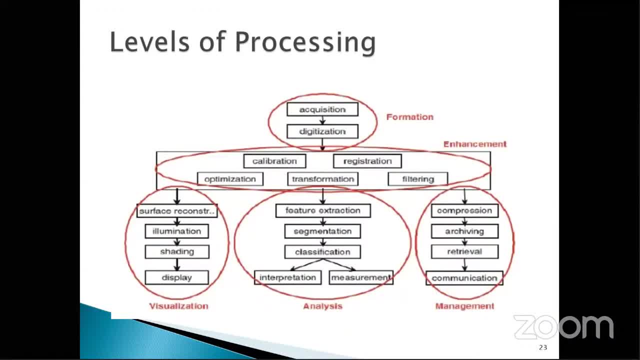 so surface reconstruction illumination, suppose, if image is taken in dark shades, okay, it is not clear, it is not bright, okay, so illumination correction, meaning you to lightning only. okay, some areas will be bright, some various will be dark. so we need clear image means we have to correct the illumination. so on the whole, all the pixels should be in same illumination means we can. 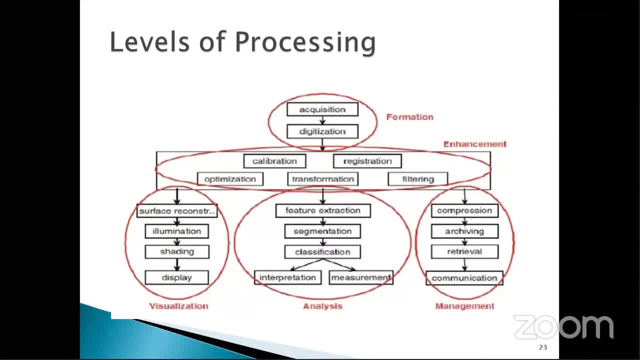 get the clear image. so this illumination correction: before processing, we need to correct the illumination and shading. okay, so what are all the unwanted area we can shade or what are? what is our region of interest? okay, what is our interest? that area will be shaded in color shading or 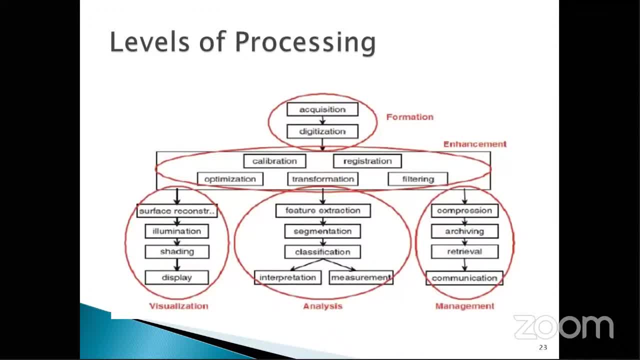 a normal shading grade level, shading and we can display. okay, so if you want to go for analysis after visualization, we have to use this analysis. okay. so in analysis, what are what are all there? feature extraction, segmentation, classification, interpretation, measurement. okay, so analysis contains all those things from the enhanced image. we can do this. okay, after analysis management. 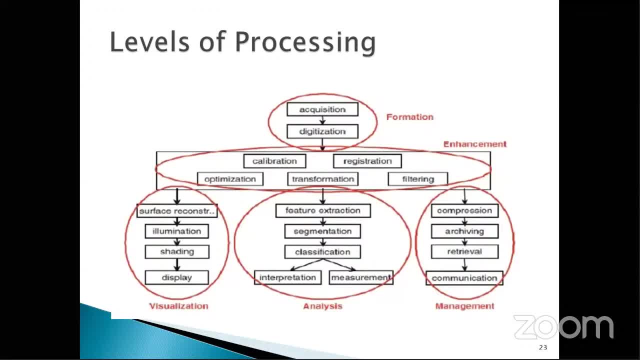 management: okay, management means how we can store the image. it should be lossless, medical, normal image means we can use lossy techniques. okay, storing the image, compressing the image. some lossy techniques will be there. we have to compress the image. we can store in a less space: okay, in a pen drive or some. 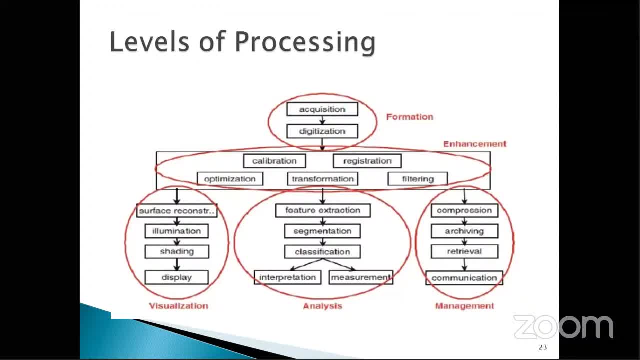 disk. but for medical image, we have to use lossless techniques for compression, because if any information is lost, we we will miss the data. okay, important data, we will miss it. so for a medical imaging, no need of loss compression, loss compression, okay, we have to use lossy company lossless compression and archiving. 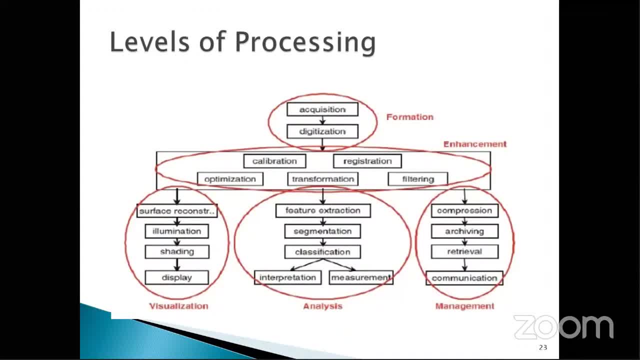 means we have to store in your database. okay, whenever we want, we can take that image and we can analyze. okay, we can show so next time the patient is coming and showing some other image means we can analyze. okay, we can show so next time the patient is coming and showing some other image. means 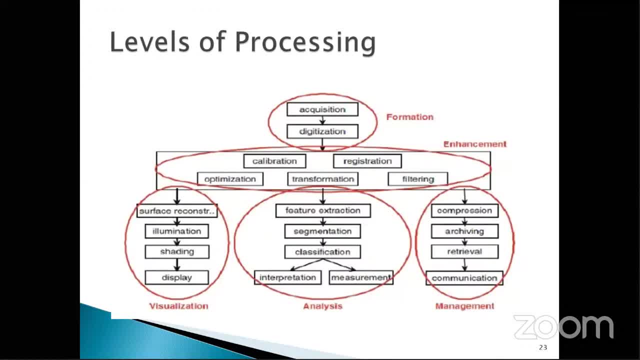 we can compare that image with previously stored image, so how the problem will be increased or decreased, we can analyze. so that is management and communication. okay, if you are transferring that image from one place to another place, the data data will using reduced bandwidth. okay, so data data will be reduced. so compression is helpful for this data reduction, so it is used. 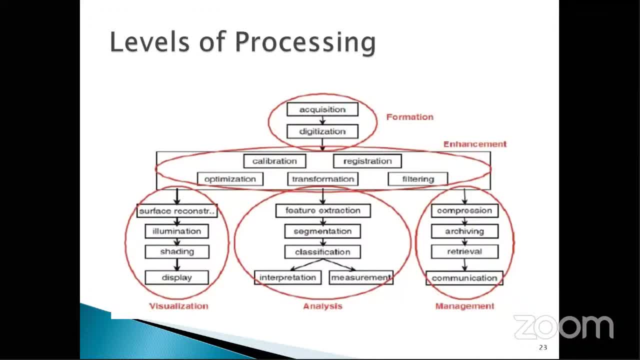 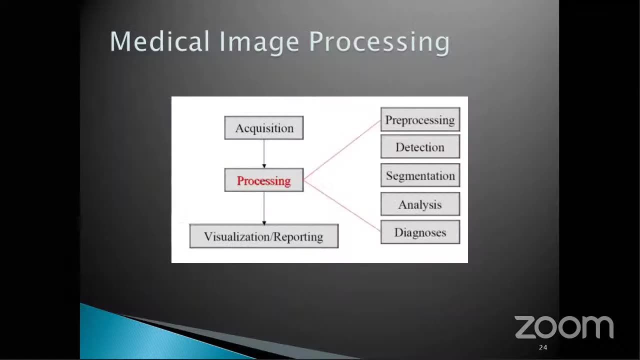 for communication. so these five component- formation, enhancement, visualization, analysis and management- these are all required for digital image processing or medical image processing. okay next, so this is also showing same same thing: acquisition, pre-processing and visualization. so in acquisition we know different modalities are there. from that modality we are acquiring images. 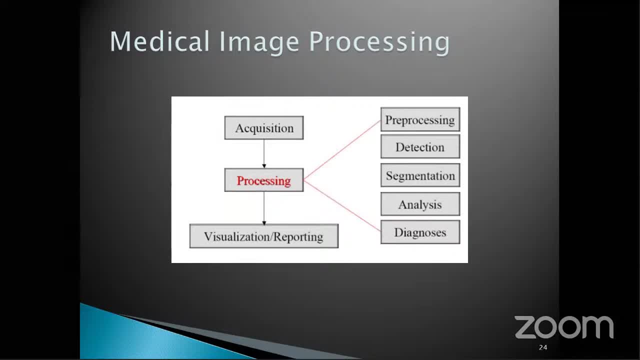 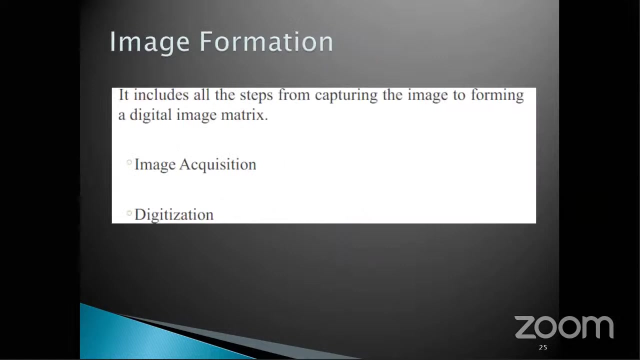 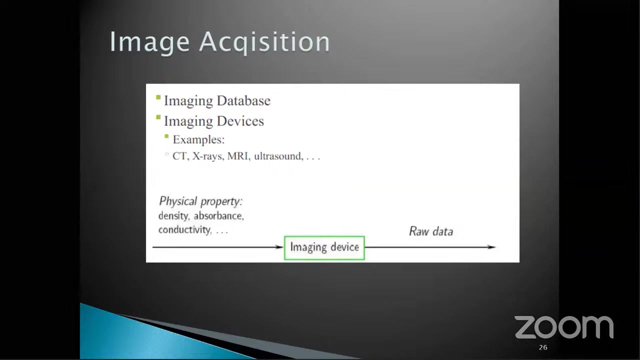 okay, from object, then processing. this processing have these segments: pre-processing, deduction, segmentation, analysis, diagnosis. okay then from processing, visualization. so previously also we saw same thing, only next one. so image formation means image acquisition and digitization. image acquisition and digitization, next slide, so in. uh, this is the imaging device. image acquisition: okay, it, it may be ct x-ray mri. 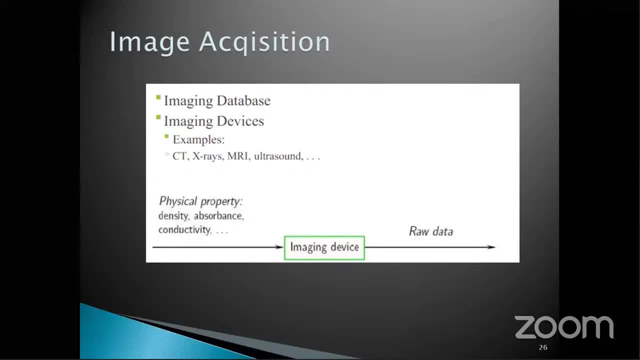 ultrasound, anything, okay. so, physical property: the density, observance, conductivity, okay, these properties will. using this properties, we are taking some image. okay, we are increasing the x-ray capability, x-ray, uh, attenuation of the image. so this is the imaging device: image acquisition. we are less decreasing the x-ray attenuation. okay then, uh, amplitude will be increased, like that some. 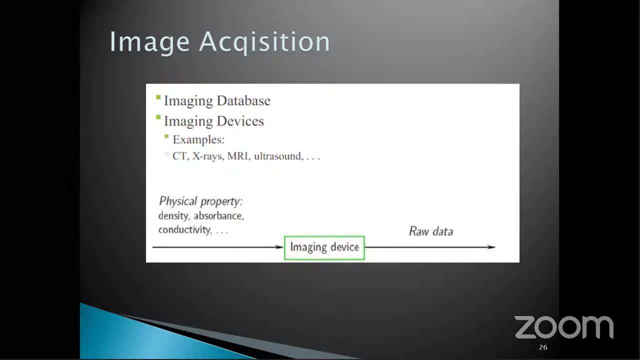 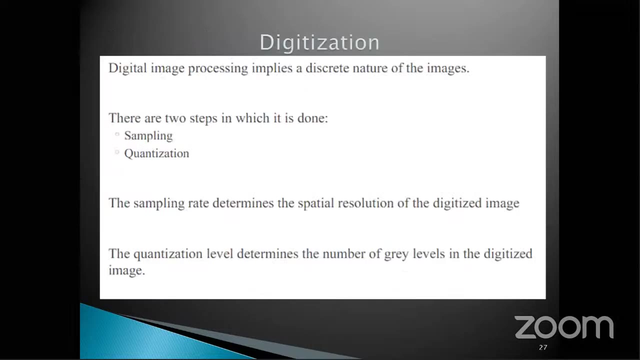 physical property we are taking the image. from using this imaging device, we can get the raw data. this raw data means what it can be mixed with: some artifacts, noise, anything. okay, next slide. so digital image processing implies, yeah, the image processing here. loosing 즉xial neighbourhood to the external literature is part of technical web processing. so we havestarter information here: cnt bathroom data, data. data data means what it can be mixed with: some artifacts, noise, anything. okay, next slide. so digital image processing implies: here there are many options for digital image processing, so dynamic~~. 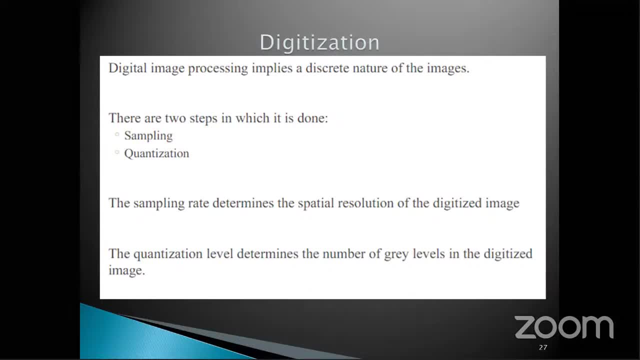 discrete nature of the image. so analog means analog nature. okay, we cannot easily process the image. we cannot process the computer using computer. so digital image we can easily process through computers. there are two steps in which it is done: sampling and quantization. okay, the image is divided into different samples and it will be quantized. okay, the sampling rate. 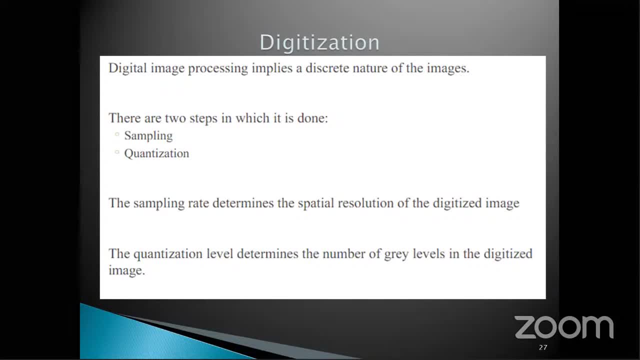 determines the spatial resolution of the digitized image and the quantization level determines the number of gray levels in the digitized image. so this gray levels means we are dealing with. if we are dealing with gray levels, black and white image or gray image, we are using this number of gray levels in the digitized image. okay, 2-bit image. 3-bit image. 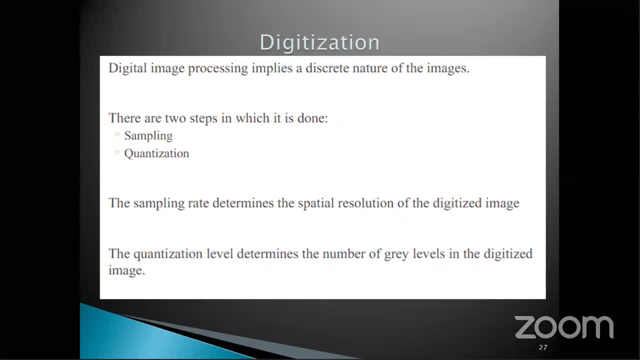 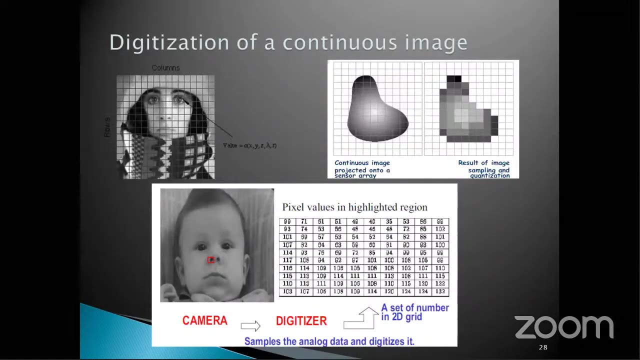 okay, 3-bit image, it means 8 level of gray levels. okay then, 2-bit means 4 level of gray levels. so, like, different grade levels will be there in digitized image. next slide: please see here: digitization of a continuous image. this is a continuous image. see the whole. 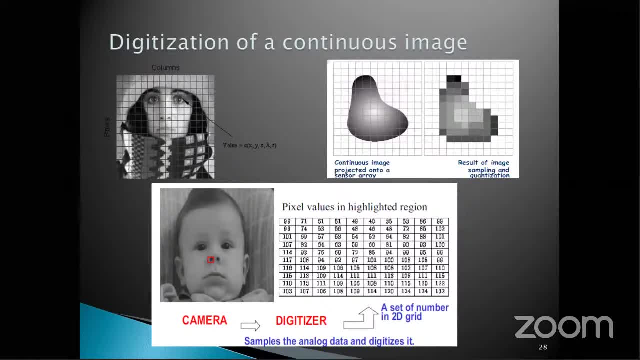 image: a lady is there, okay, wearing some muffler. this is a whole image, continuous image. but seeing this image, lot of squares will be there. these are all called the pixels. okay, this is some 41 into 40, uh, 41 into 15 image, that is, these are all rows, these are all columns. 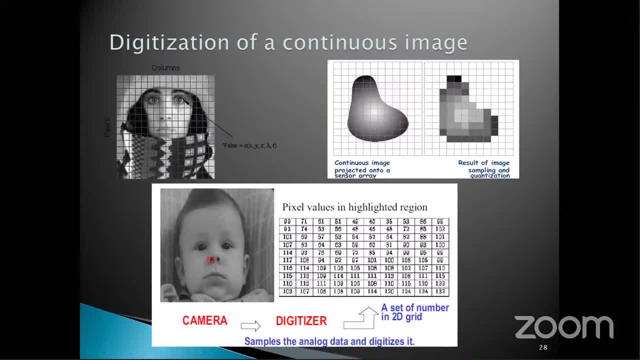 the image is divided into rows and columns. it will be um given as a pixels. what are the pixels? pixel values. pixel values means the intensity of the image first. this pixel is having some intensity. this pixel is having some intensity, so this intensity of the pixel is given in this matrix. 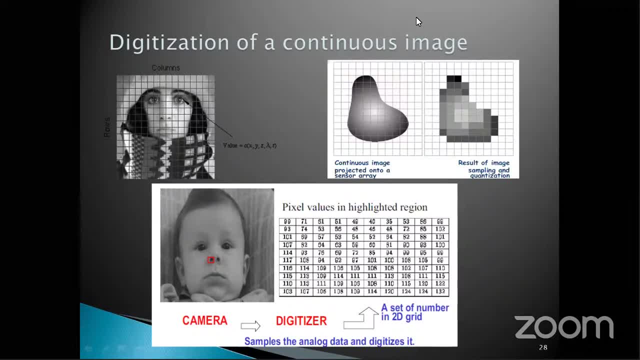 form: okay, so rows, columns: okay, see here. this is a here an image, here this a highlighted area. okay, this is highlighted. some. this area is highlighted in this area, how many pixels are there and what are all the pixels? intensity: this will be highlighted here, the very small area. 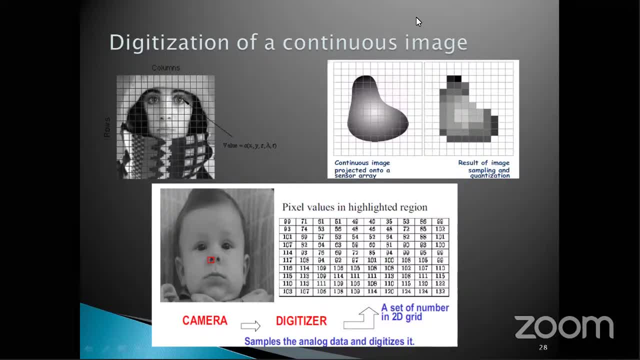 see here this very small area, some 10 to 11 rows are there and here also some 10 to 11 columns are there. so in this particular area, 10 rows, 10 columns are there. okay, so we are taking this image using camera through digitizer, we are digitizing the image. 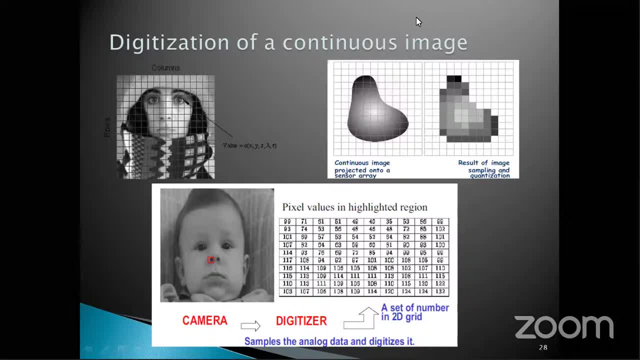 how it will, digitized using sampling and quantization. okay, digitized. and a set of number in 2d grid. this is called a set of number in 2d grid. so these are all intensity values of the pixels. so this is the intensity value of the pixels and here, see here y. okay, equal to. 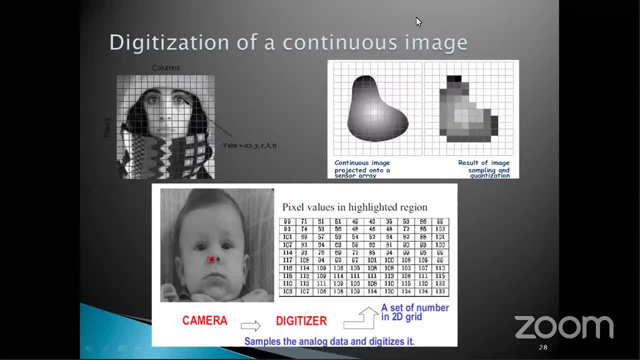 x comma, y comma, z lambda. some parameters will be given. so here, x and y are coordinates. in which row, which column this pixel is present? okay, coordinates means f of x comma, y. no, f means intensity: x is the coordinate, x axis coordinate and y is y axis coordinate. so this pixel, this pixel's intensity. 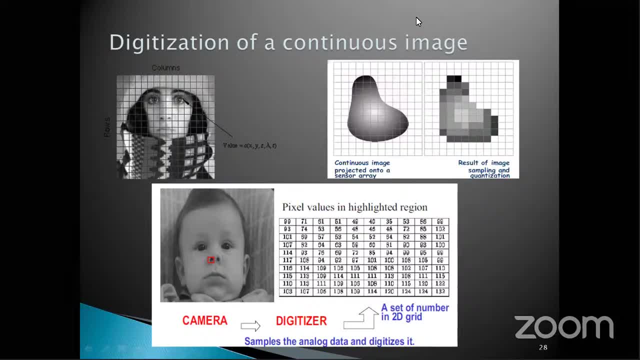 is 99. see here: the pixel intensity is 99. how i can represent the image: f of x comma y, 99 of 0 comma, 0 or 1 comma 1. suppose this is the first row, first column. okay, this is the first row first. 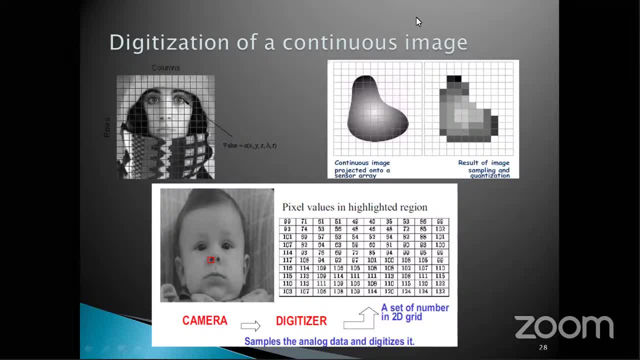 column this pixel. so how i can represent this pixel: 99 of 1 comma 1 because it is present in first row and first column. so i can represent f of x, y means 99 of 1 comma 1 if i am representing this pixel. okay, one, two, three, four, five, six. okay, this is first row, sixth column. so this intensity is this. 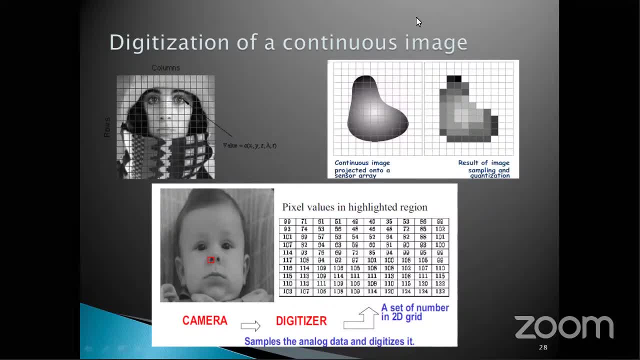 sixth intensity, one here, 40.. intensityここ 1 rock. 6, column. okay, 40 of 6 comma 1, comma 6. so first row, sixth column. so i can represent this pixel as a uh in digitized form: intensity with the coordinates: okay, so this is the digitization. 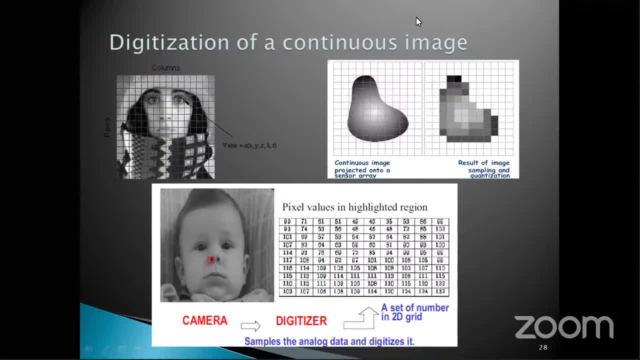 of continuous image. see here some image. instead of this lady image, some image is given okay, and it is uh grayscale, uh shades, okay, so this is one grayscale. see here, this is one grayscale. and this is some other grayscale, and this is also some other grayscale, this is also some other. 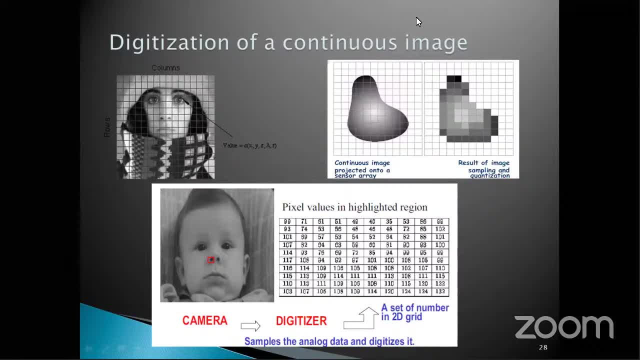 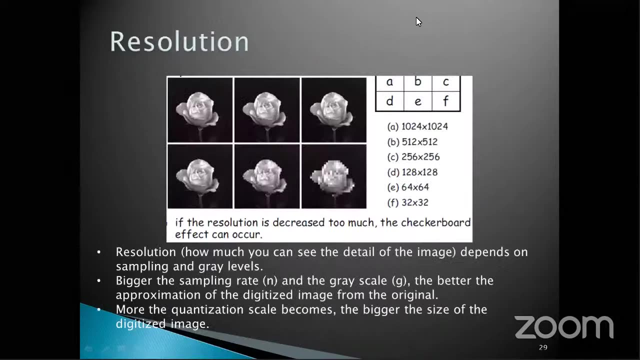 pixels, some 8 bit representation. okay, so 2 to the power, 3 means 8, so 8 gray shades will be there. okay, so digitization of the continuous image. next slide. please see here resolution. what is meant by image resolution? okay, it depends upon sampling and gray levels. So how many samples I am taking in the image? okay, So 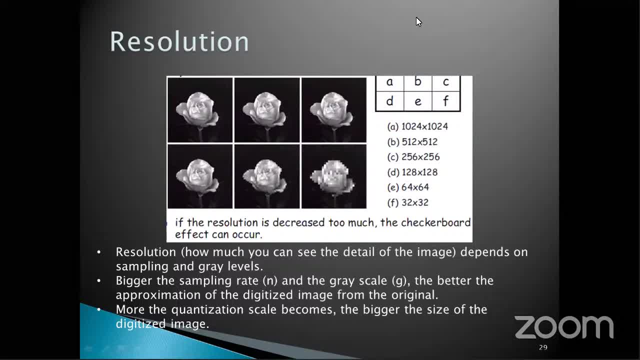 if I have more sampling I can get clear image. If I have less sampling somewhat, it will be less clarity. So resolution: how much you can see the details of the image. So in an image if you see some important minor details, it will be called as clear image. okay, See here. 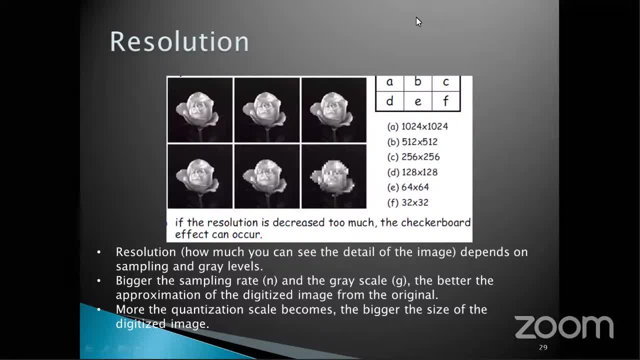 some steps are there. okay, This is due to quantization. It is not having smooth edges. okay, If the quantized values will be very less, then we can get a smooth image. See here: totally all step okay. Some step like some square. many squares are seen, okay. 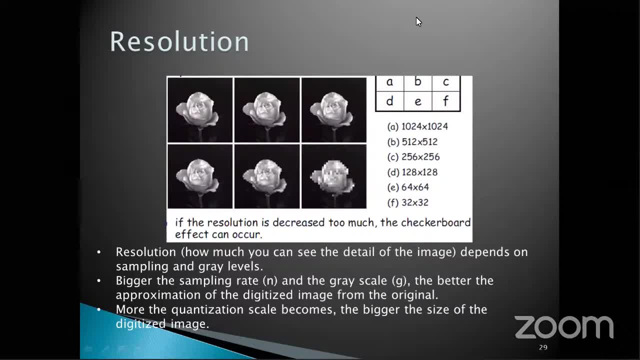 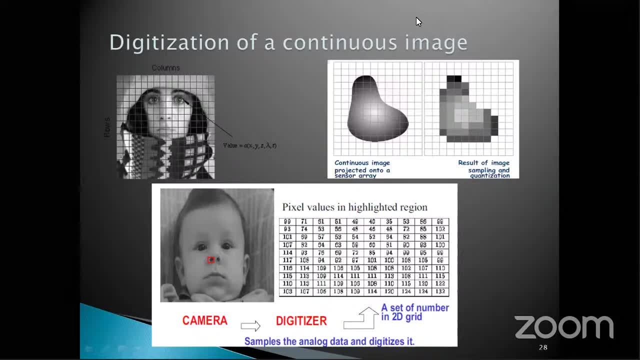 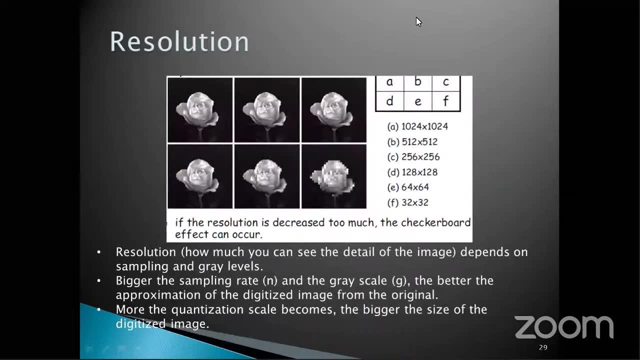 So if I have more sampling, I can get clear image. So if I have less sampling, I can get clear image. See here previous slide. previous slide. See here: different shades are there all represented in some boxes, inside some boxes? okay, Next slide: Like that, this image also. 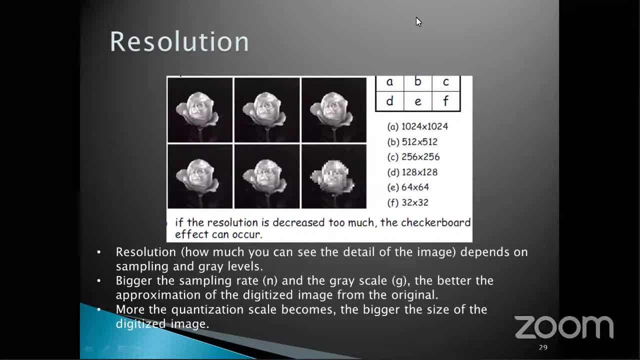 sampled and quantized. okay, See here, this image is having 1024 into 1024.. What it means: 1024 rows, 1024 columns, okay, So what is the multiplication of these two number? That much amount of pixels will be present in this image. first image, A image: 1024 into 1024,. 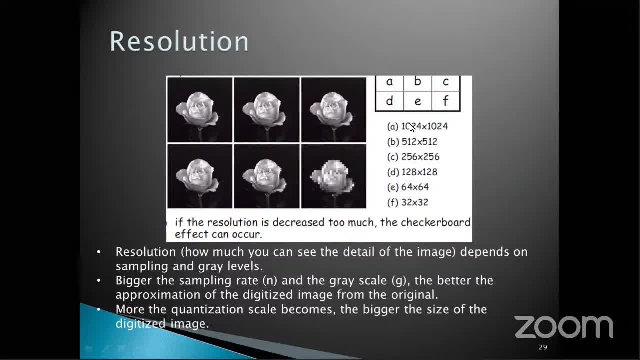 okay, That much pixels are available in this image. That is why it is clear than this image: okay. Second B image: 512 into 512.. Here some 65,000 pixels will be present. okay, So the multiplication value: that much amount of pixels will be present. It is less. 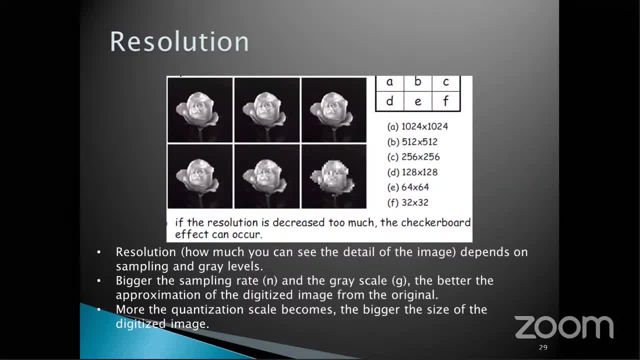 clear than this. See here it is 256 into 256.. This is 128 into 128,, 64 into 64,, 32 into 32.. So if less number of pixels will be there means okay, Or gray levels okay. So if the gray levels 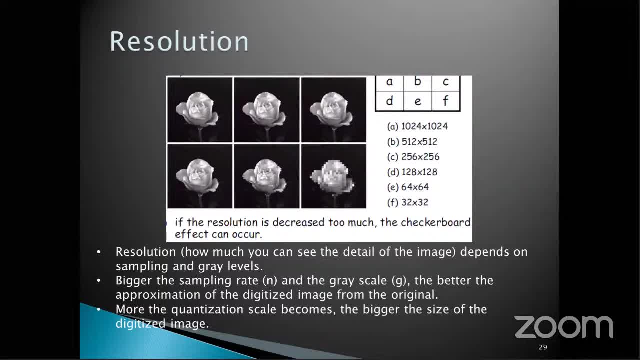 are reduced, if the pixels are reduced, we can see the checkerboard effect. See this checkerboard effect. checkerboard, checkerboard, check, chessboard, black and white. okay, We will see this checkerboard effect. So bigger the sampling rate and the gray scale, the better the approximation. 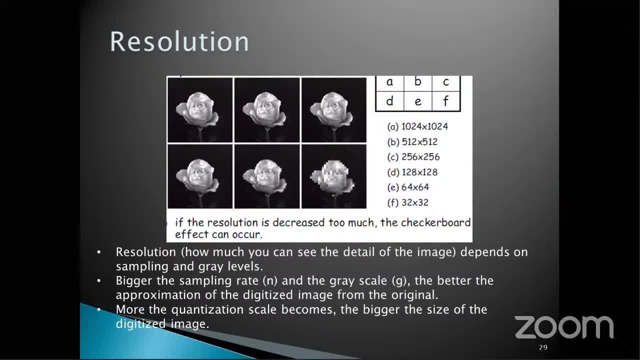 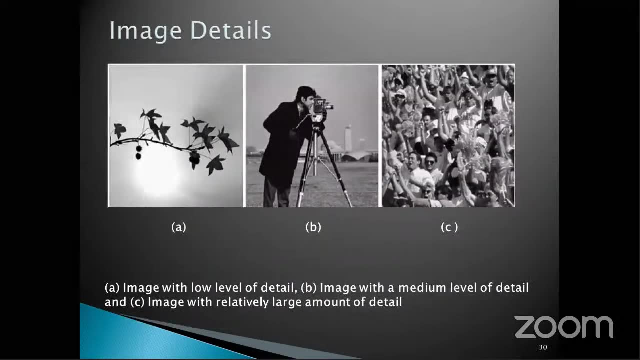 of the digitized image from the original. More the quantization scale becomes, the bigger size of the digitized image. So here the sampling and quantization plays major role in digital image processing. Next slide: ma'am See here this image shows low level of detail. We see background In that background, some sun or 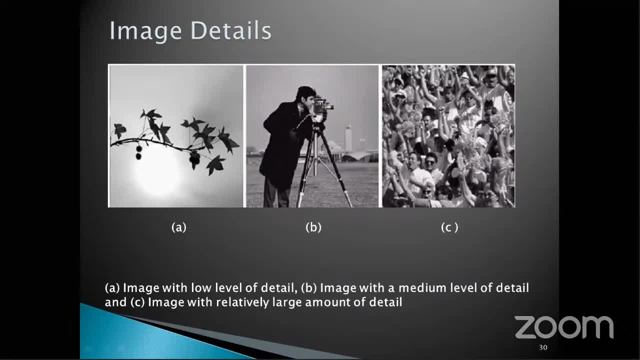 some lighting is there Before that. this is background, This is foreground. Some leaves are there, okay, See here, this is background In background itself. many images, okay. Some buildings are there. trees, oxidized leaves, have greater roles in programming, So here the image shows the hyp染 field. 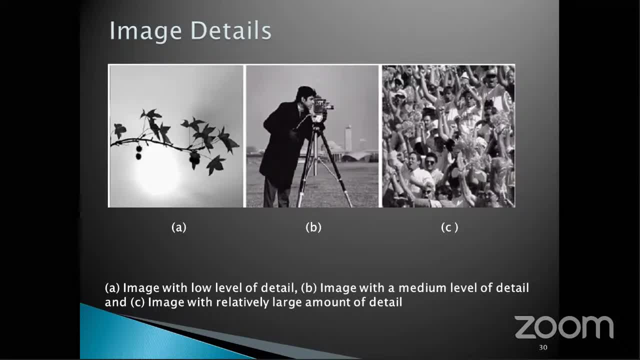 the top of the field nearby, 2,000 feet, And the background: okay, here is grass or something. okay, This also background. This is foreground, Foreground. a man is there with a camera. okay, With this tripod. 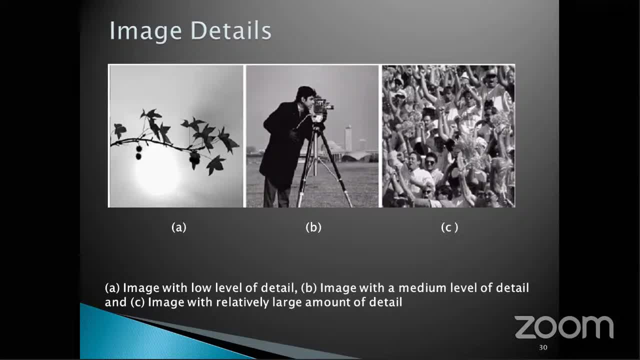 So in this image with the medium level of detail, So man is there, tripod, is there, camera, And in background some buildings and sky, some trees, These all are there. okay, There's more, for example 3,000 feet, But these bubi is tiny, We can just compare it exactly to 1,500 feet. 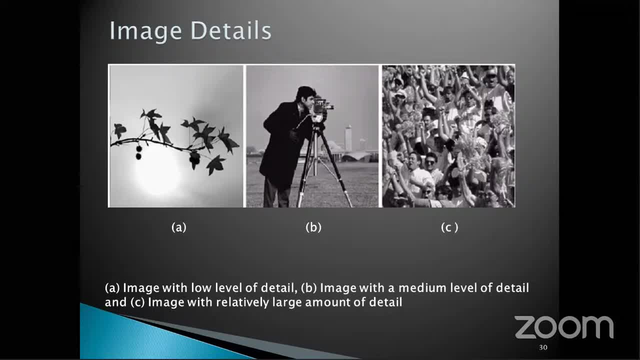 So in the background, as you know earlier, this is. this is not a GRAM, So in three dimensions, tick me. you get these three of detail. see here: more number of detail, large amount of detail. many persons are there, okay. so if you want to see someone's image, okay, particularly some person's image, we need to. 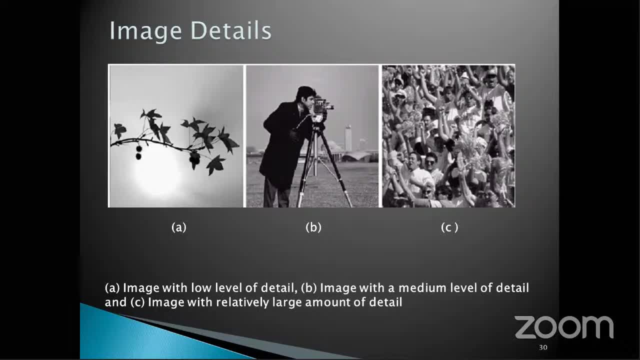 zoom it. okay, we need to identify. okay, so we have to use some features and to identify that person. okay, so many people are there through features means here: uh, his color, his size, uh, is he wearing some spectacles or not? okay, he is having some beard mustache, like that. some features. 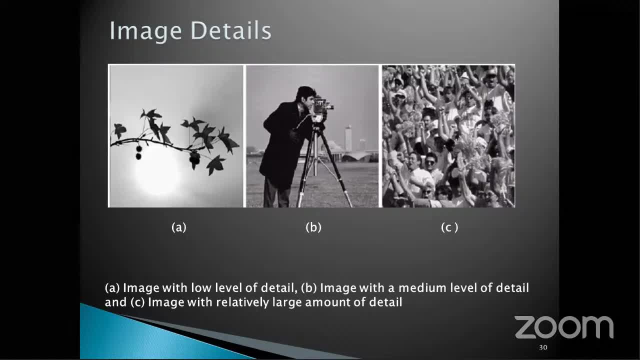 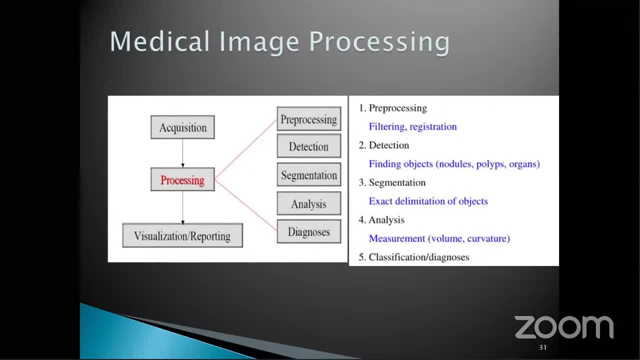 we can recognize some people, okay, so next, so to find some important details. we are going for image processing. in medical image processing also, we have to find out important details in an image. okay, that's why they are going for medical image processing. okay, as it is, we are taking image, okay. 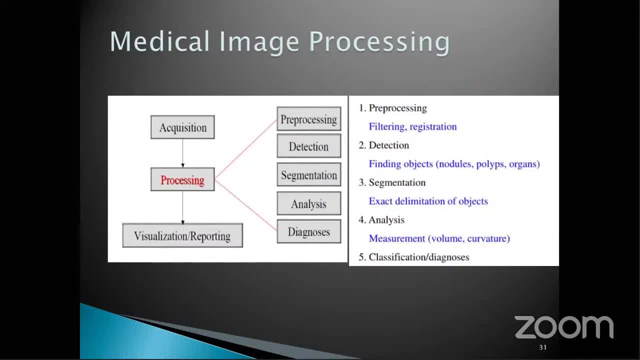 we are not using as it is, we are using some processing techniques. we can find out important details. so here the processing: it has: pre-processing detection, segmentation, analysis, diagnosis: see here. pre-processing means filtration, registration, detection means finding the objects: nodules, polyps, organs, segmentation, extracted diamond: delimitation of objects. 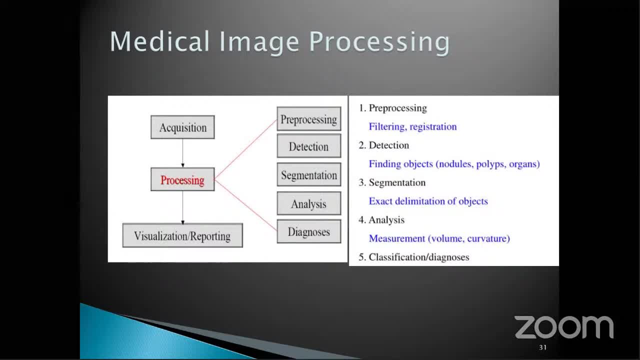 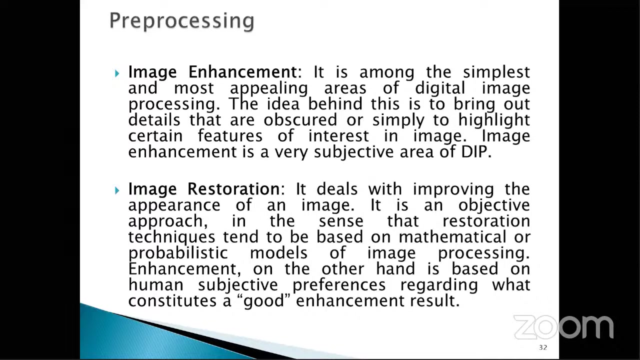 analysis, measurement, volume, curvature, some size of the organ or objects, then classification: okay, it's a normal or abnormal, like that. we have to diagnose something and we have to present. it's a abnormal image. we have to give clear information. next slide, please. so pre-processing- what is one with pre-processing here? image enhancement and 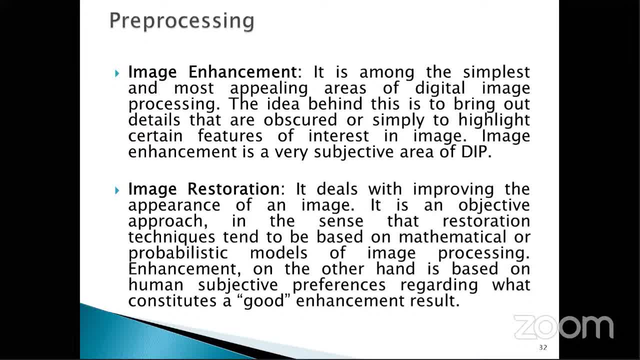 image restoration. two things are there okay in preprocessing: image enhancement and image restoration. image enhancement means local things, already available apps or some other features we can use. you can use that uh features and we can enhance the images. it is among the simplest and most appealing areas of digital image processing. 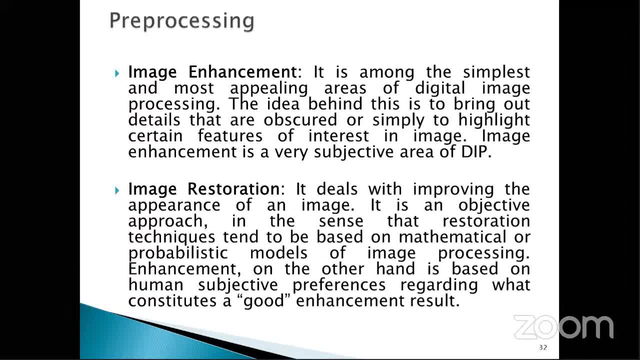 the idea behind this is to bring out details that are obscure or simply to highlight certain features of interest in image. image enhancement is very subjective area of digital image. some of the portion is not clear. we can patch some other pixels on that image. we can like pasting, pasting something on the image. this is enhancement. okay, image restoration means it. 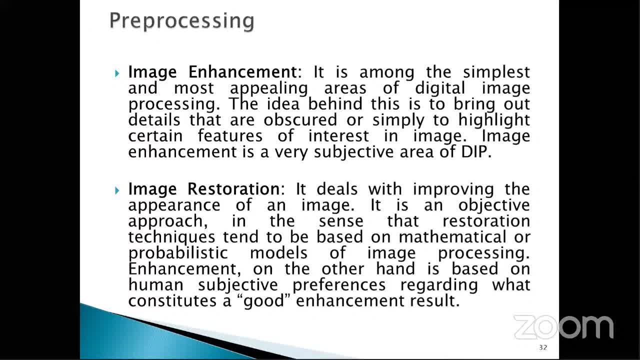 deals with improving the appearance of the image. it is an objective approach. okay, so enhancement. if i am seeing some image, i don't have any idea about that image, just i am seeing some picture scenery. i am telling: this is very nice, nice color, nice birds are flying. 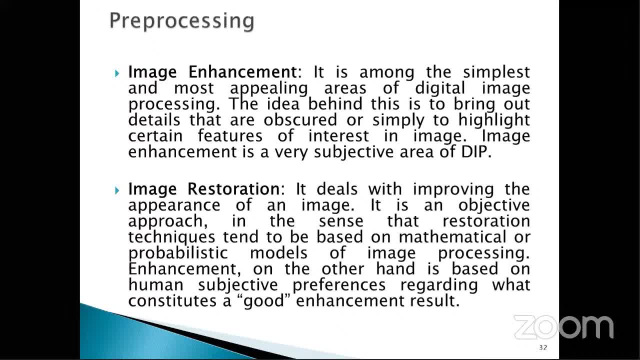 background is very nice, like that, i am saying. but in image restoration fine details will be observed. so for that we are improving the appearance. we are using more algorithms to improve the image. that is called image restoration. in both the places, both the types, we are having some filtration. 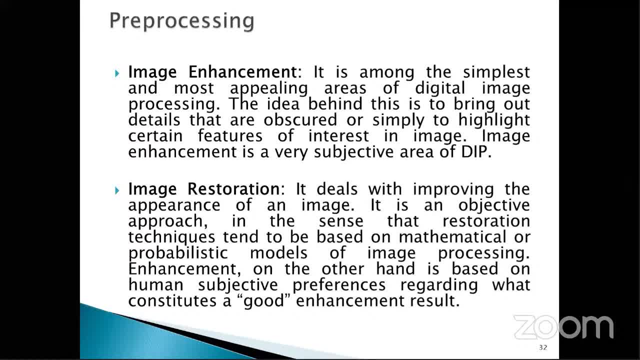 some apps. okay, in the sense that the restoration techniques tend to be based on mathematical or probabilities method of image processing. so we can do some mathematical techniques. manipulations. we can add two images. we can multiply two images. okay. we can multiply some pixels with the total image. we can append some images we can. 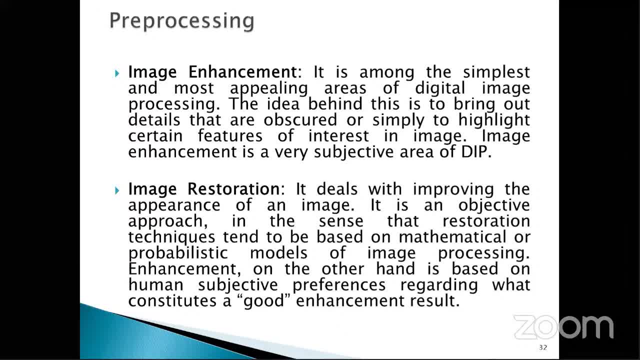 cut out the background. okay, we can clear the background, we can separate the foreground. instead of some other background, we can include some other background like that in image restoration, we are improving the appearance of the image. so enhancement, on the other hand, is based on human subjective. okay, so if the if, 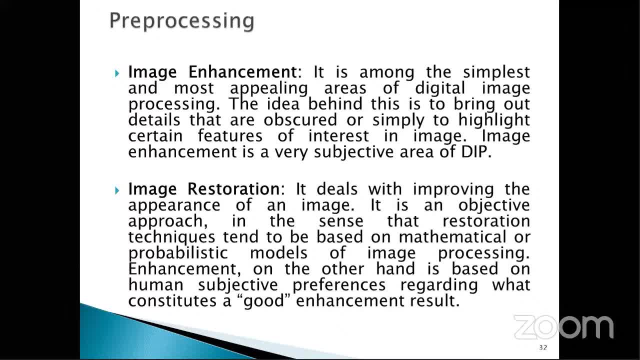 doctor wants to know some details. he will further improve using some image restoration techniques. okay, as a whole, we know this is x-ray. okay, this is showing some uh lung uh in lungs. some uh specific uh things are there. but doctor wants more detail about the image, so he wants to. 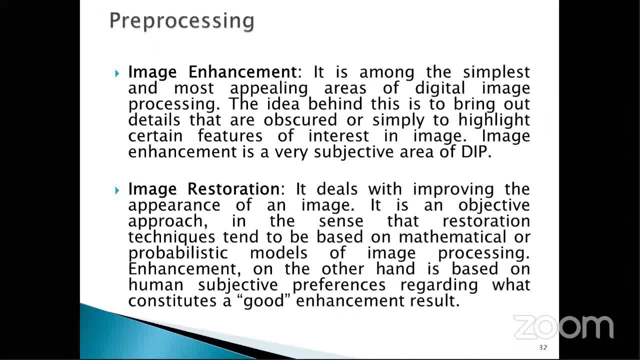 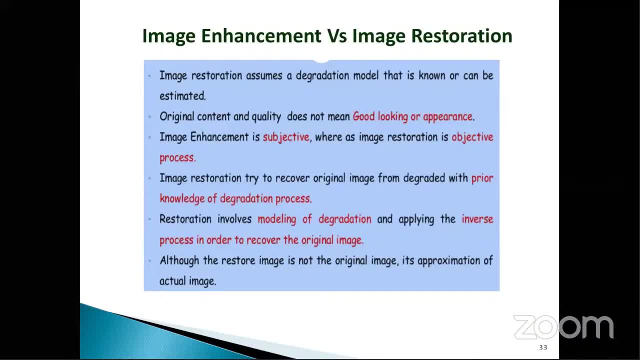 add more image restoration techniques. okay, next slide, please. so image enhancement we we have. uh, we have to get good looking or appearance, okay, so here we can use our knowledge of uh. we have used our knowledge by using some different algorithms and we can find out what are the degradation present in that if you are sending some image from one place to 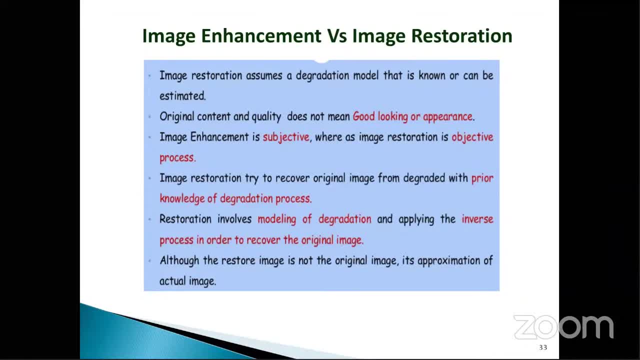 another place. more number of noises will be mixed with, so it will. the image will get degraded so that time we can use degradation process. what are the degradation present in that uh image so that we can restore? okay, through some other uh process. okay, so modeling of degradation, degradation and 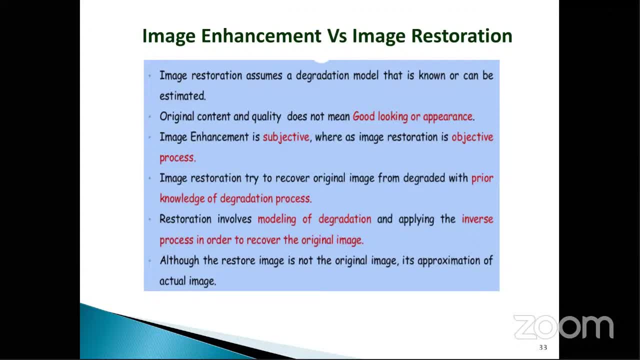 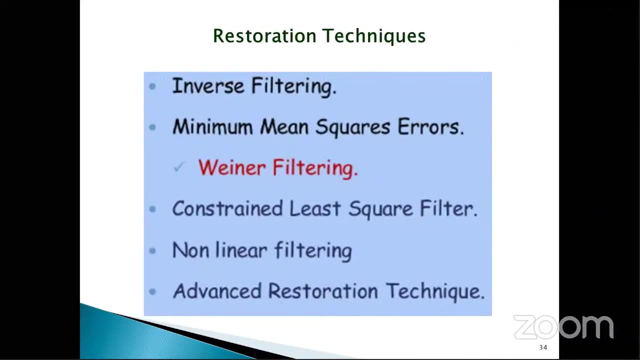 uh, applying the inverse process in order to recover the original image. okay, we are doing this real restoration process. we can recover the original image. okay. next slide restoration techniques: filtering techniques. okay, the example way near: filtering constrained least square filters, non-linear filtering, advanced restoration techniques- was available. next one: 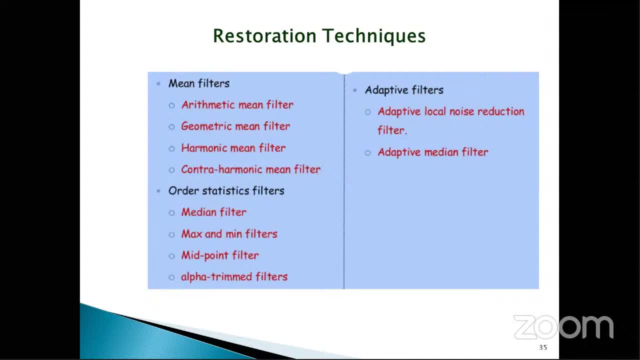 mean filters, median filters, order, static filters, adaptive filters, different filters will be there. we have to use these. what are the filters actually here? these are programs, advanced programs, okay. so if you want to use this filter filter technique, we have to choose here each and every filters and apply on the image. we can get some results. which result is okay for yourself? 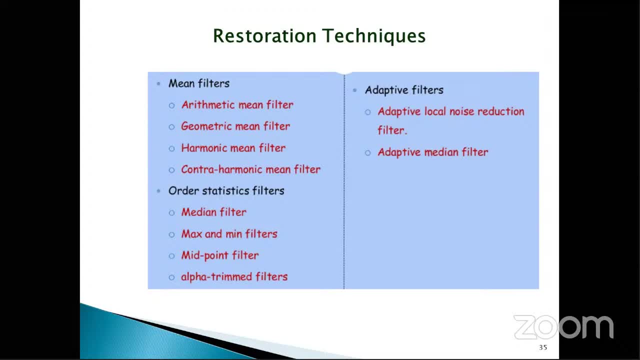 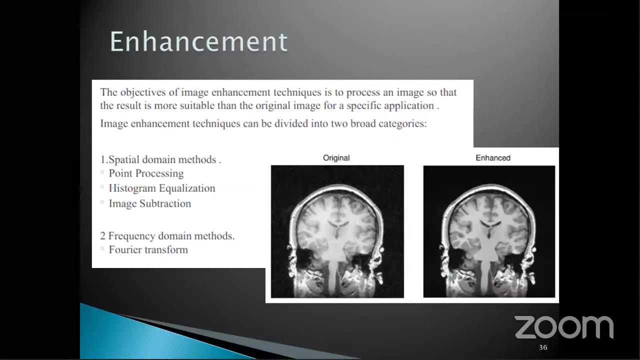 you can use that filter. okay, for good appearance, which filter is easy? which filter is giving good results? we can use that filter. so for that we can use all the filters. on the image enhancement: okay, so enhancement. the objective of image enhancement technique is to process an image. 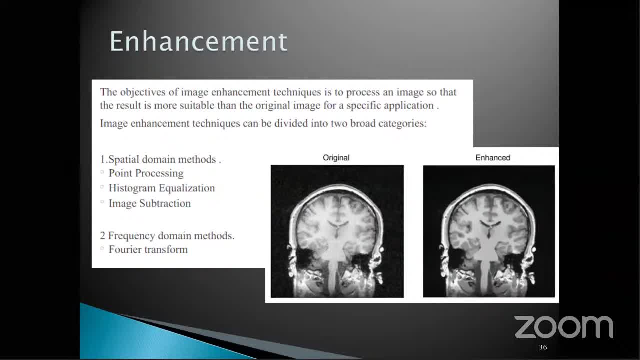 so that the result is more suitable than the original image for a specific application. image enhancement techniques can be divided into two broad categories: spatial domain and frequency domain. so in spatial domain, each pixels will be altered, each pixels will be manipulated. okay, so it is called point processing, histogram equalization, image subtraction. 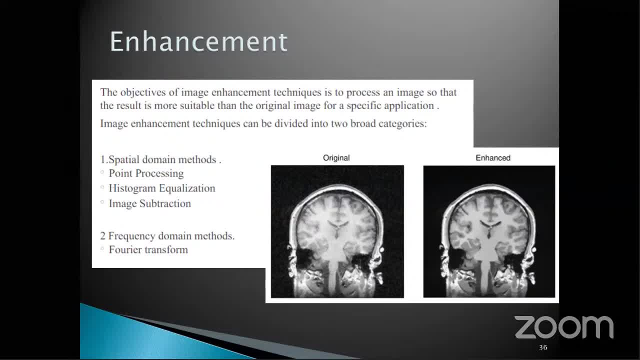 image addition, image multiplication. okay, many manipulations will be there, but all these manipulations are pointing to the particular pixels. okay, so we are doing some process on pixels. it is called a spatial domain method. frequency domain means on the whole. the frequency domain will be carried out on the whole image. the frequency domain methods are used. so, for example, 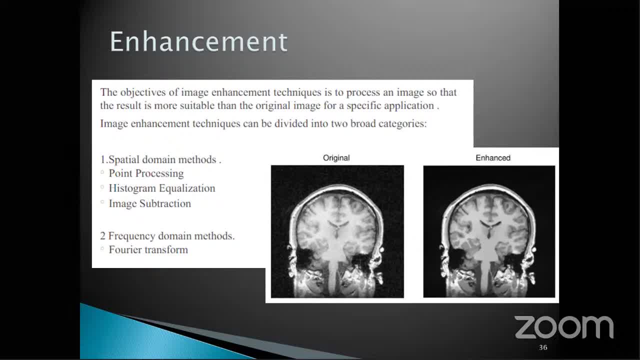 fourier transform. we can use fourier transform to get frequency related image. okay, so from this also we can take more um output good results. okay so fury transform, rigidly transform, replay transform, cosine transform. okay many things. we can use it here. uh see here for enhancement original image. it consists of: 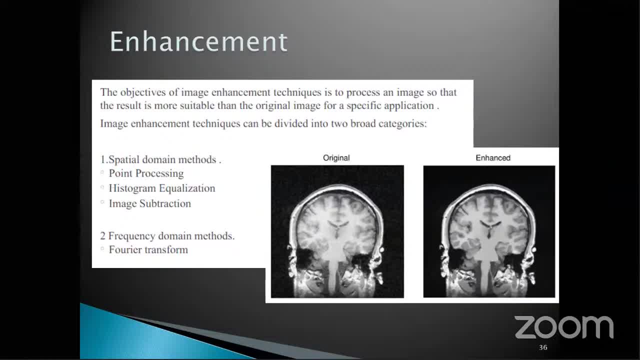 some artifacts. we don't know what is that? artifacts, okay, but we know somewhat. it is not clear. if you use some enhancement techniques, we can get clear image. see here the dull portions will be enhanced. we can get good result here. this gray level will be improved, so we can get this. 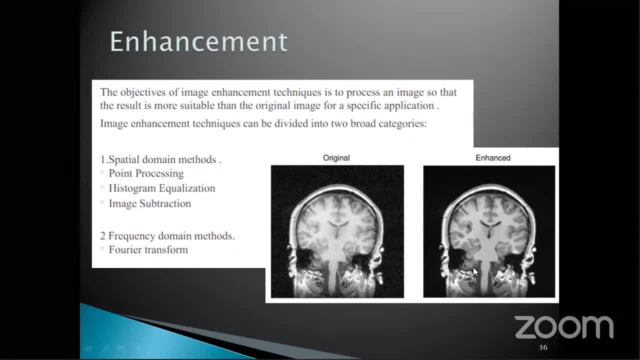 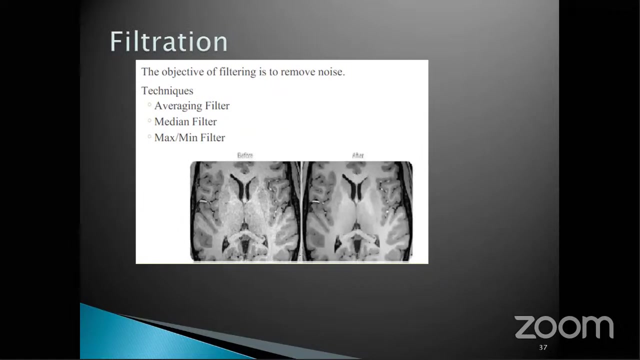 dark image here, dark area here. okay, see here. uh, some portions will be, uh, very lighter, but here it is very bright. in enhanced image all will be very higher bright. okay, so using some enhancement technique we can get a better image. okay. next slide. ma this is. objective of filtering is to remove noise. see here: before filtering, after filtering. so here, 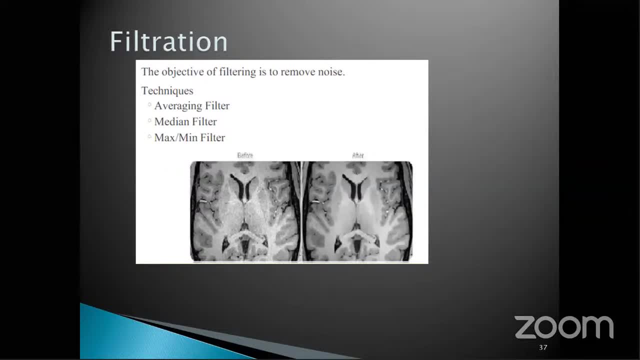 some pepper and salt noise, some dark and light pixels will be there, okay. preference also means white and black dots is present here, okay. so by filtering, after filtering, we can get clear image. see here. so in original image, by using some uh filtering tools, we can get clear image. see here. 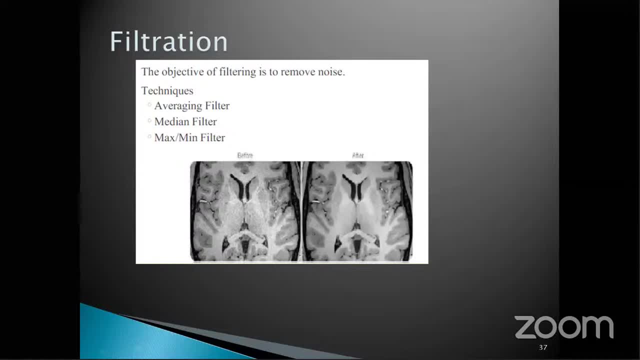 imaging modality. we can get this image after digital image processing. we can get this image after, after filtration. so see this: two filter images. this will be after will be very clear. so, using average filter, median filter, maximum filter, many filters are there. okay, so using these filters we can do uh, pre-processing. next slide, ma'am. 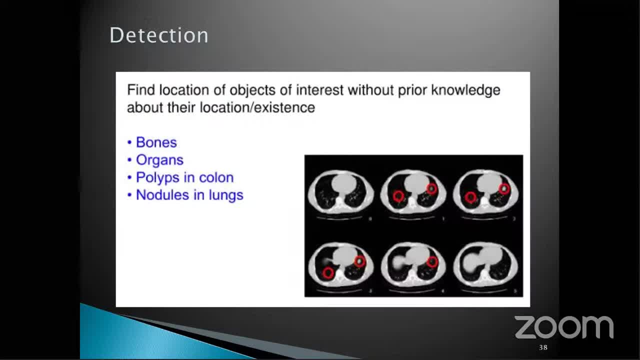 and next reduction. okay, reduction means finding out some abnormalities present in the image. okay, so we uh, for that is engineers, we cannot predict what is this, uh, um, this objects. okay, this is lung image. we know that lung ct image, but inside this some objects are there. we don't know what is that, but doctors can easily identify. 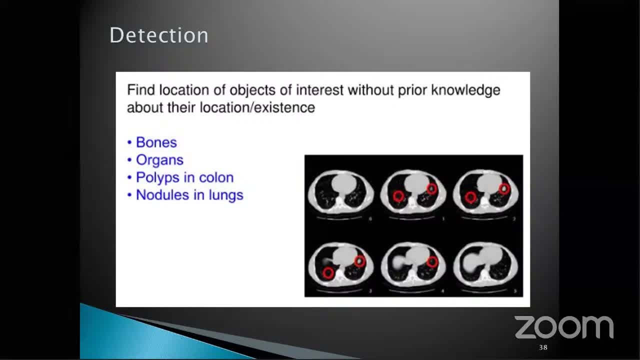 okay, so in this before doctors some engineers can analyze the figure. they can mark the unwanted objects. some objects are there- we don't know what is that, so they can circle the image and they will send to doctor. then doctor will analyze. okay, so before doctor consultation um imaging in imaging modality scan centers. some engineers also will be there. 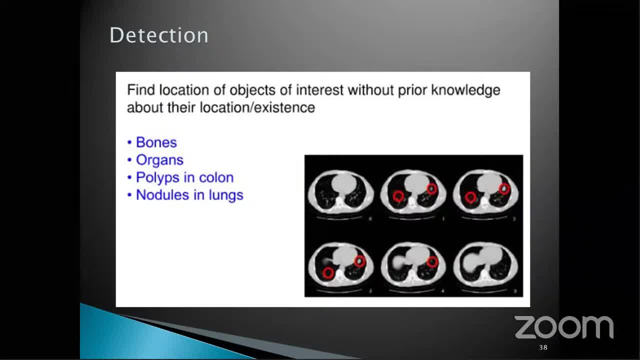 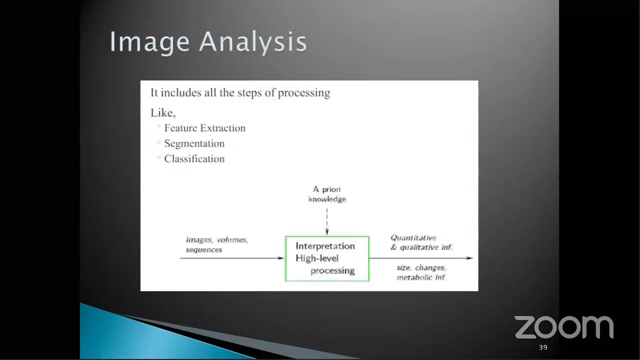 they will predict some abnormalities, blink odontolux transform possible, so this prediction, so finding location of objects of interest without the pre-earth knowledge. okay, so organs, polyps and colon nodules and lungs, this can be observed by other normal clinicians. okay, razed exes は. 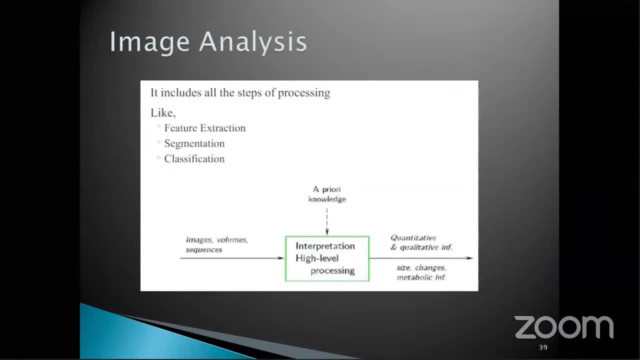 next slide, ma'am. so here it includes all the steps of pre-processing. see here just to reduce location. okay, eleka, feature extraction, that is image analysis. we are step into major analysis. this image analysis includes feature extraction, segmentation, classification. okay, all these steps will be included in image analysis. first, we are going for segmentation. it's a interpretation. 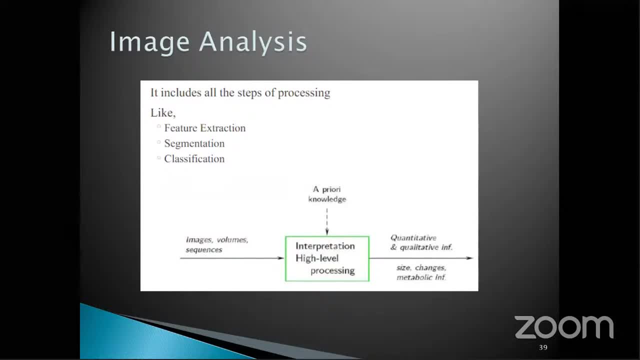 high level processing. okay, so we are segmenting the image. so in an, in an medical image, suppose uterus image- okay, ultrasound or ct uterus image- some tumors will be there. okay, the tumors is segmented. so using some algorithm we can segment the tumor alone. okay, then features are extracted. 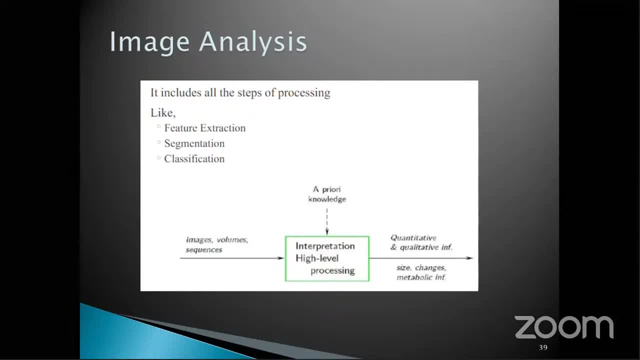 what is the size of the tumor? what is the length of this tumor? depth of the tumor, like that? some features will be extracted from that image and a classification. okay, using some other images, doctor can classify. is it a benign tumor or malignant tumor? okay, see here qualitative and call a quantitative. 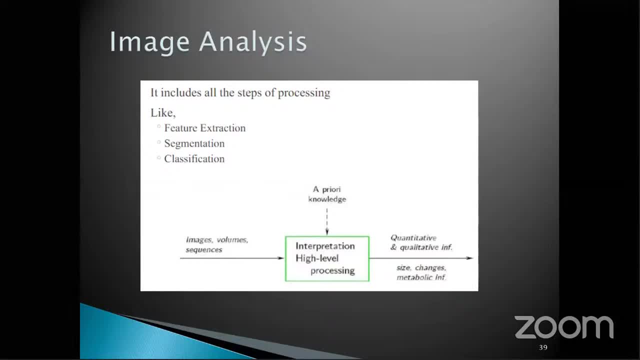 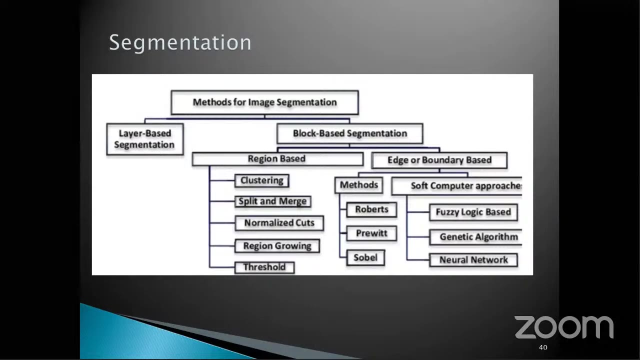 information. from this interpretation we can get qualitative and quantitative information, example: size changes, metabolic informations. okay, next slide. these are all the some segmentation method used in digital image processing: layer based segmentation, blog based step segmentation. some of the types: clustering, split and merge, normalized cuts, region growing threshold. these are all different types of region based. 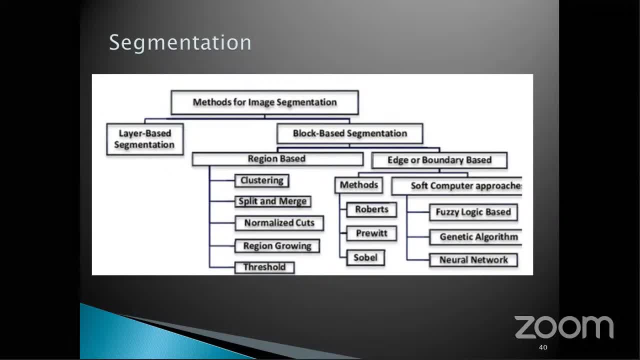 segmentation and edge or boundary based segmentation. okay, these are all edge based method robots. pervils the sober canny. different methods are there and soft computer approaches. okay, here, different algorithms are present when we are doing this analysis. if you are using a large panel or a large cluster of neural networks as a whole, or if you are using a large cluster of neural networks, the 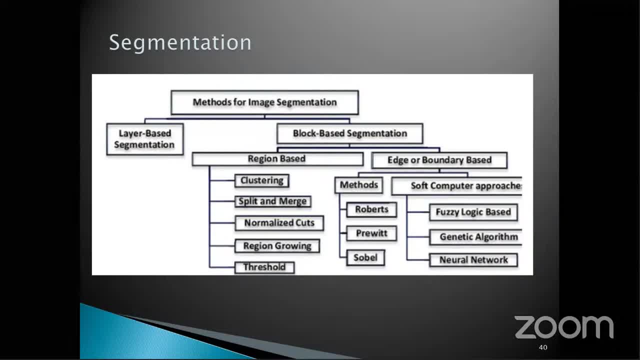 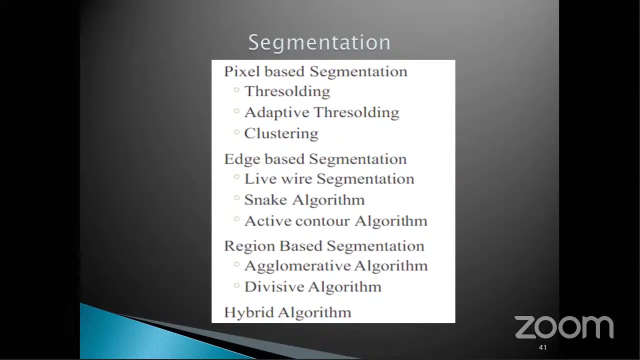 okay, nowadays, many algorithms are there. using those algorithms- fuzzy logic based genetic algorithm, neural network, like that, these algorithms, these softwares- we are using the software. using this we can segment the images. next slide now. so segmentation: pixel based segmentation. okay, so in an ct image, some important pixels are there. 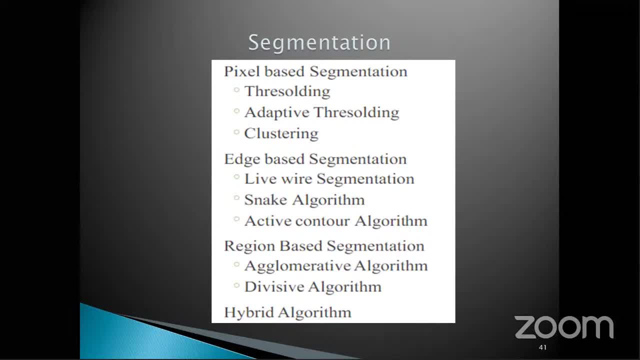 different pixels are there? what are the pixels we have to analyze? okay, so that is threshold basing based adaptive thresholding cluster. these are some pixel based segmentation method. edge based segmentation: okay, snake algorithm, active contour algorithm, liver segmentation. these are all edge based segmentation. it will it will segment the edges of the 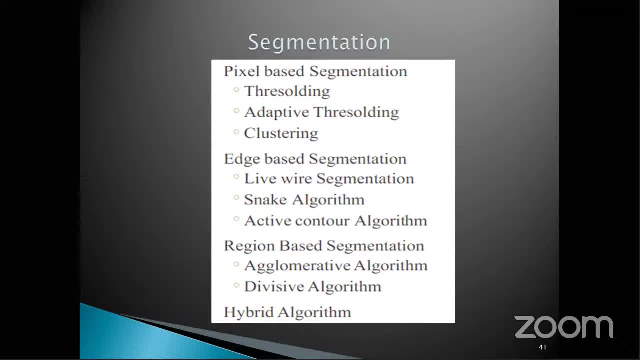 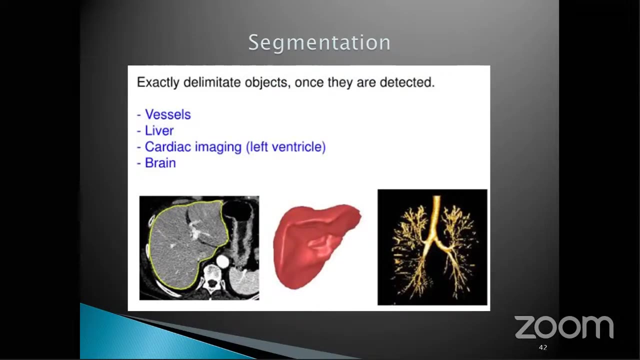 tumor or some other places. okay, region based segmentation. these are all some software, software, software, algorithms. next next slide, please. so segmentation means this is the ct image from that liver image, ct liver. okay, so in this liver liver is segmented. so other areas will be other background, so it will be eliminated. so we this. 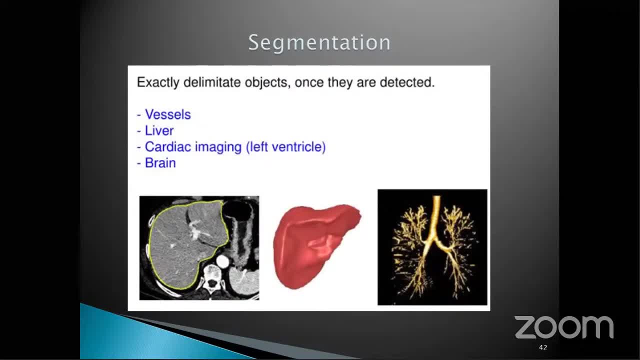 is the region of interest? okay, the area inside this yellow line. okay, so this is active contour method using edge based method. okay, edge detection: the liver edge will be detected using some software, some algorithm. okay, so liver is taken out. okay, that the image. from the whole image, liver alone taken out. 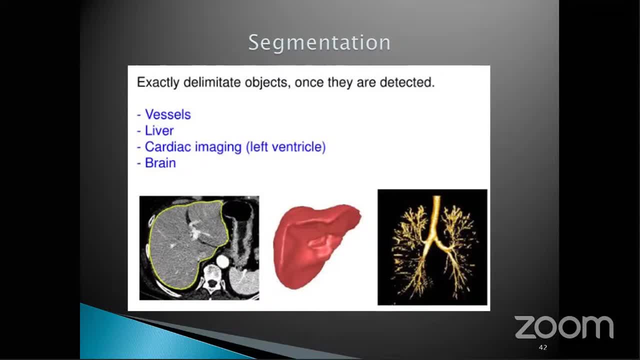 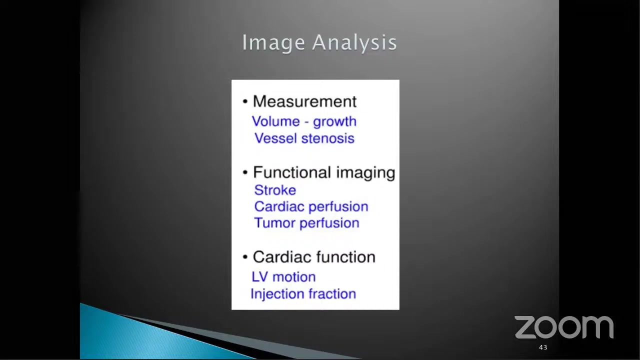 that is called using segmentation. we are analyzing the image. see here some classification is there. okay, classification is there and this is lungs. alright, Emma, image anal, не t is okay. so next image analyst as imas analysis means we know that volume growth the vessel stereo experiences functional. 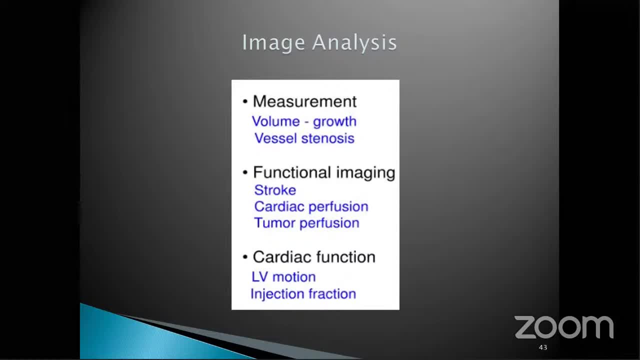 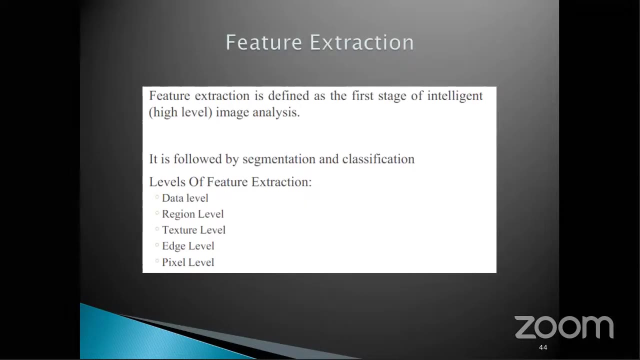 imaging: stroke, cardiac perfusion, tumor per Ih'll, factional cardiac function, healthy motion injection fraction. these are all image analysis using different Spotify modalities, different and always be taken place. okay, the doctors are using different image analysis for from modalities next, next slide. so here a feature extraction. you know, feature extraction means taking some features from the. 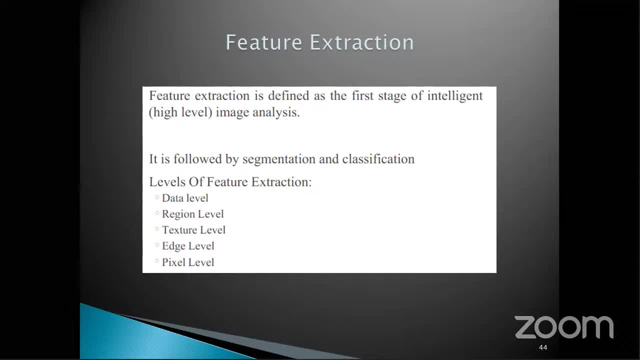 image, size, length, volume, like that. okay, so it is like data level, region level, texture level, edge level, pixel level, so different types of features will be taken. okay, data level extraction: so if you are in a database, more number of images will be stored. okay, example: eye images: using fundus camera, eye images can be, that is, retinal images can be uh imaged, it will. 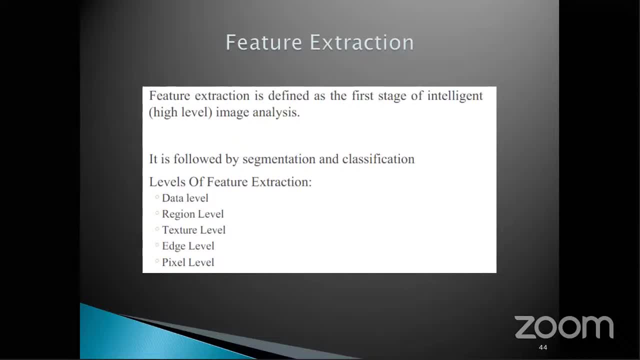 be stored. okay, in an hospital, in a hospital database, all the images will be stored in your database. so, kidney images in kidney images. ct scan is there, ultrasound is there. mra is there for bone x-ray will be there. so different uh data will be present. different modalities, image modalities: okay, so data level. 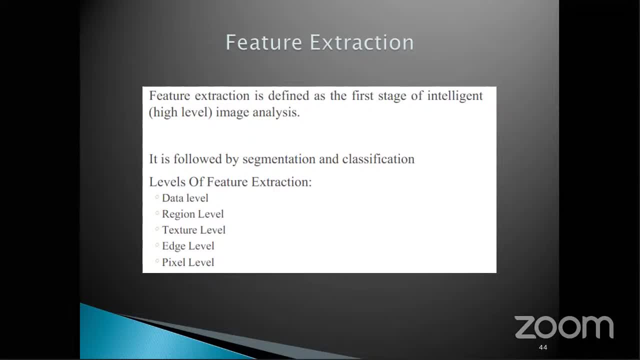 we can take different data level: region level- okay. IneCT scanning- okay, whole body CT scanning. lungs will be separated, okay, from the whole image. lungs will be separated and analyzed. liver will be separated and analyzed like that: the region level and texture level: texture levels, smooth, uh. image in. 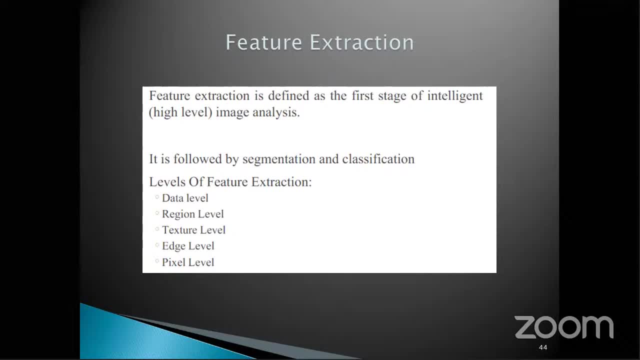 the bones: okay, smooth bones and some, uh, deformated bones: okay, in that bones, pore pores will be analyzed okay, texture will be bone. texture will be analyzed. edgy level: okay. if the size of the lung is shrinked or expanded, okay. if pneumonia, if you, if any patient is having pneumonia, means 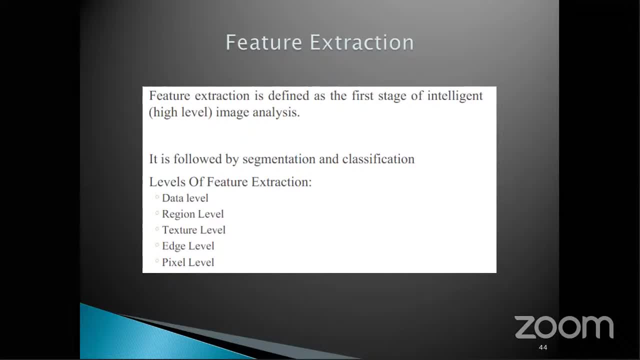 he might be having uh expansion of lungs or deformation of lungs, shrinking of lungs- both he can. um, he can be coming through so that we can using using texture analysis or edgy level, we can find out that- and pixel level also. okay, this also used for uh deduction. next slide, please. 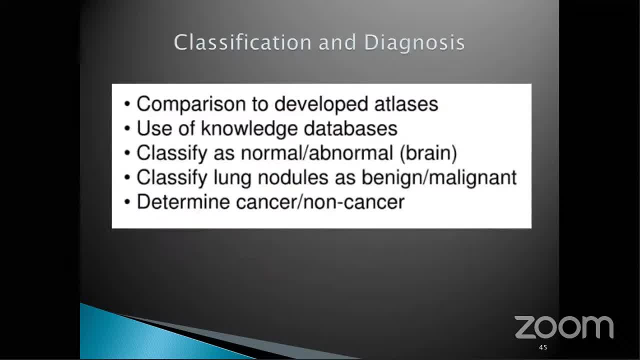 classification and diagnosis, then comparison to uh developed atlas, use of knowledge database, classify a normal, abnormal brain. so classification means we are taking some image. whether it is normal or abnormal we have to find. okay, that is the classification of uh image, with using some features taken from the segmented. 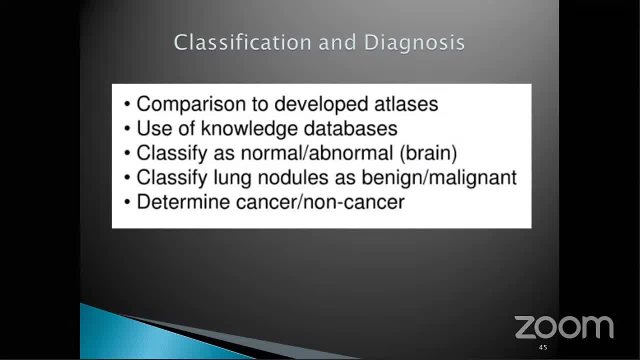 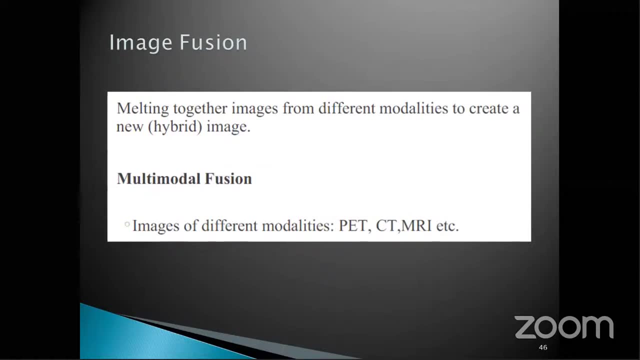 image it's a cancer or non-cancerous and the classical lung nodules are benign or malignant. like that we are classifying the image. next slide, please. the next slide please. image fusion, suppose ct images not enough for my observation. i can combine with PET positron emission topography, so i can combine these two. i can get good image, good information. 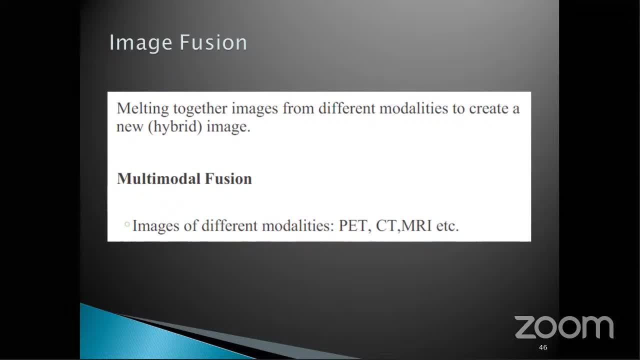 i can get. suppose mri is not enough for my observation, i can come back, combine mri with the pet. okay, these two will be combined. i can get a combination of these two. okay, if there is a good, more clear image. okay, that is called multimodal fusion here. this is one different type of 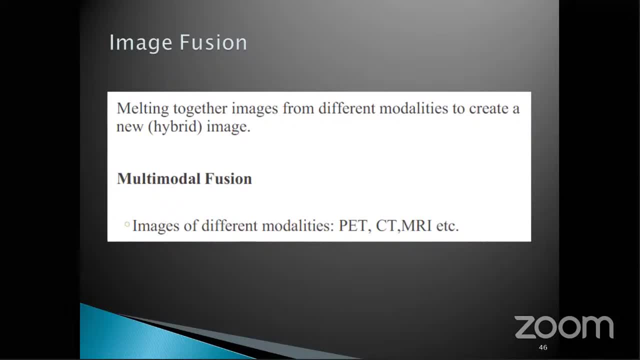 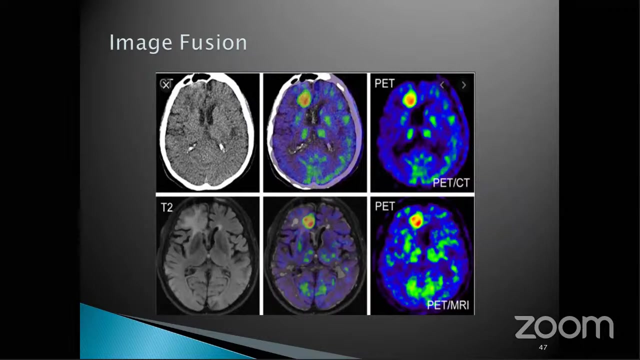 modality ct is an different modality, mri also like that, but combining these two. it is called as modal multimodal fusion. okay, it is called hybrid image. two images will be combined, so it is called a hybrid image. next one: see here, this is ordinary ct, this is pet. okay, here combined. 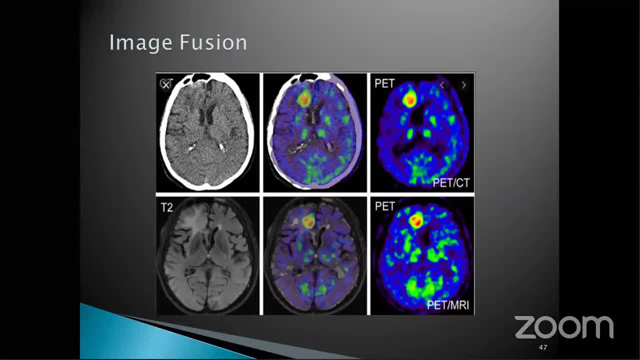 these two ct, with the combined, with the pet, it is called pet ct. okay, so from this we observe some area. this area, okay, highlighted area, okay, this will be very clear. okay, so it is the area of the hybrid image. next one: see here, this is ordinary ct, this is pet. okay, here combined. 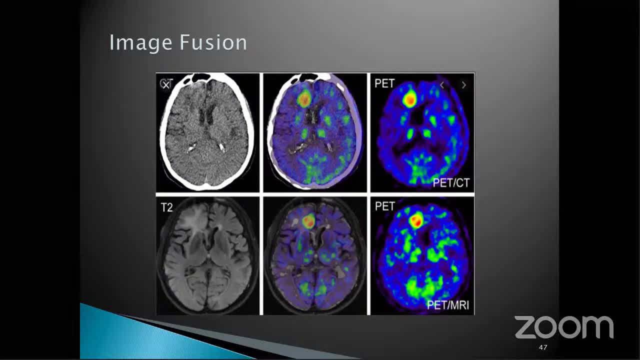 actual abnormality will be diagnosed easily by doctor. okay, actual abnormalities can be um diagnosed. and here it is mri. okay, so it is having some area. but see here, pet ct. same image. pet ct is showing some abnormality here. okay, so combining these two image, we can get more. 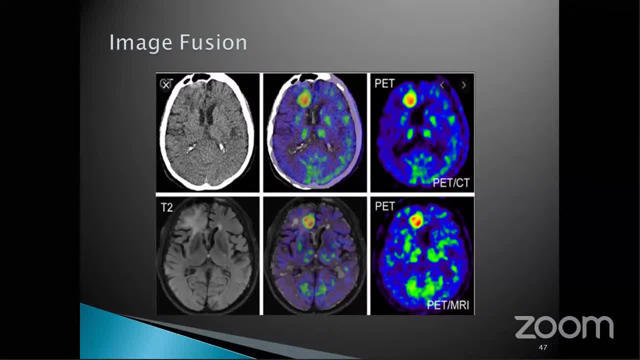 more the normalizability of the information. okay. so if we take the normalizability of the normalizability of the image, we can get more normalizability of the image. we can get more clear image here. okay. so here also some portions. are there some abnormalities? it is not clear. 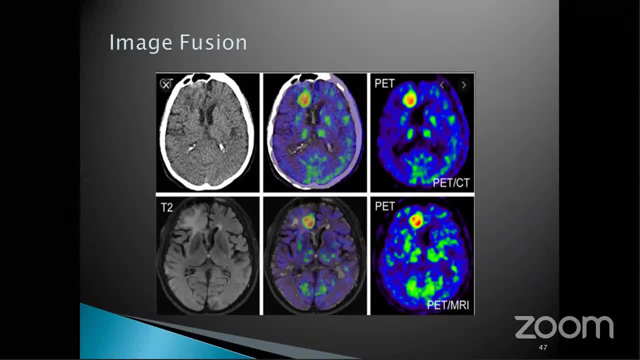 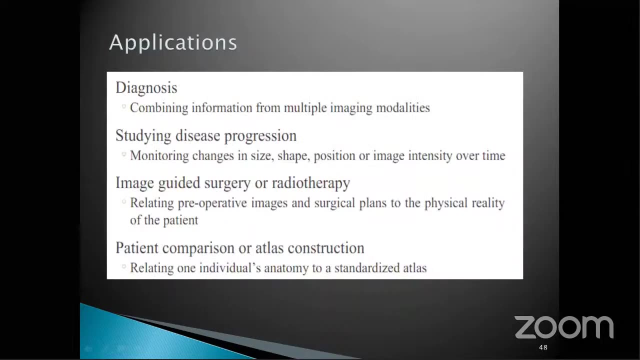 size also reduced. but you see here the size, actual size will be shown. so combining these two modalities. okay, ct with the pet pet mri. sorry, pet ct here. pet with the mri pet mri. okay, next slide. so applications using digital image processing. the applications of medical image processing: 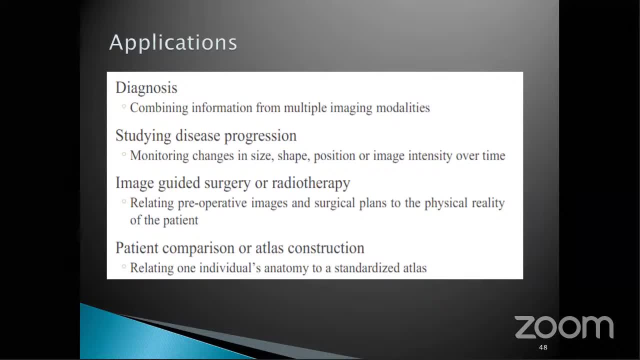 okay, diagnosis combining information from multiple imaging modalities. studying business progression: okay, monitoring changes in size, shape, position or image intensity over time. image guided surgery or radiotherapy: okay, image guided surgery. so nowadays many operations are conducted, surgeries are conducted using guided image. guided image means by seeing the image they're taking, they are doing some surgery. okay, eye images, liver images. 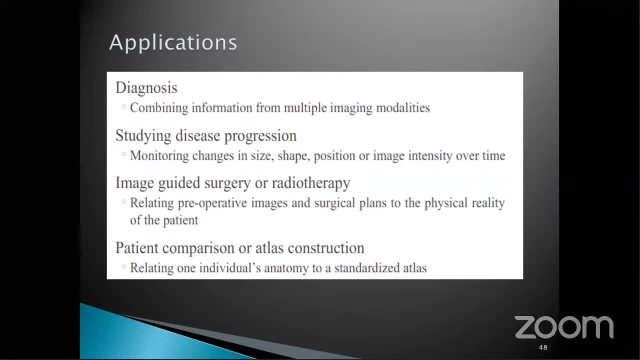 heart. heart surgeries will be then using this image: guided surgery. okay, radiotherapy, radiotherapy. for cancer patients, radiotherapy will be given. so we have to give the point. application of radio, radio, radiotherapy: okay, so that isotope waves and our radiations, nuclear radiation, will be given to that area. 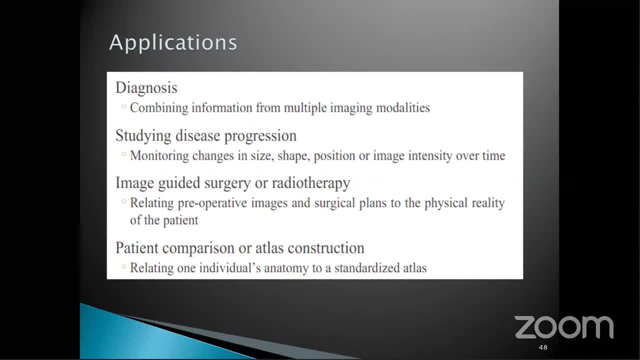 particular area we should not give to the near nearby cells then that it will also get affected. so pointed area we have to give the radiotherapy for that. they will use image guided radiotherapy. so radio relating pre-operative images and surgical plans to be to the body physically, uh, reality of the patient, patient comparison or atlas construction. so 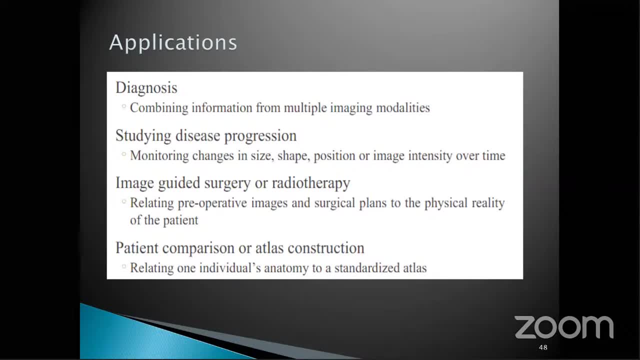 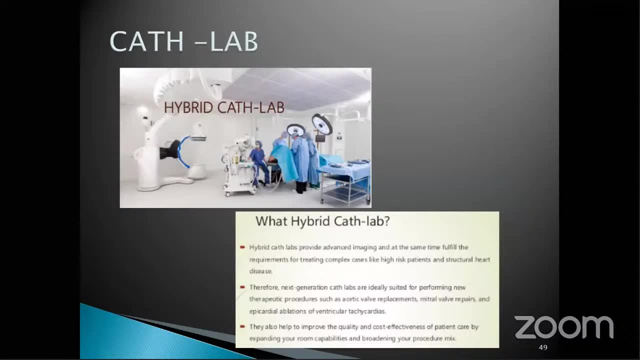 relating one individual's anatomy to a standardized atlas. okay, next slide, please. so this is the cath lab, so cat lab means catheter lab. okay, so nowadays, uh, angiograms and uh, some stents will be, uh, you will be fixed in our heart. so some of our laparotomy. 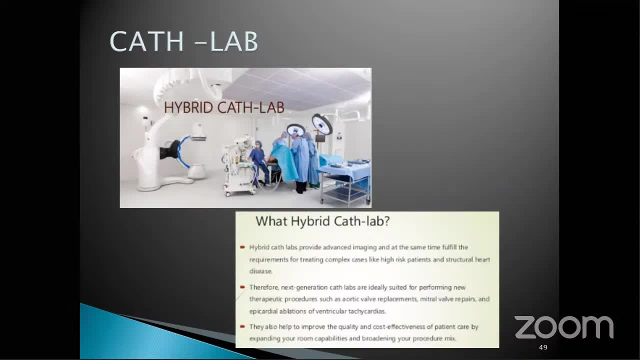 work on it. so and in which stage we will provide. 웠 Sk solved our laboratory cancer. now, the end of 2018, and we are already okay- heart valves, heart vessels stand- will be given provided okay. so for this type of such surgeries, they are using catheters. so the catheters is having some camera and balloons and 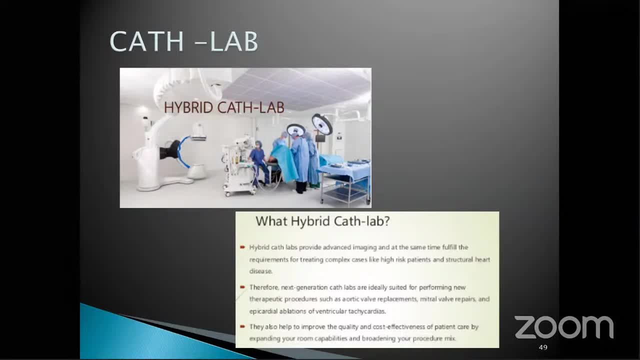 for cleaning- suppose it is some tumor- means they have to cut the tumor and they will excrete the waste, okay, through some uh pipes. so the catheter is having the tube tube structure, uh in front of the catheter camera will be provided and through optical surgery they will cut the cut the 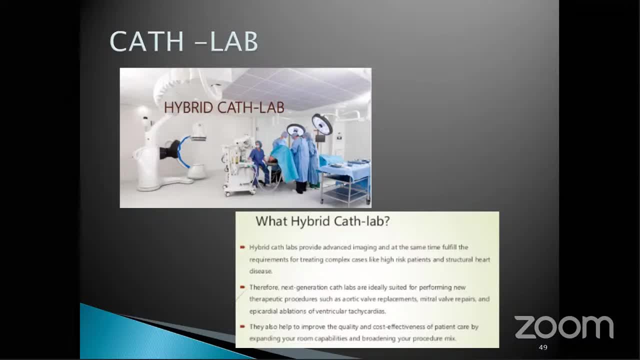 tumors. they will clean that portion, okay, so it is called catheter lab, cath lab. it is hybrid cath lab here. imaging modality also there for guidance for the surgery using image modality and they will do surgery. okay, see, this person is guiding the uh, doctors. okay, so guiding the doctors and doctors also. 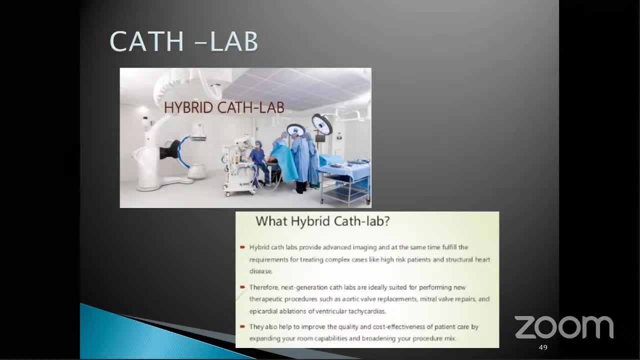 side by side. they will see the structure. okay, they are inserting catheters through some veins, through the heart. they will place the catheter in the valve or vessels and they will do some surgery. they will remove plagues in that vessels. they will put some splendid okay. so this is the example for a hybrid catheter lab where 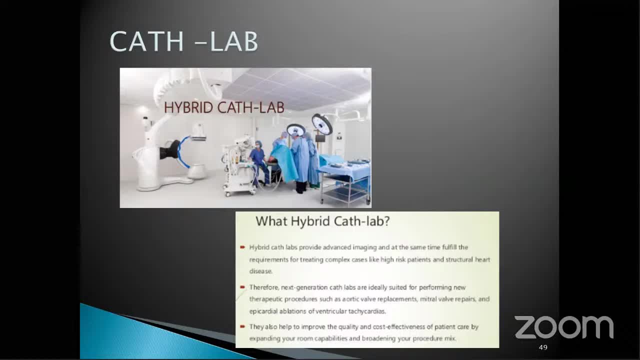 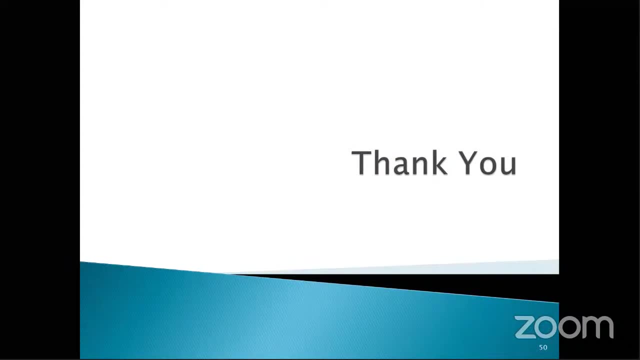 the imaging is very, very important. okay, next, next slide. thank you, students. that's all about the medical imaging and application. so i have touched a very important in this. if you have any doubts, please ask me this query session. thank you so much, madam, for your valuable presentation. in fact, we have touched all. 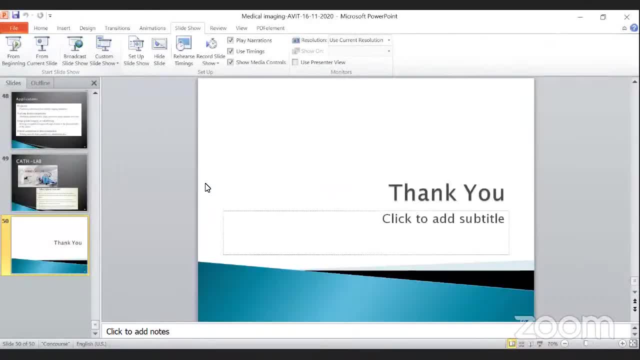 the basics and inner notes of image processing techniques and as well as medical image processing also. i hope this is a doubt clearing session, as you rightly said. so, students, if you have any queries, please raise your hand. i can allow you to talk, or you can put your questions in chat. 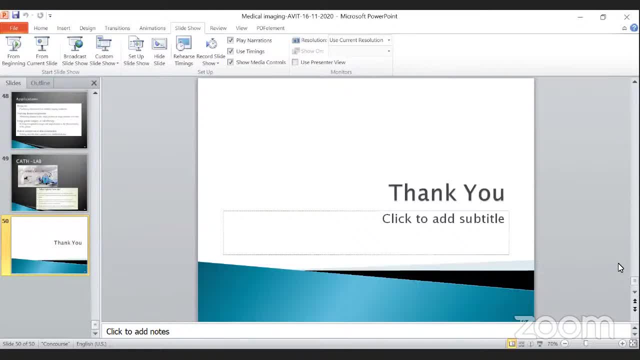 box, we'll have a discussion. hey students, if you have any questions, please put up in chat box or please raise your hand. i'll allow you to talk. ma'am. i have a question, ma'am, can you just actually this is a very basic one, but i just want to know in in. detail about what is the difference between mri scan and ct scan, so which one is most preferred? while taking an uh imaging of and critical sections: in critical sections, ct is best because ct in all 365 degrees it will take image. okay, it will clearly give the volume of the abnormality. 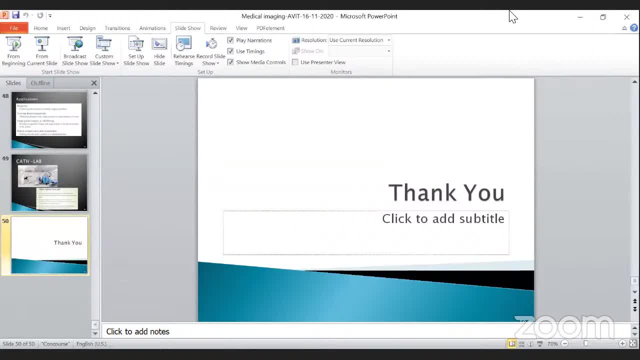 okay, suppose tumor is there, means it will give clear picture about the volume of the abnormality. mri also okay, no problem. but ct. comparing to mri, ct will be best, but ct radiation is there. it is combination of x-ray in all the directions, so radiation will be more, but mri radiation is not there. but comparing to mri. 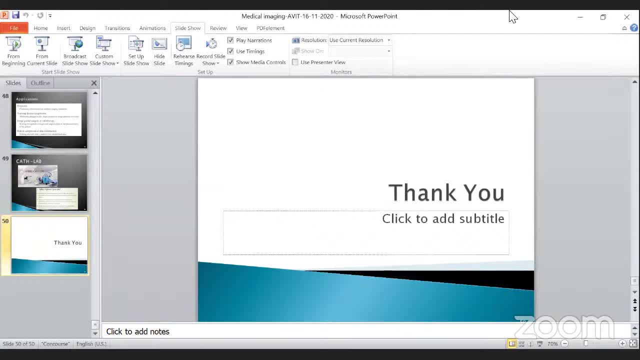 ct will be giving good clarity about the image. okay, suppose if, if an organ, like if you take a brain, if that has to be sampled into number of slices, so in that case mri holds good, or ctm mri is in that case, uh, brain, brain in the. in that case mri is best, sir. 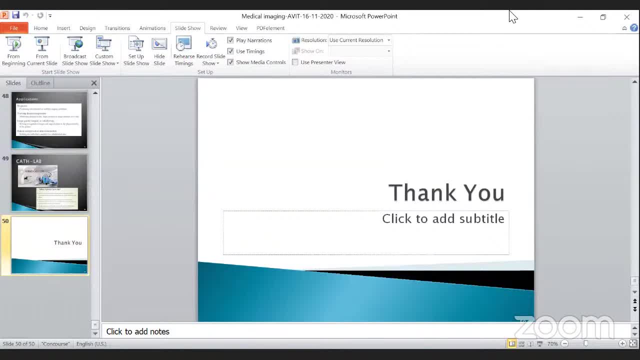 for brain structure, mri is best, okay. okay, then we have another question also. yes, uh, which is the best filter for noise removal for satellites? which is the best filter for noise removal for satellites? imaging man? any idea on that? adaptive filters are very actually good for a satellite images, because satellite images 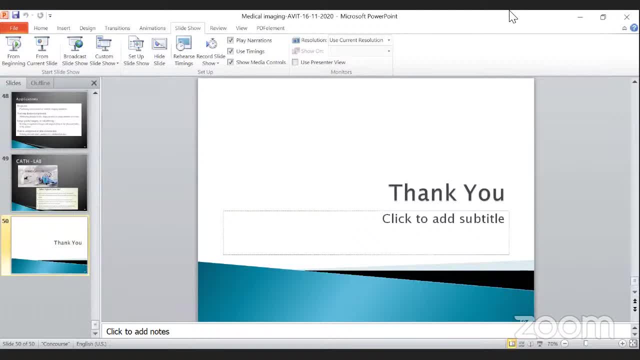 the height will be more, altitude is more and also it is using climatic condition also. it depends upon the climatic conditions also. so in that bad situation it will use adaptive filters. okay, okay, okay, thank you. thank you for your answers. is there any other questions from the participant side? 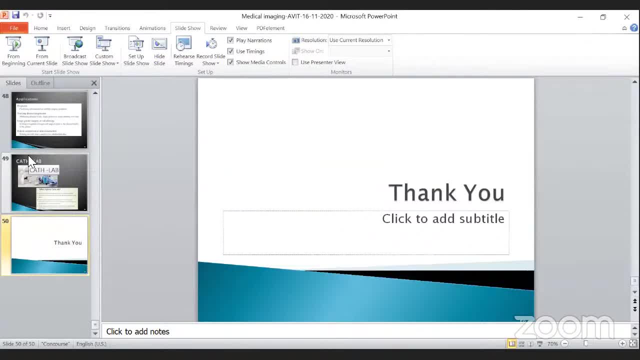 okay, sir, thank you. ah yeah, yes, ma'am, thank you, and i have this. i have one last question them: uh like uh. is there any advanced uh image enhancement algorithm? is there any currently available uh algorithms? so nowadays, many optimization techniques will be followed, sir. optimization techniques for uh image segmentation, image analysis: optimistic in everywhere. 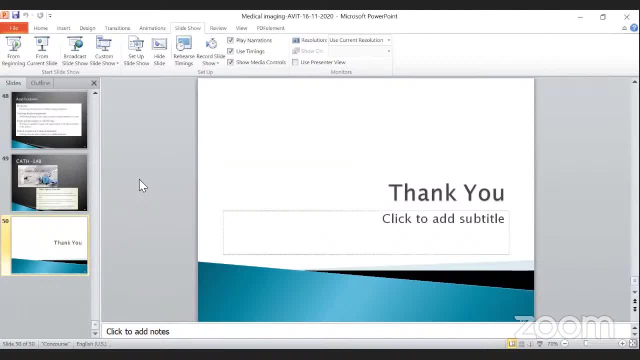 optimization techniques are used, sir. so in that electromagnetic optimization and algorithm, uh, swan spam optimization- so many things are there, so we can go for deep learning like that we can go for. so many things are there, so we can go for deep learning. like that we can go for. 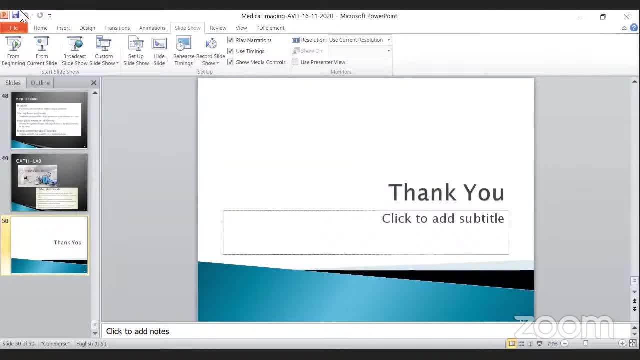 okay, okay, okay, ma'am, thank you. thank you so much for your answers. uh, ma'am, sanjay ma'am, i think we can formally wind up. uh, yes, sir. so, ma'am, ma'am, i need. i have one last question. yeah, yeah, please. uh, because, uh, like in classification, because we have been using a lot of classifiers for output. 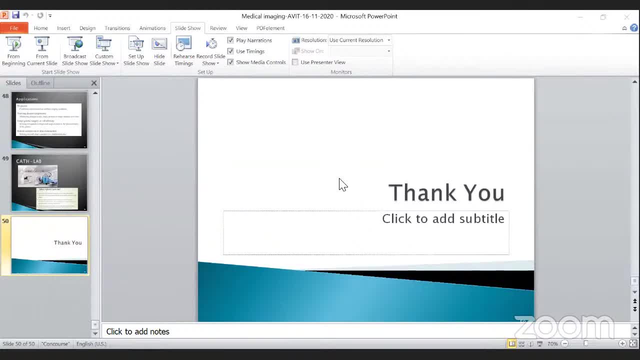 uh for differentiating normal versus abnormal cases. so because i have just uh used um to my project was spm, which is a support vector machine and in which techniques we can use the support vector machine and in which techniques we can use the support vector machine and in which techniques. 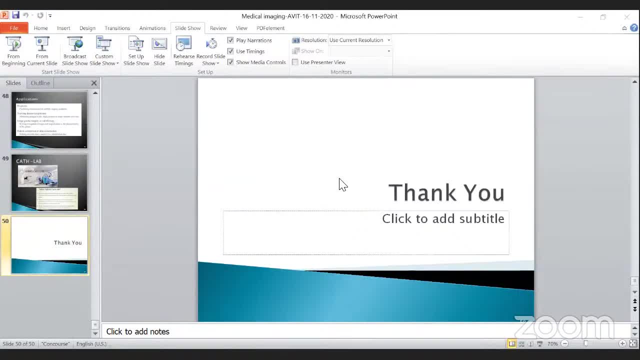 uh, we can uh improve our accuracy levels. uh, whether we're just going for spm or we have a lot of classmates right- rbf and spms and kms. so, likewise, in which technique we can uh use, uh, we can improve the accuracy map that is depends upon your input and segmentation, or which means like: 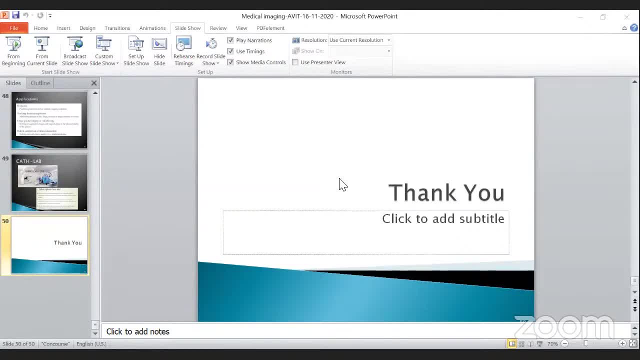 sort of things. i'm asking on which technique can improve the accuracy level in spm? also we can. it will give good results. but all uh algorithms need more number of features. now how many features you are using it will give good results. now, good classification, so taking the features also very, very important classifications. 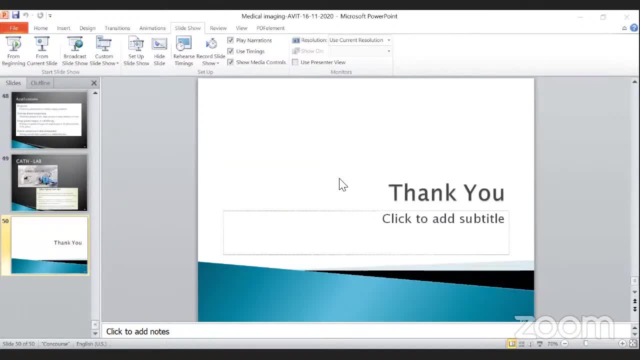 so feature classification is you have to select the different feature detection techniques are there now. so features we have to take. it depends upon features. okay, thank you. okay. any other questions ma'am from participants side one question uh is being asked by linkadarani. so matlab will be effective tool for 3d modeling for medical images? this is what the question is. 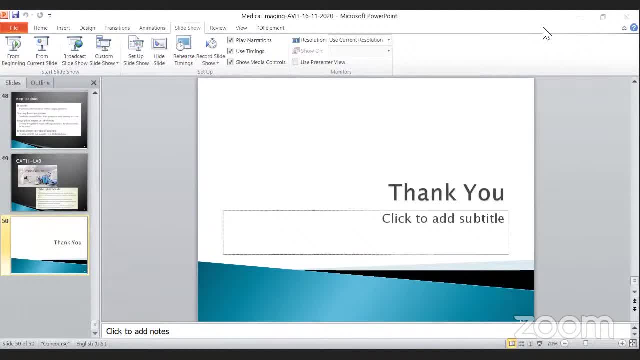 matlab will be an effective tool for 3d modeling for medical images, 3d modeling. actually, i'm not well in that 3d modeling, sir. matlab is very good for, uh, image processing for 3d modeling. i don't know that that area because i didn't do for 3d modeling. okay, okay, no problem. 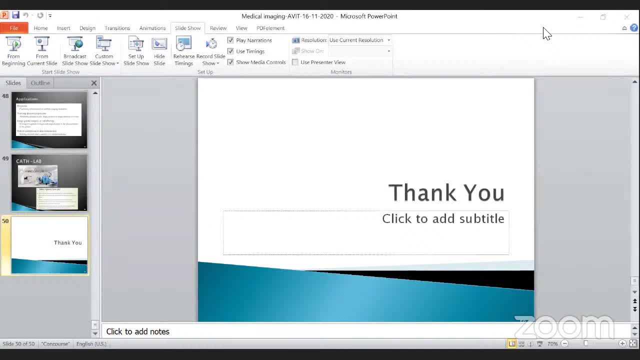 so is there any other questions? so nowadays we are using octave also, sir active, instead of using matlab lab. it's a free software. no, sir, okay, we are conducting labs through octave for signal processing, image processing, everything. so octave also. in this pandemic situation we can use octave also. 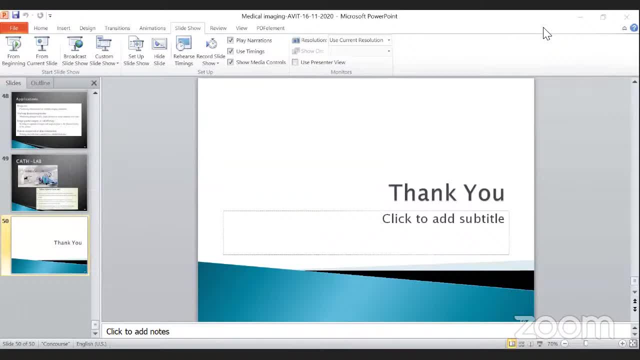 yes, ma'am. if there is no other questions, you can formally wind up ma'am. uh, yes, sir, yes, we can go. yeah, uh, ma'am, am i audible? ma'am, yes, uh, can i wind it up, ma'am? yes, ma'am. yes, ma'am, we can wind up ma'am. thank you, okay, as an end. 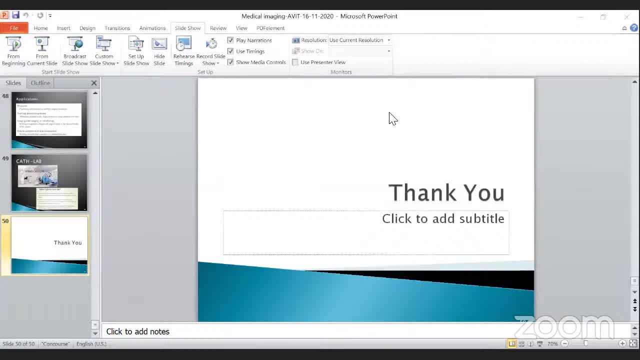 comment. i would like to sincerely thank our management for permitting us to conduct this guest lecture, and i would like to thank our today's speaker, dr jay shivagam sundari ma'am, for sharing his insights and his experiences with us, and we hope to see you again next year. 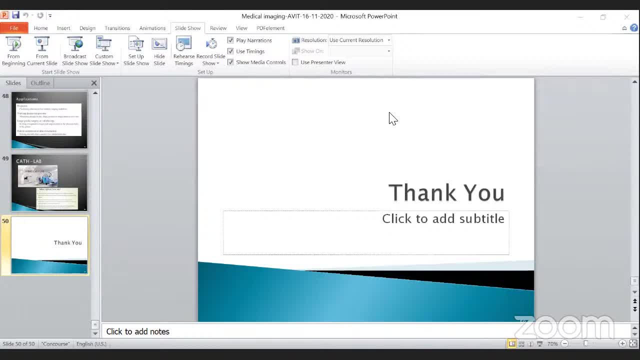 her valuable insights about medical imaging techniques and its biomedical applications. i would like to thank our head story sir for his graceful support extended towards this webinar session, and also our fellow faculty members for this wonderful coordination. and, finally, i would wholeheartedly thank all the participants from different locations and for making your presence. 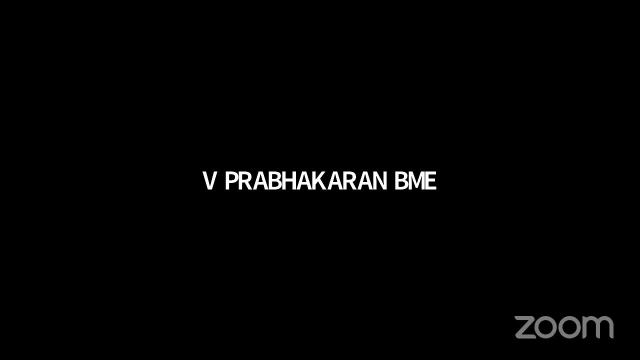 to make this webinar a grand success. thank you all. thank you, ma'am. thank you so much for your presence. yes, well, end of the meeting. uh, sandhya, ma'am, are you there? yes, sir, uh, uh, ma'am, just check the link. actually it is not opening, it seems. uh, yes, and now i have just 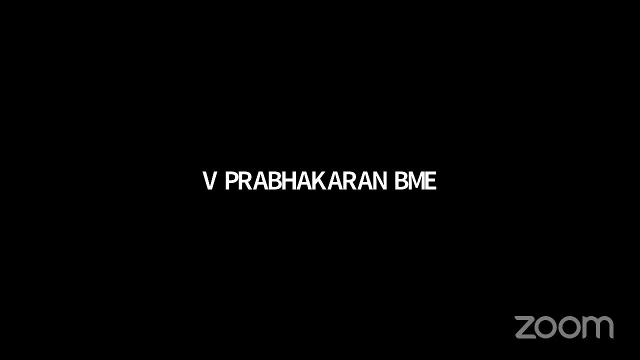 modified. yeah, yeah, please put it in chat box now, so that others can uh take up the feedback. now i think we can stop the live streaming. also, if link is ready, you can put it in chat box. ma'am. yes, sir, participants, just a few minutes. uh, the link will be corrected and checked. 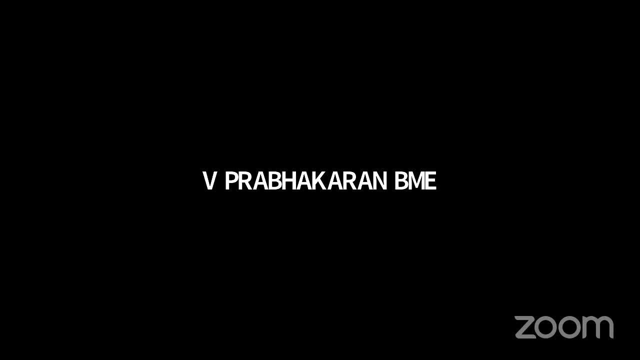